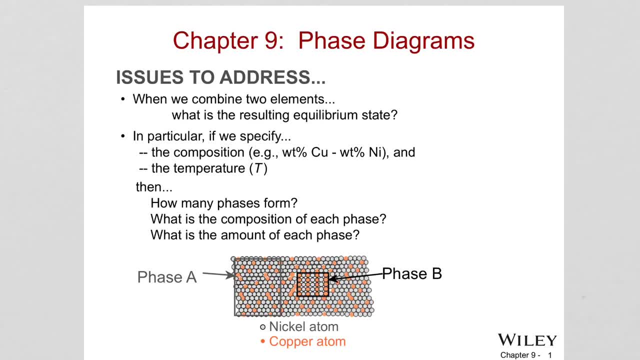 So today we're gonna learn about phase diagrams, and phase diagrams are very important because when we combine two elements, we need to look at phase diagrams to see what is the resulting phase or what is the equilibrium state. So phase diagrams are generated based on thermodynamical 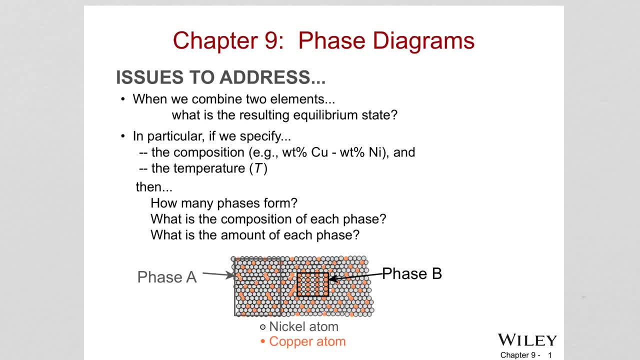 equilibrium, meaning within a long period of time, two elements are mixed and observe what type of phases they are making at a certain composition of mixture and at what temperature. So phase diagrams, therefore, is going to tell us what is the phase of a system at a certain composition and at a certain temperature, So how many phases form. So it doesn't. 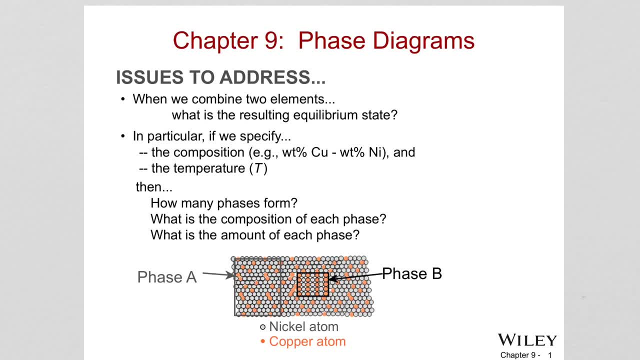 have to be just one phase. it can be more than one. And what is the composition of each phase? How much of? let's say, in the image we are seeing, copper and nickel is mixed and we are seeing they are in different phases. So these are thermodynamically equilibrium phases. So phase A and phase B. 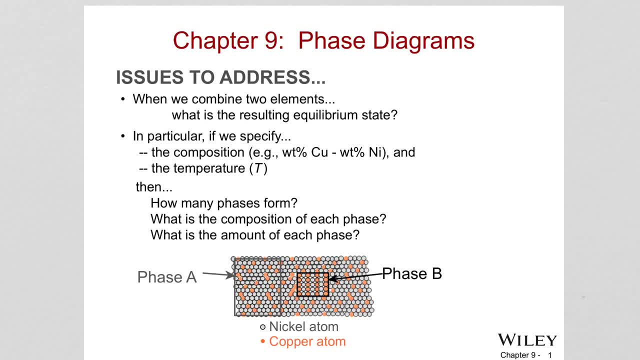 two of them have different structures, different properties, And what is the composition of each phase, Meaning what the amount of nickel or copper in phase B, or what is the amount of copper and nickel in phase A? or how much of carbon is mixed In the dimension of three or many, some with the performs of each phase. So in that particular particular application we are perhaps going to start with threehing, if we keep the parameters right, and then we will eventually start with four- depend on whichever components that are shown in the diagram Basis. consumer side. 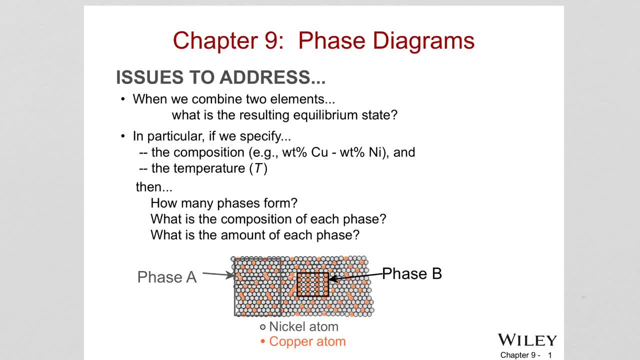 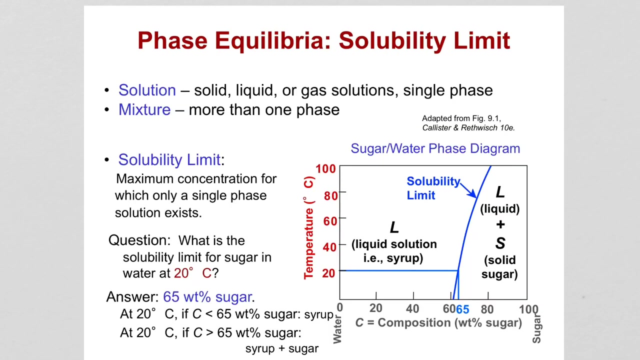 the overall alloy, the phase A is or phase B is. What is the percentage of the phase B? So amount of each phase? So we're going to understand phase diagrams and we're going to read information from the diagrams. Let's learn about solubility limit. So when we say, let's look at some terms, Solution. 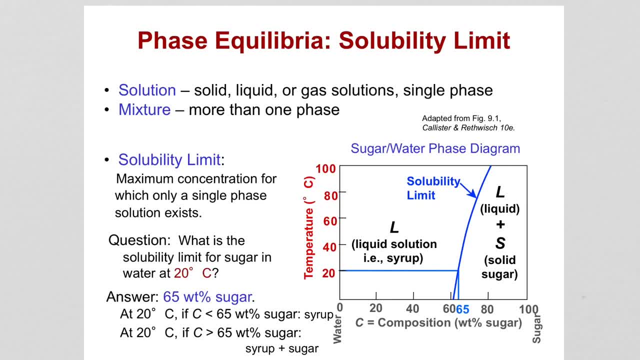 means one single phase. It can be a solid phase, solid solution, or liquid phase, a gas. These are all single phases and the mixture is more than one phase. So, in terms of solubility limit, think about water and sugar system. You keep adding sugar to the 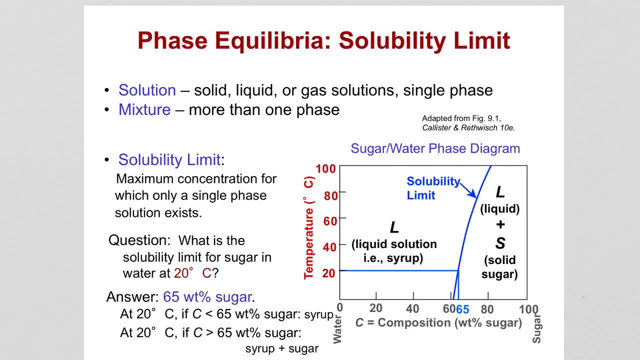 water. First it dissolves and you just have one phase which is liquid. But then, as you keep increasing the sugar amount, it becomes concentrated, The solubility limit is reached and you keep adding sugar. So this is a solubility limit. So this is a solubility limit and you can. 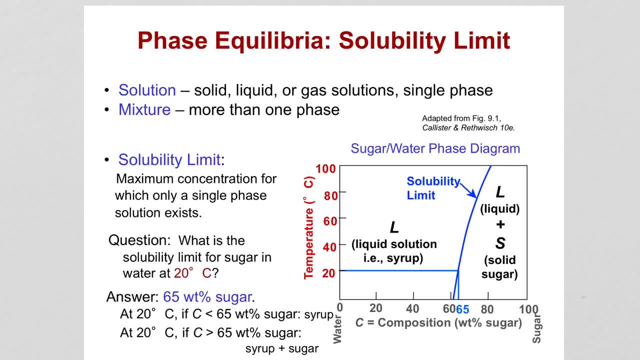 measure the solubility limit. If you have more solubility limits you can measure the solubility. the water cannot dissolve the sugar anymore, so the solution becomes saturated with the sugar. so it is not capable of dissolving the sugar anymore and therefore it's going to separate into two. 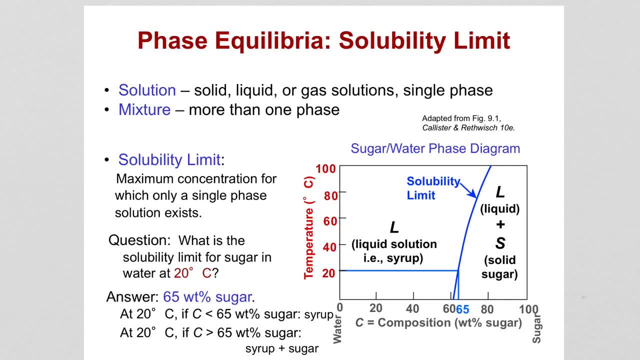 separate phases, sugar and water. so definition of the solubility limit is therefore maximum concentration, for which only a single phase solution exists when you think about sugar and water system. of course, the solubility of sugar will change depending on the concentration, depending on what type of temperature. 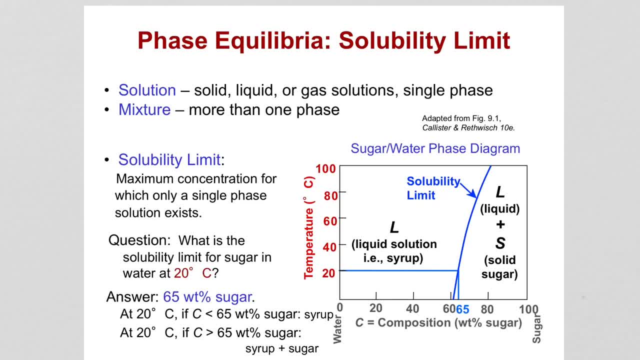 what is the temperature? they all change, uh, the solubility of sugar in water. so we are given a phase diagram of sugar and water mixture. here, as we see in the x-axis, we are seeing the composition, the weight, percentage of sugar, and it is increasing from left to right. 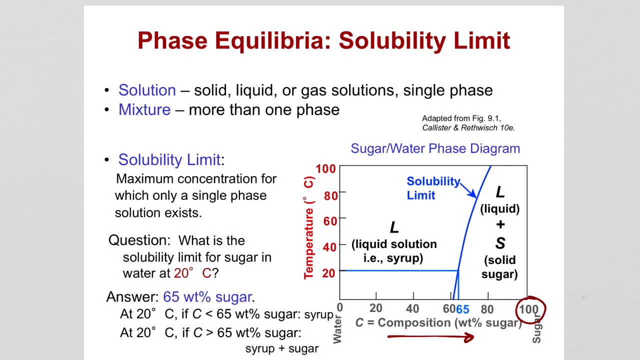 in case of here, hundred percent sugar, zero percent sugar means water. so on the y-axis we are are seeing temperature. Now the phases are separated. So you see, L represents liquid solution and S represents the solid sugar, and different regions, different phases will be thermodynamically in equilibrium. So 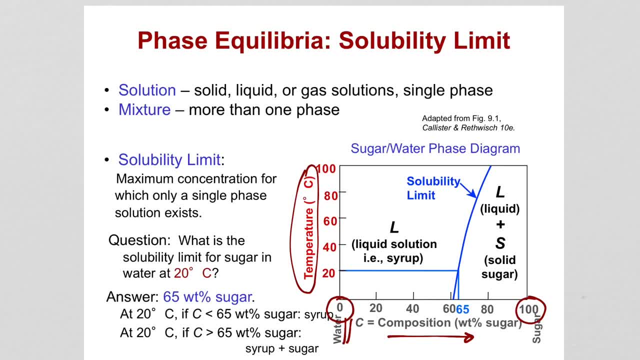 depending on what composition and what temperature you choose, you will have a different phase which is thermodynamically stable. What I'm trying to say. for example, if you have, let's say, 80% sugar and the temperature is 40, and then this is the phase region that your point ends, So that 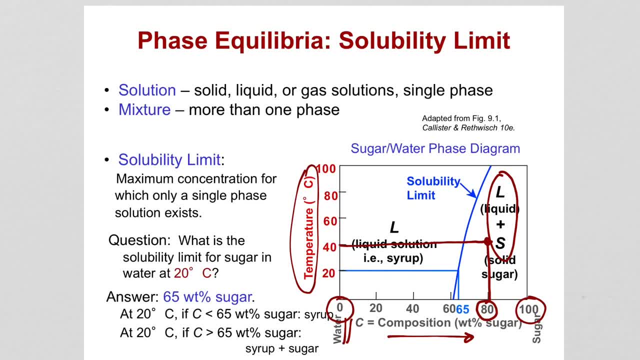 means you have liquid and solid sugar in equilibrium. Okay, so this wasn't just an example Here for you guys to understand, so let's look at now the example. it says what is the solubility limit for sugar in water at 20 degrees C. So, as you can see, at 20 degrees C. 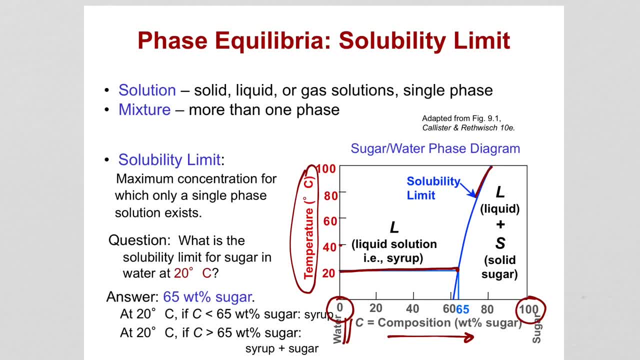 we are. so this solubility limit line is showing us where we cross from liquid to liquid. solid sugar formation. right, if I go further here, that means at 20 degrees C. if I go further compositions, then I will have solid sugar. start the solid sugar in my system, but where does it start to form? it starts to form at 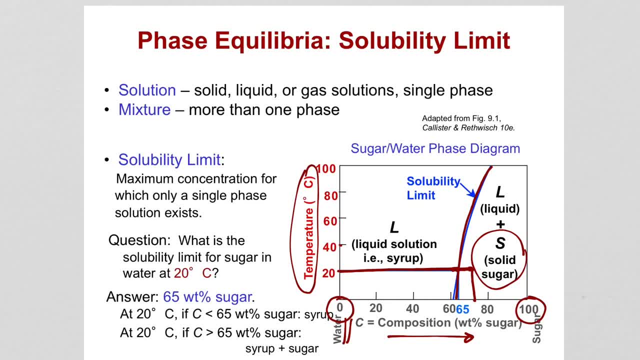 the intersection of that solubility limit line with the temperature line at this point, right, okay. so now then what we need to do. to start from 20 degrees C line- let me choose different color here- we go to the intersection of the temperature line with the solubility limit line and go down to read 65%. so 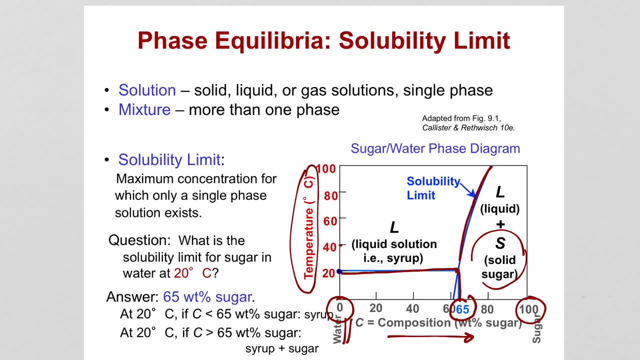 that's the intersection of the solubility limit line and go down to read 65%. so that's the means at 20 degrees C, if you have components of sugar lower than 65%, you will have liquid, which is the syrup itself. so dissolved sugar is dissolved. 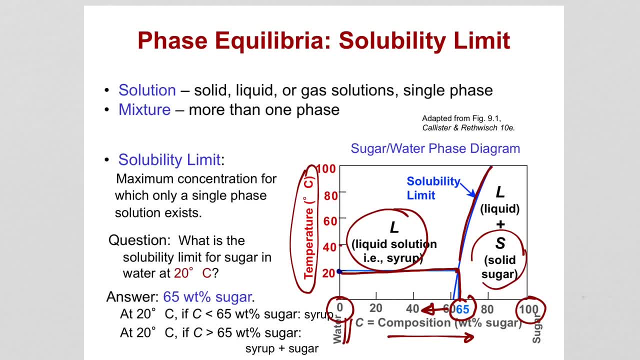 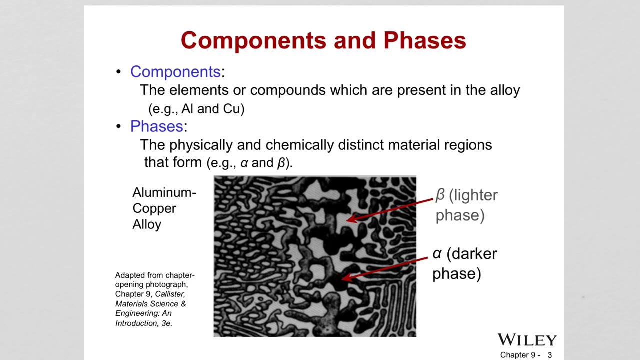 and from the syrup. and then, if you go above temperature, above compositions of 65%, you will both have the sugar and the liquid. so this is the information we obtain for the liquid of sugar at the temperature line, the solid and the from the phase diagram. We need to understand the difference between the terms Here when I say 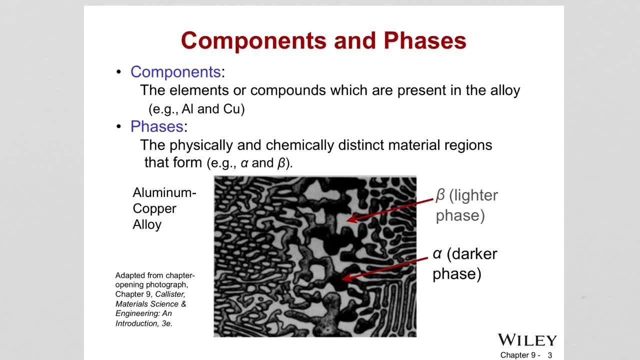 components. that means it is. we are talking about the elements or compounds which are present in the alloy. like we are mixing aluminum with copper. we have two components, but the phase is they are maybe forming a solid solution together. right, so the phase is physically and chemically distinct. 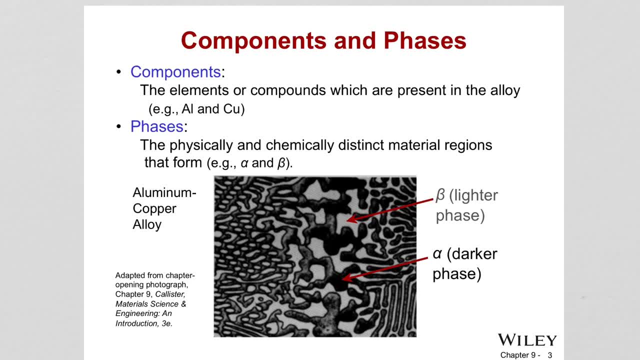 material regions that form and in this microscopic image we are given the structure of an aluminum copper alloy and we are seeing that we have two different phases, because they are good, basically physically different, and one of them is called alpha, the darker phase, and beta it, which is the lighter phase. both are solid. 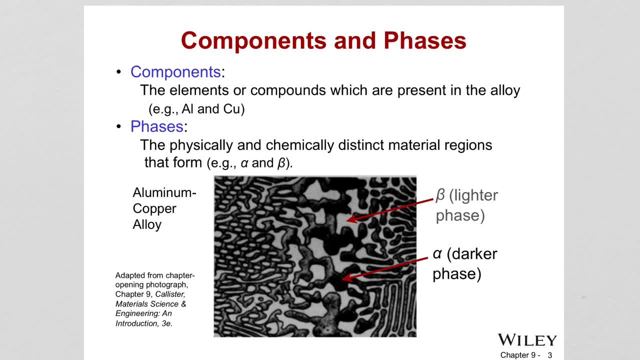 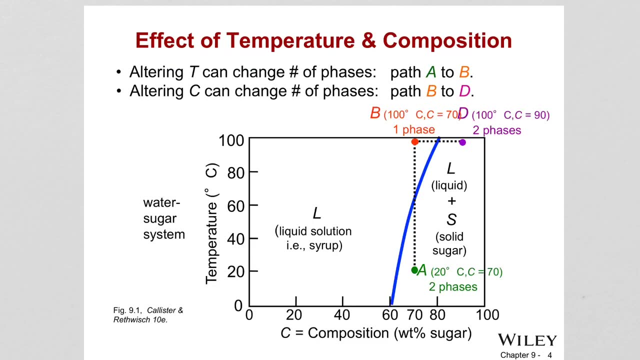 solutions of aluminum and copper. overall the system has two components and two phases. so both the temperature and the composition is affecting what type of phase will be in equilibrium. so if you again look at the water sugar system and as a function of composition and temperature, we are seeing what are the phases that are in equilibrium. so here, 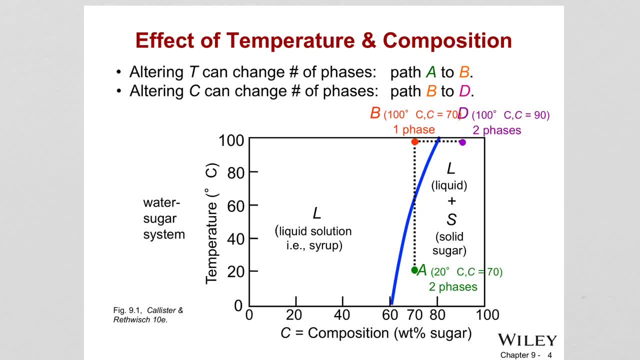 if you keep the composition the same. think about you are going from point A to point B. how can you do that so you keep the composition the same? it's a vertical line, but let's say we are increasing the temperature of the system. therefore I travel from point A to point B. now, at point A I had 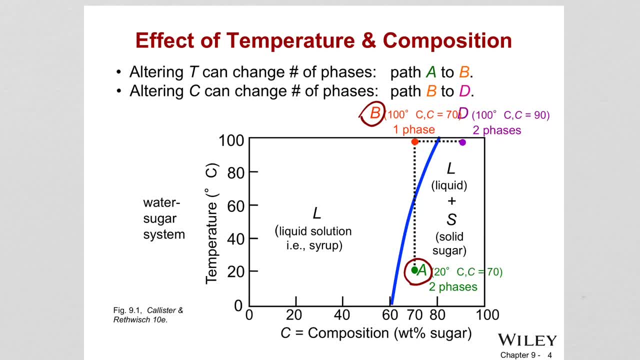 solid sugar in the system together with the liquid. okay, so it was saturated and there was solid sugar in the liquid. now if I increase the temperature I go from A to B. now I have the sugar dissolved again, because at that point- the point B- I have liquid as the stable phase. so that means 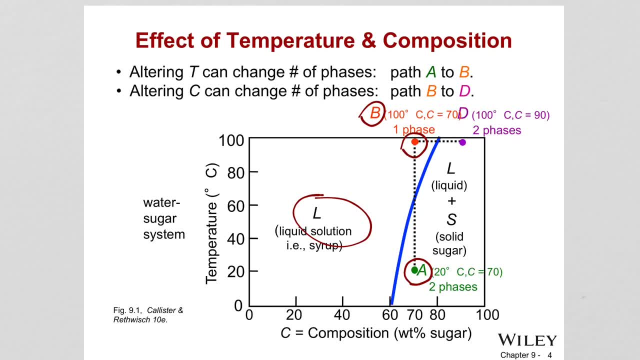 at point A you had two phases, sugar and the liquid, and when you increase the temperature you end up with having just one phase, which is just the liquid, because the sugar now dissolved. you went, you reach to the solubility limit and go ahead and go above. 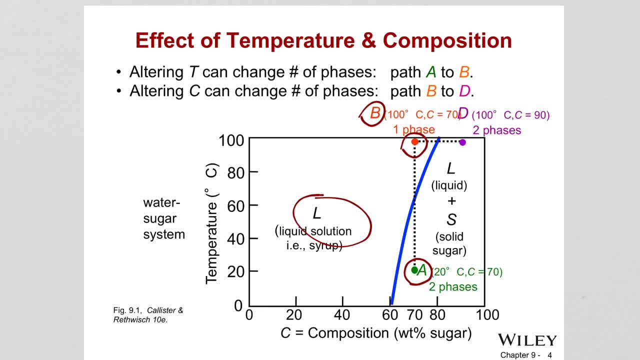 the solubility limit. so let's say you are at a constant temperature and you are changing the composition. let's say you are adding more sugar. if that is the case, let's start from point B, where we had just have one phase and we are going to 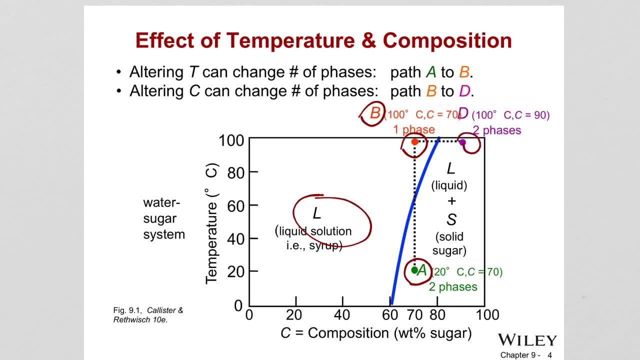 point D: we just keeping the temperature constant, but we are increasing the composition. so if you increase the composition you are again going from one phase and to two phases. there is again sugar. you can observe as another phase inside your liquid because you have now thermodynamically 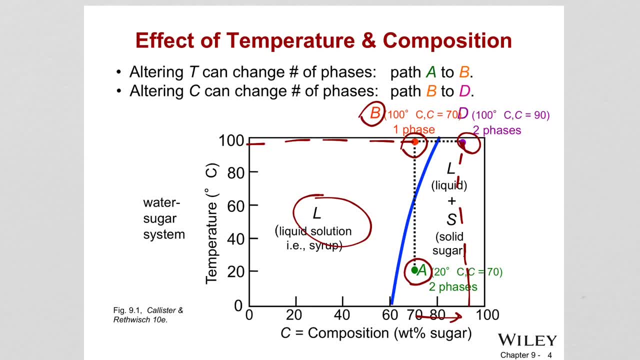 different phase- liquid and solid- is mixed, mixed inside your system. so, as you can see, what does this tell us? depending on the temperature and depending on the composition, different phases will be thermodynamical equilibrium. so different phases will exist in your system, depending on what your composition is and what your temperature is. and we learned. 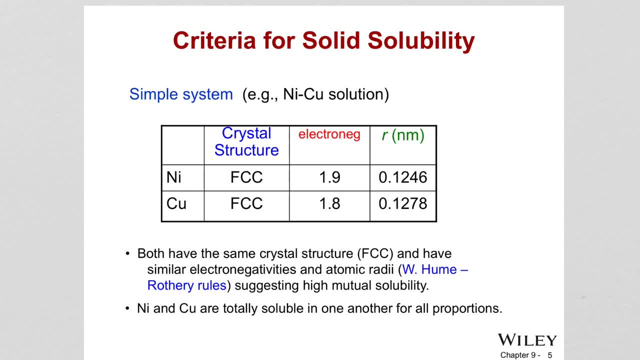 about solid solubility, right for a couple. and nickel system. they both have FCC structure. there are electronegativities, are similar, atomic radius similar. so because they have so close numbers in terms of their electronegativity and atomic radius, basically this suggests high solubility in between each other. in fact, nickel and 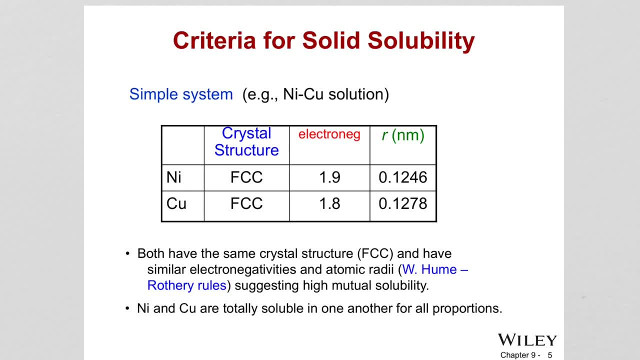 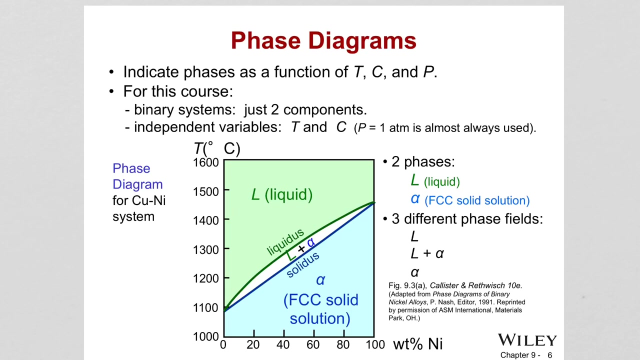 copper are totally soluble in one another for all proportions, so it doesn't matter what composition you have you. they can dissolve in each other at any composition. This is a binary system and it is represented by binary phase diagrams. So we now gonna take a look at the phase diagram of copper and 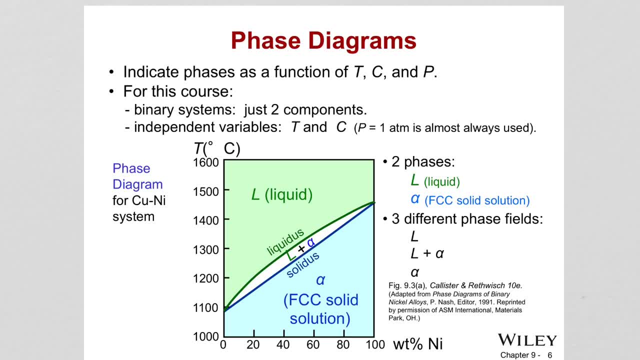 nickel. So of course the phase diagram will show us what type of phase you have as a function of temperature and composition. Usually, when the phase diagrams are plotted, the pressure is always the same, which is kept at one atmospheric pressure. So in this case we said it's a binary system means we 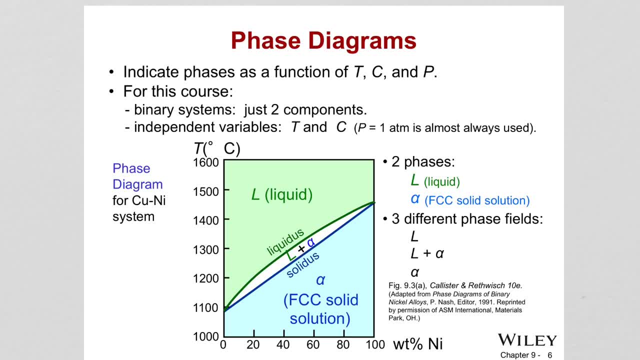 have just two components, copper and nickel. You can change the temperature and composition because they are not depending on each other. So in this phase diagram, for example, we are seeing two phases. So we have two components, copper and nickel, and we have two phase which is liquid and solid, and the solid is FCC solid. 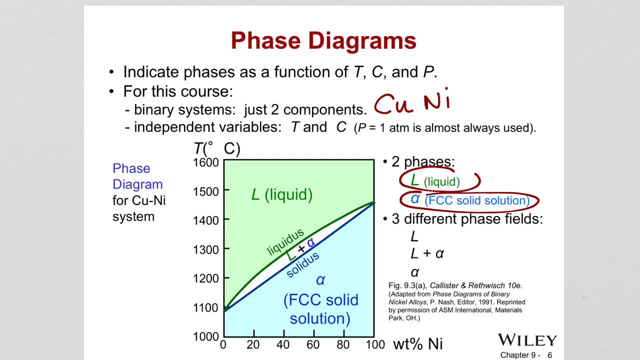 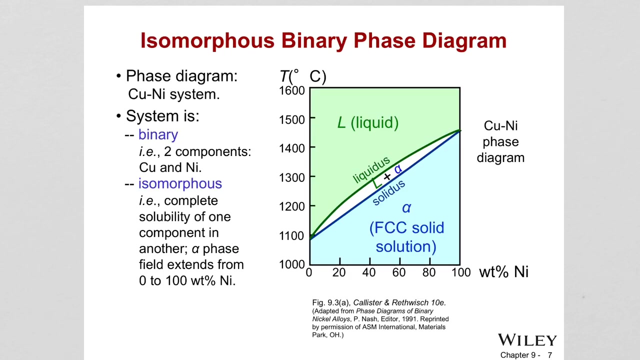 solution, But we have three different phase fields because we have liquid, we are seeing liquid, we are seeing liquid and solid in equilibrium and we are also seeing the solid solution, alpha, as representing three different phase fields. So these are the copper and nickel system is termed isomorphous. 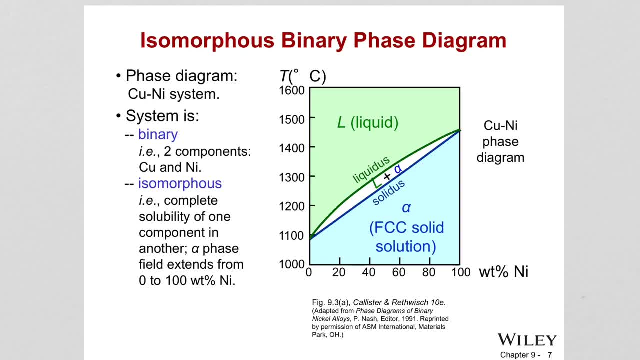 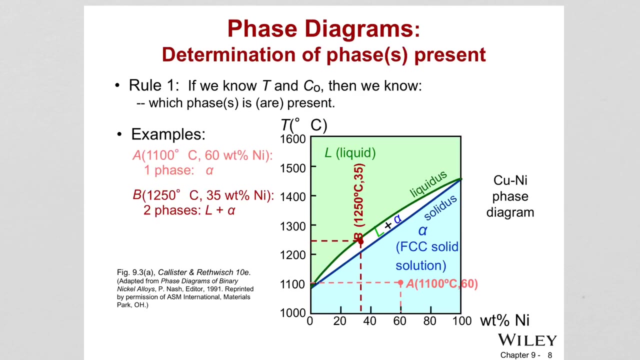 binary phase diagram. This term is because they have complete liquid and solid solubility. So these are the two components in liquid and the solid form. So binary means two components. Okay, we need to understand that. for metallic alloys, the solid solutions like mixture of copper and nickel. when they dissolve in each other, the these solid. 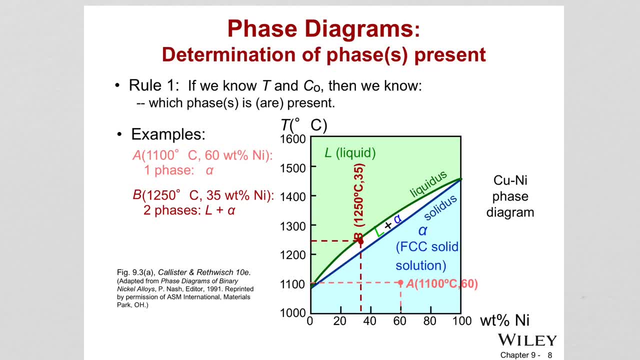 solutions are represented by Greek letters like alpha, beta, gamma, And the lines we observe in the phase diagram is separating the phase fields. Okay, so the line that is separating the solid solution, alpha, from the liquid and alpha phase region is called solidus line, And the line that separates the liquid and 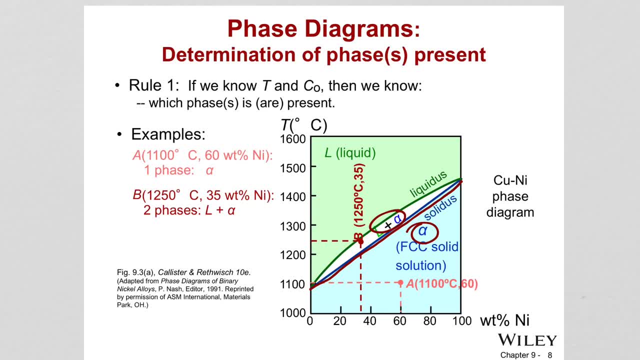 alpha mixture from the liquid. the phase is called liquidus line. So here on the x-axis we have zero, zero percent nickel, because the x-axis is drawn as a function of the nickel percentage of the nickel that is added. So at zero percent of nickel, 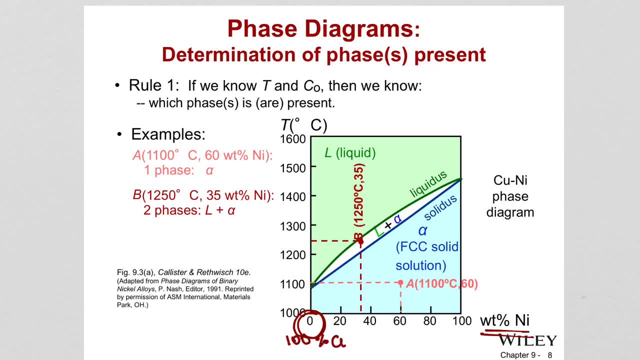 executives had hundred percent copper And at hundred percent nickel you actually have zero percent copper. so these points here- that point is actually representing the melting point of the nickel itself and this point here representing, if I go above this part- well, two points are represented here. 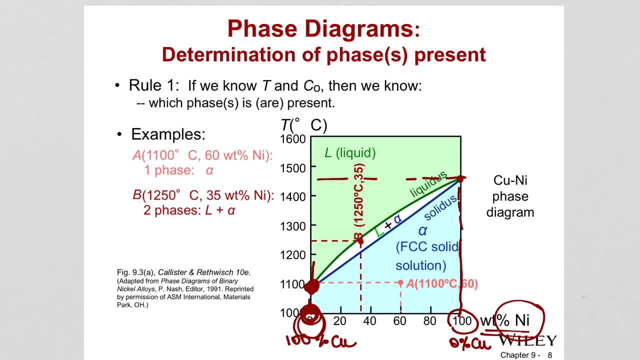 Right representing the melting point of copper copper- pure copper. One is pure nickel, one is pure copper. But, as you can see, the melting point is increasing as a function of melting points are increasing as a function of nickel addition Because to see the melting point of the alloy you need to look at from the 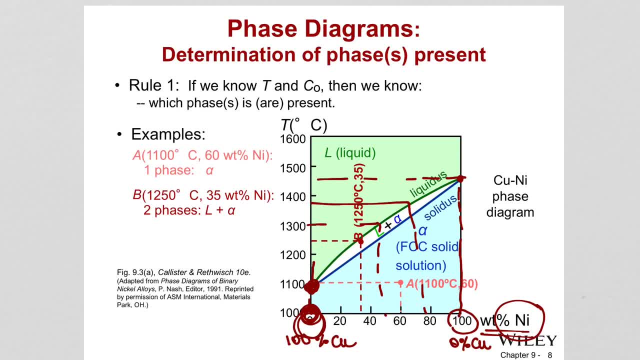 composition of that alloy. Go upwards, draw a vertical line, as I did, and go to the intersection of the liquidous line and then read the corresponding temperature on the y-axis. Okay, So, as I said before, if you are given the temperature and the initial composition, 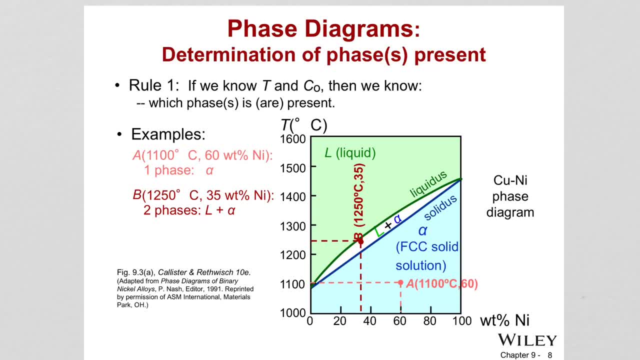 않은 sabaç kimi nut of that alloy. You know what the temperature is, what is the initial composition is. You can figure out what phases you have. For example, point A: We are given it is at 1100 degrees C and at 60% weight percent of. 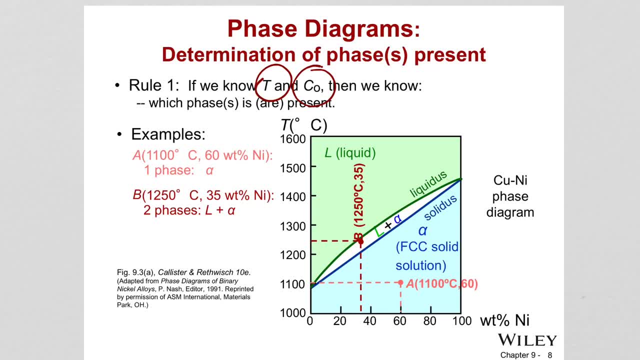 nickel. It puts us to a point where we are at alpha region. So alpha is a solid solution, right? If we have a temperature of 1250 and the composition is 35 weight percent nickel, then we are at a position where it's actually we are at the phase of liquid plus solid mixture. 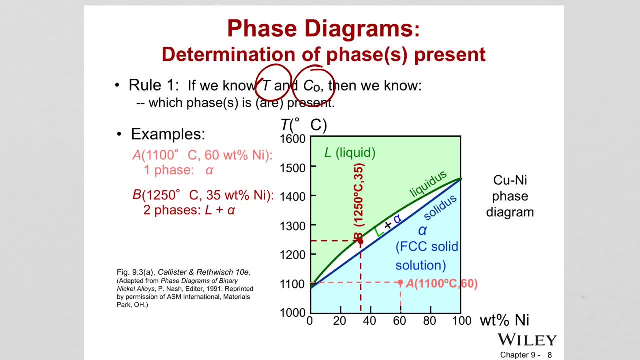 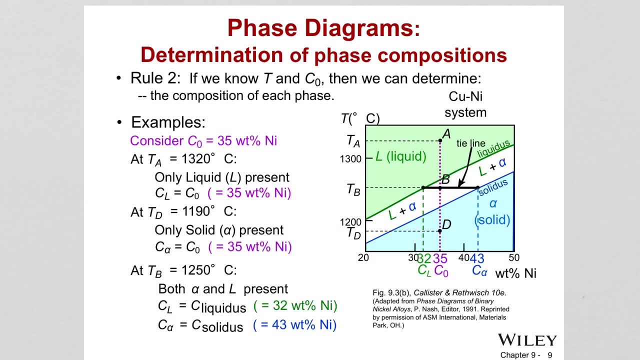 So liquid and alpha Is it? It's a mixture, exists in equilibrium. Now let's take a look at how we can determine the phase compositions. So if we know the temperature and initial composition C naught, then we can determine the composition of each phase. 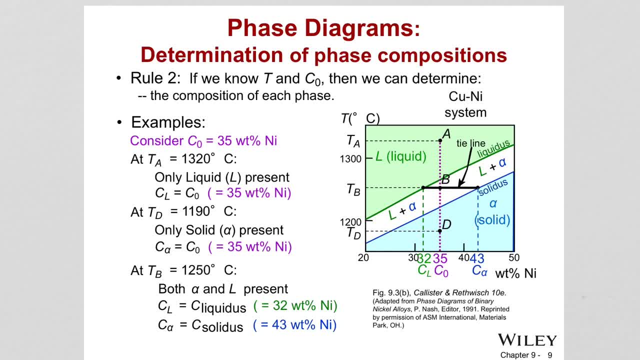 For example, consider an alloy which has 25% nickel, So automatically 65% is copper. Of course you guys can understand that right. So when I have an alloy which has 35 weight percent nickel at temperature 1320 degrees, 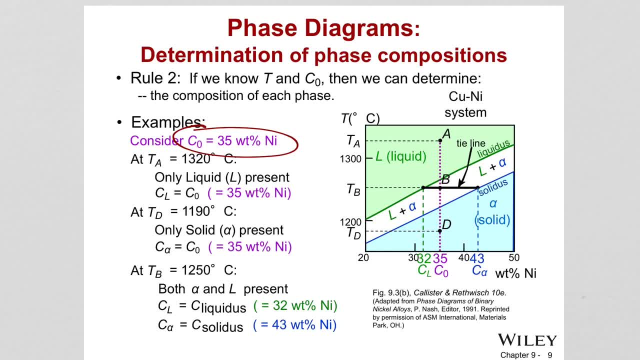 C, What is the phase that is present? So let's look at it. 35, I locate from the x axis and I find the temperature, my temperature line ta, which is 1200 in 1320, and I go here and intersection, I find that I am located. 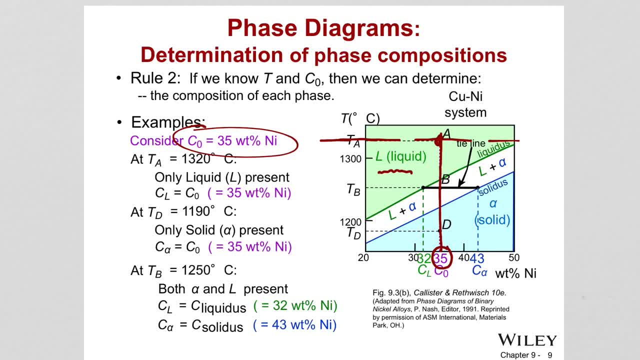 in the liquid phase. So I only have liquid. So If that is the case, if you have one phase and then your, that means your initial composition and the composition of the liquid is the same. That means with in the liquid. also, it is 35% nickel and 65% copper. 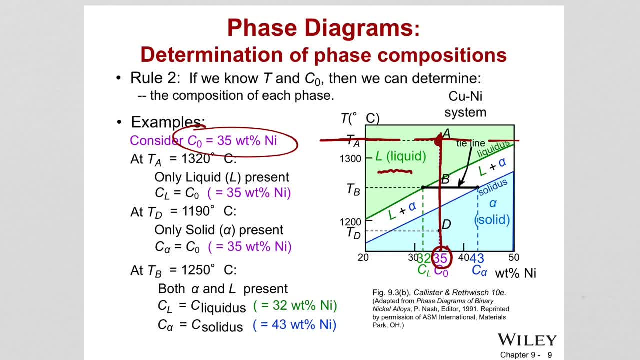 Okay, If you are at point D, for example, which is at a lower temperature, But the same composition again, you are at a point which is within the alpha phase region. Therefore, you just have a solid solution, solid solution of copper and nickel. 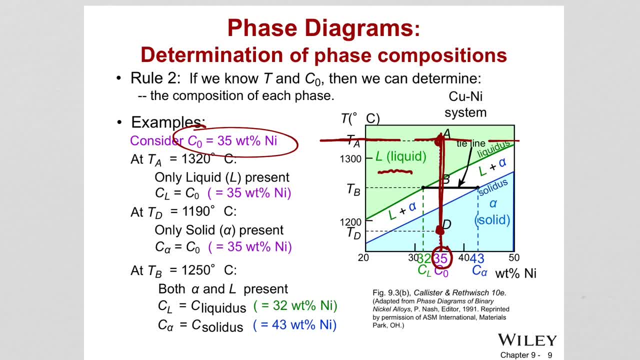 And in this case again, you just have one phase. That means the composition of the solid is equal to the initial composition of the alloy. So again, the total composition of the alloy is equal to the initial composition of the alloy. So I any more solid solution of copper with 35% Alpha is still because I had. I had the 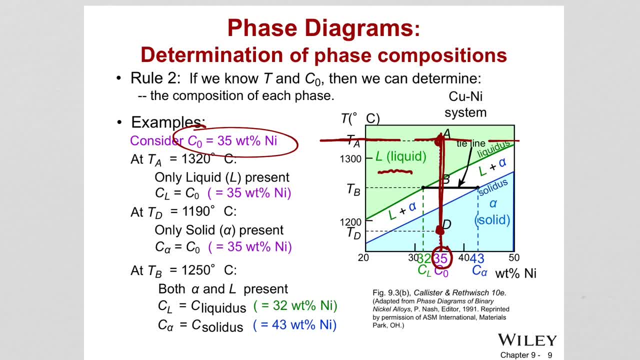 solid and yellow and negative reaction was the solution. I mean, if I have it, if I have the further ice here, it still will be solid. If I have a solid base, the solid is still, but I have a solid, So I am going to use theissa surface and for the higher I am going to use theiss Line. 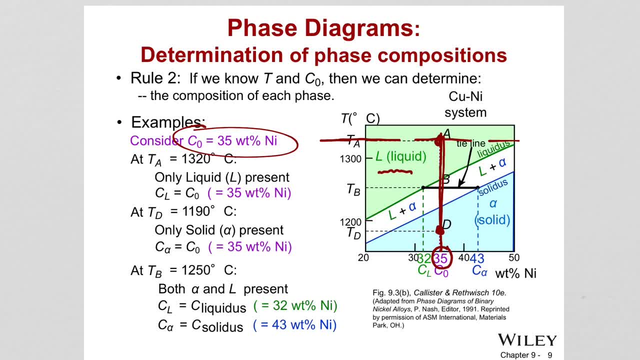 Donans, We are looking at the actual location of our liquid. What is老이� 해요? This is the normal. I mean, this is actually not regularly made. It looks still and not, But we put our solid on top. 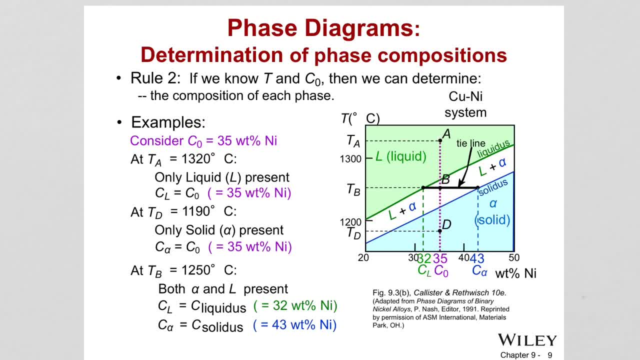 Unfortunately, this is in. It's still possible right now. Yes, So when that is the case, you start with the same composition and we are given the temperature is 1250.. And then it puts us to a point where the two phase is in equilibrium, which is liquid and alpha. 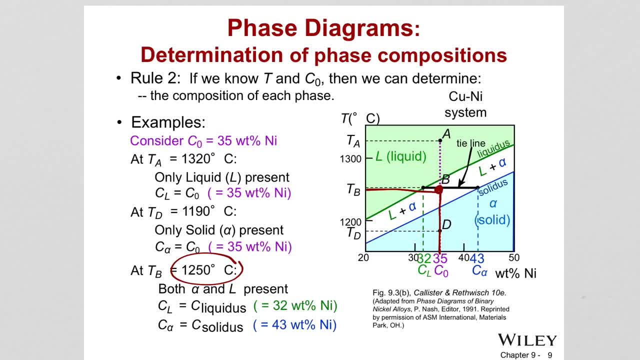 So the question is how much of nickel there is in alpha or how much nickel there is in liquid. So to understand that we need to draw a tie line, Tie line is the line at that temperature which connects the intersections of that temperature line with the liquidous and solidous line. 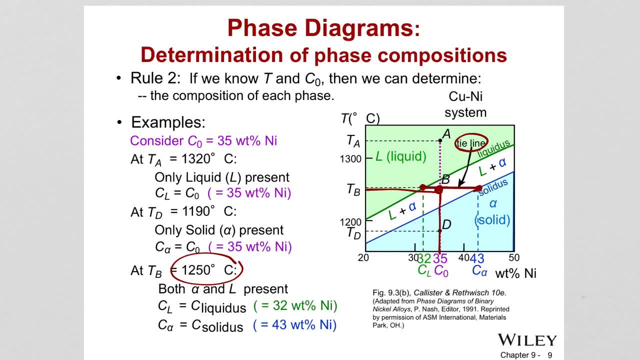 So, from the intersection, Intersection of that tie line with the solidous line, If I go down and read the composition, that composition, because it's the intersection with the solidous line, is going to give me the composition of the solid, which is the composition inside, I'm sorry, the percent of nickel inside the solid phase. 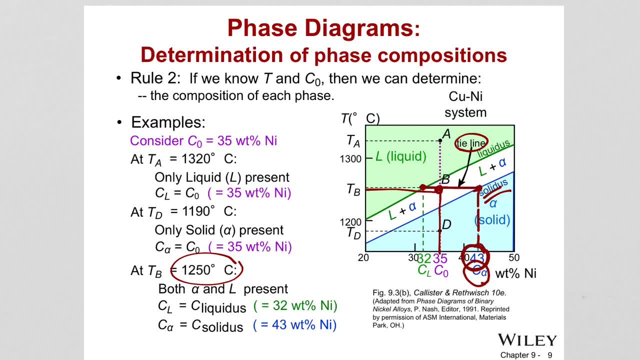 So that means 40.. 43%, 43% nickel is in the solid phase. Okay, So the composition of the solid is equal to C, with the subscript alpha which is 43.. Okay, So what about the composition of the liquid? To understand the composition of the liquid, this time I go to the intersection of that tie line with the liquidous line. 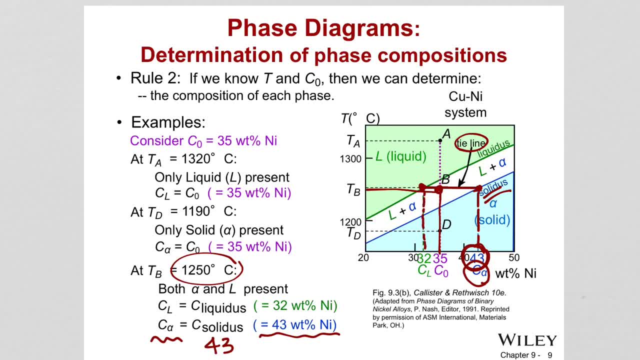 Which will give me the composition of the liquid. If I go down CL, which is 33%, That means within that liquid, the 32% of is nickel. So this way we figured out the compositions of the liquid and composition of the solid. We didn't figure out what is the amount of solid or what is the amount of liquid. 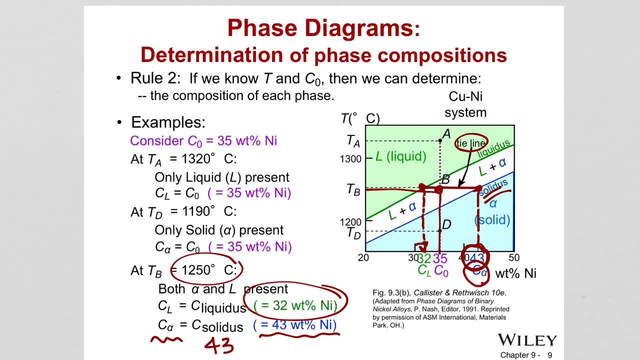 We just figured out the compositions of the liquid and alpha phase. So how much nickel in the solid, how much nickel in the liquid? It is not the liquid percentage or the solid percentage That is different. We're going to take a look at that now. 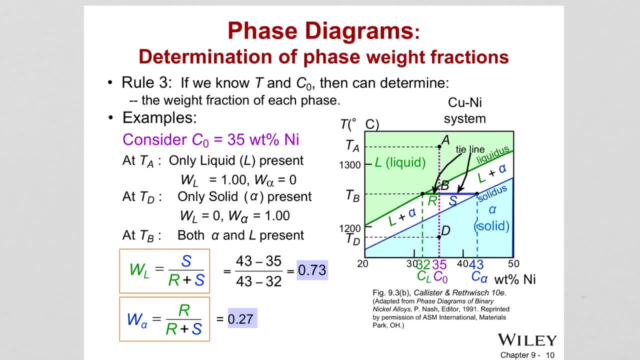 So if you know the temperature and the initial composition, You can determine the weight fraction of each phase. What does it mean If you are in a phase that where you have liquid and solid in equilibrium and the liquid and alpha? in this case, that means you can figure out the percentages of alpha and percentages of liquid, How much liquid there is, how much alpha there is in the overall alloy mixture. 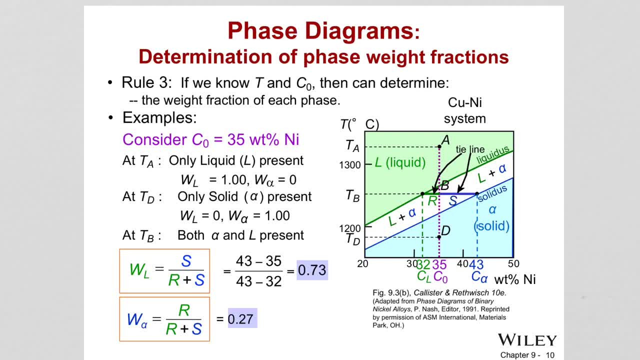 So let's do the same example Here. Okay, and in order to calculate the weight fractions of each phases, there are equations used and we call this lever rule. So these equations are given to us. For example, if you want to calculate the weight percentage, weight fraction. 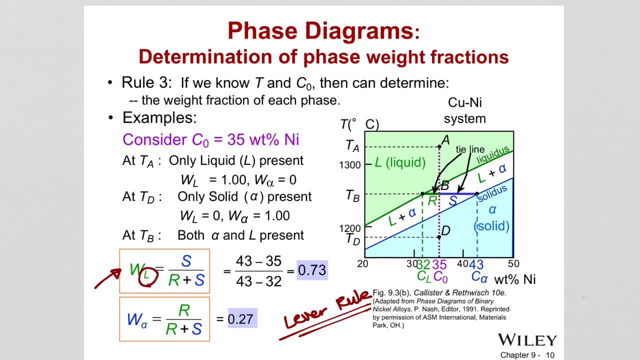 Of the liquid phase, you have to use this equation. Okay, and if you have the want to calculate the weight fraction of the solid alpha phase, you're going to use this equation. And let's see now how we're going to use this equation. 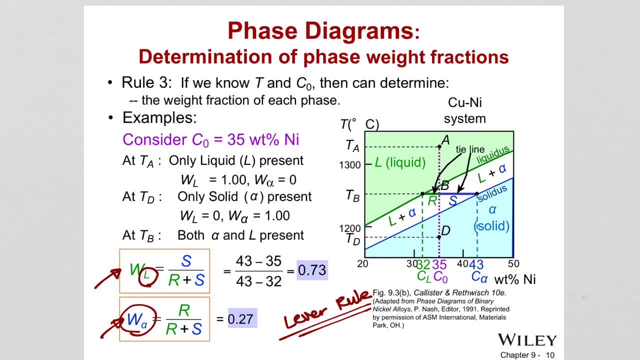 Okay, so Initially we have 35 weight percent nickel- Okay, our CNOT original composition. And at point A We have, And with it corresponding to that temperature, We figured out that we just have liquid. So what is the weight fraction of liquid then? 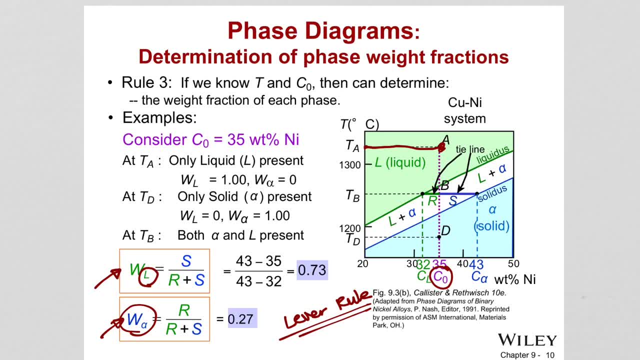 Hundred percent. right, The weight fraction is one. So we don't have any alpha. So alpha is zero. What about at point D? So the same composition, Different temperature, Corresponds to point D. At point D we just have a solid. 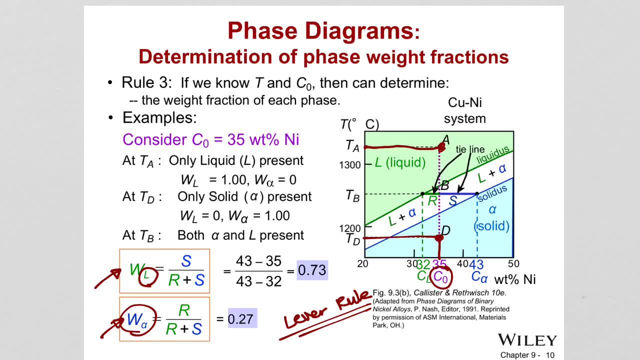 And the solid is the only phase that presents Meaning. it is hundred percent solid And the weight fraction is: therefore, It is one. Okay So, because we don't have any liquid phase. So if we are at the point B, Where, and at that temperature, 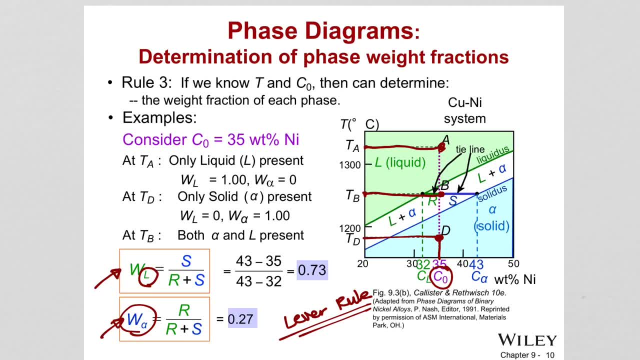 We are here in point B, Where we have two phases, Liquid and alpha. What you need to do to calculate the weight fractions of each phase. So let's say you want to calculate the weight fraction of the liquid, Of course you're going to go ahead. 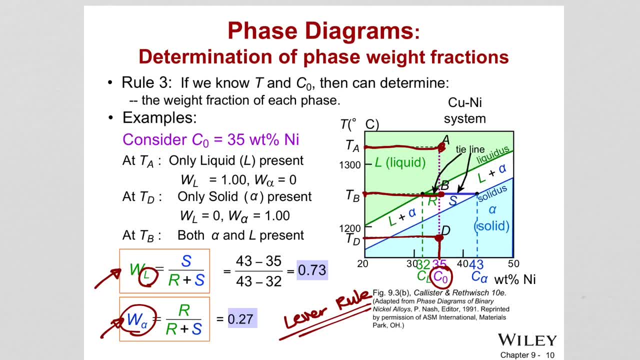 And read the intersections of liquidus and solidus line First, you're going to find the composition of the liquid And composition of the alpha, As we did in the previous slide, Right. So this was the composition of liquid And this was the composition of solid. 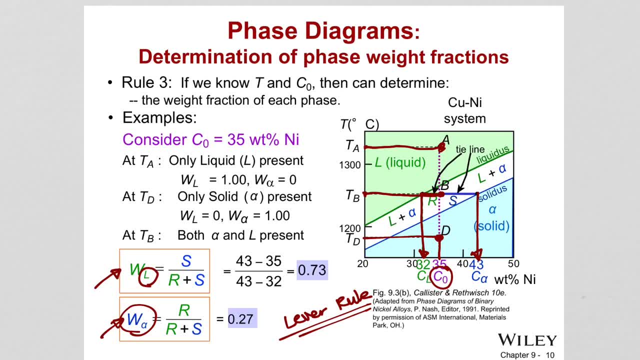 So using that information- The composition of liquid and composition of solid- We can calculate the weight fractions. So in this equation It is given to us as S over R plus S, So those are representing these lengths Or the ranges of these. 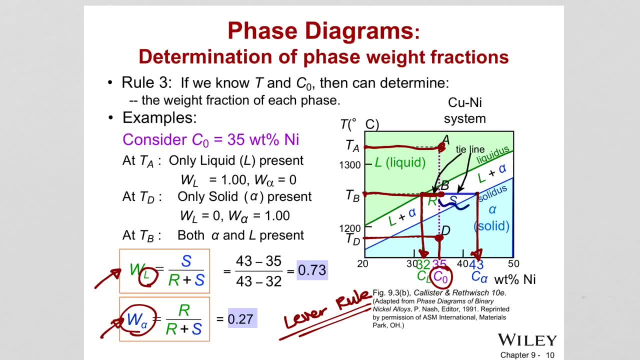 As letters are given in us in the phase diagram. So this is R, This is S. So I don't like this type of this equation Actually written this way. What I can tell you is We can use this equation Because it is the same. 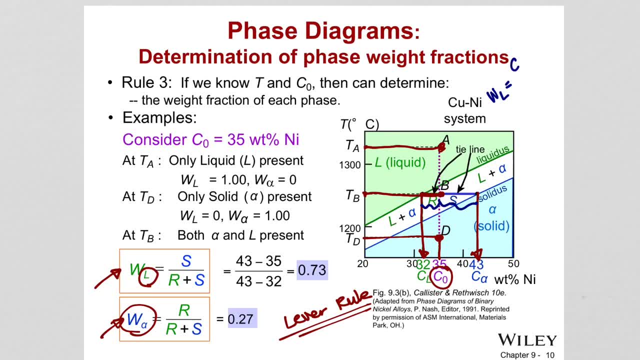 Right. So S means Copper. I mean the composition of alpha Minus the initial composition, Because that is the distance Right. Distance S Is 43 minus 35. Which is the composition of alpha Minus the original composition. 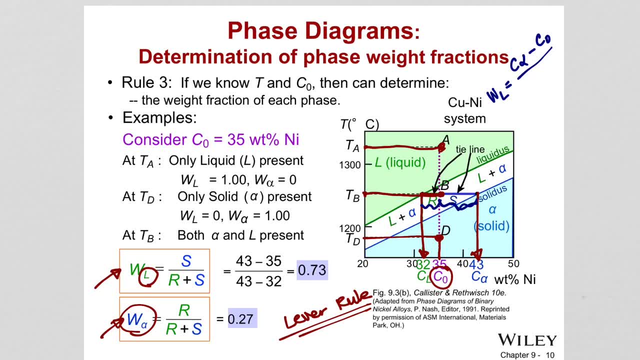 Over the sum of, Over the sum of the R and S: Meaning 43 minus 32.. Meaning C, Alpha Minus C, L. Okay, So the equations will be given to you this way. Okay, And from here? 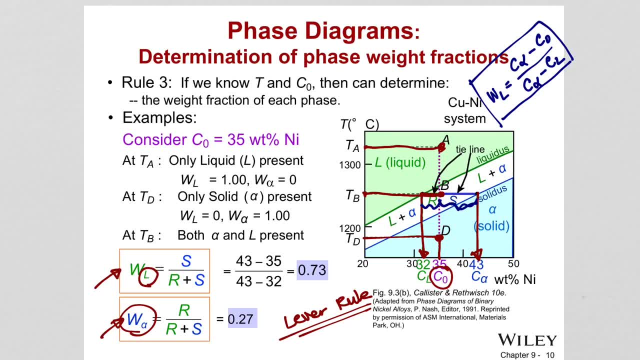 Now you can calculate The weight percent. Weight fraction Of the liquid. So all you have to do: C alpha is 43.. Minus C, naught is 35.. Over C alpha is 43.. Minus C, L is 32.. 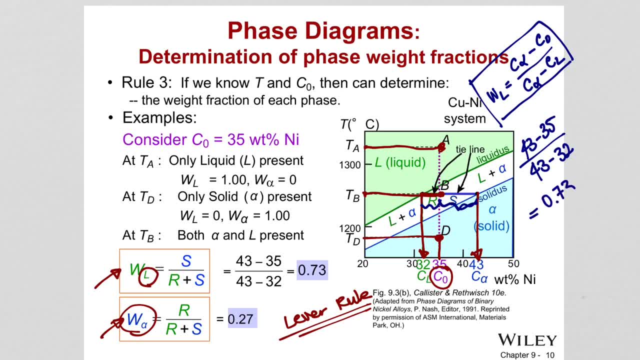 This will give you Point 73. Or 73 percent Of The overall Alloy Is liquid At point B, Okay, And the remaining, Of course, Is going to be the Solid. But to find the solid, 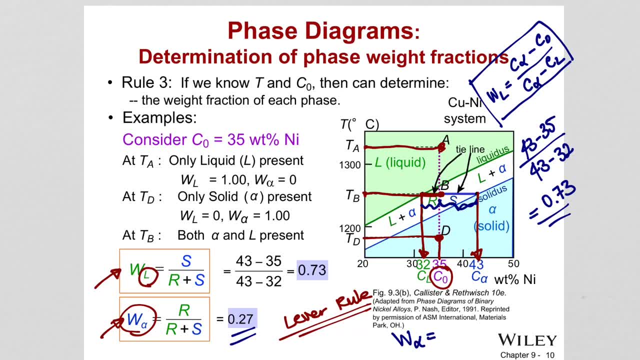 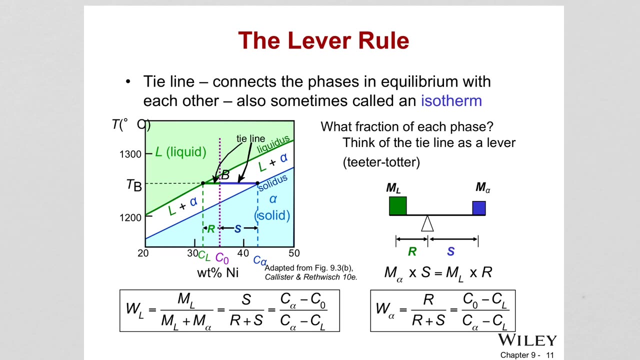 You can again Use this equation That is going to be C naught Minus C L Over C Alpha Minus C L. Okay, You can use it To figure it out Yourself. 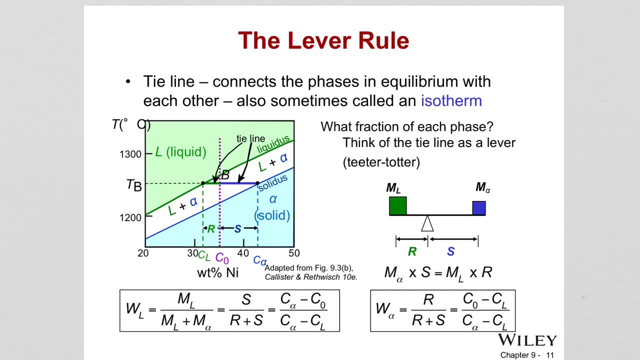 Okay, So In this Slide We are Going to be shown How to Derive This Level Rule. Okay, So We are At Point B, Right there, Right And The. 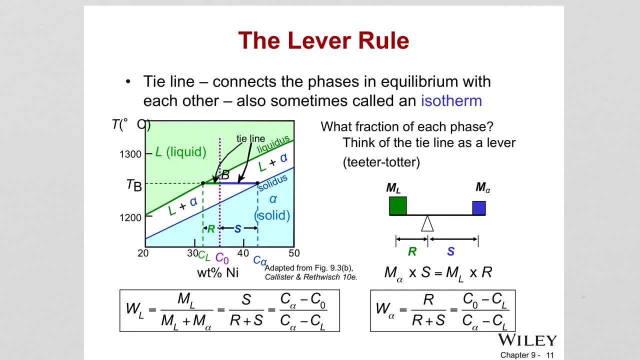 Phases Of Liquid And Solid Is Derived. So We are At Point B, Right there, Right, And The Phases Of Liquid And Solid, Alpha They are. 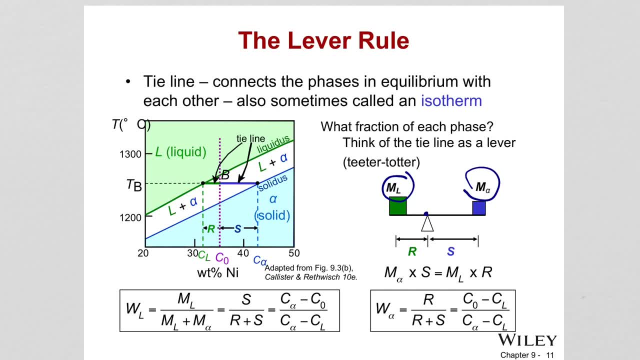 In Equilibrium, Their Weight Right, Their Masses. So What Are? Their? Distance To The Point B Is R And S. So, Basically, Because This Has 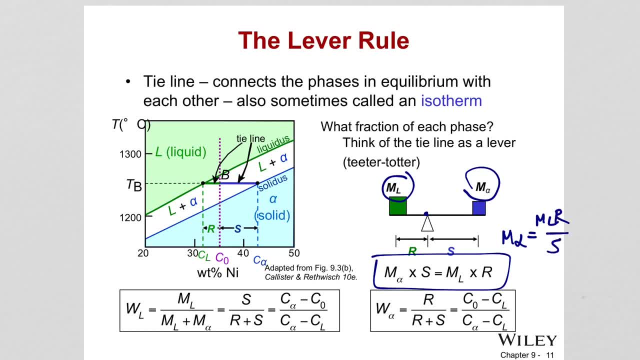 To All Our S. Okay Now, If You Want To Calculate The Weight Percentage Of The Liquid, That Means We Are Just Dividing The Weight. 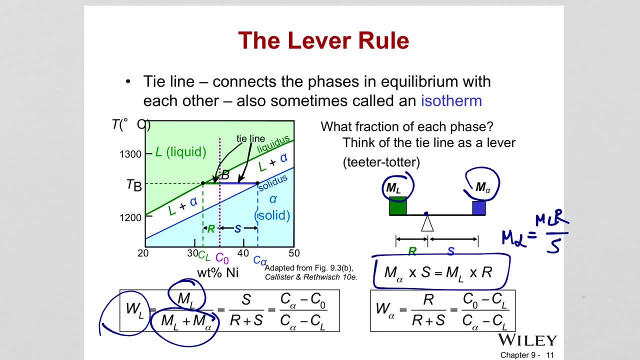 Fraction Of The Liquid That. So This Is Going To Give Us The Weight Fraction Of The Liquid Phase. So If You Come Here Put This, 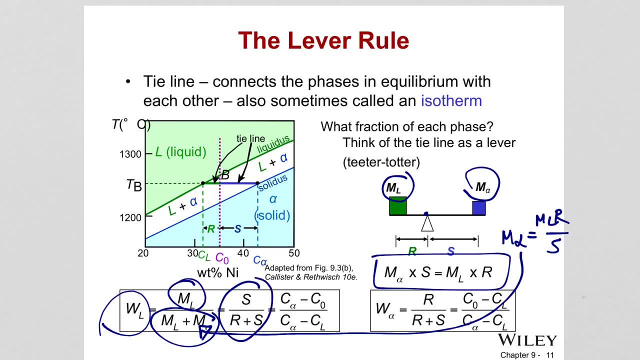 In Here. Okay, Put It In M Alpha, And We Know: R Plus S Is C, Alpha Minus C L. So This Is R Remember. 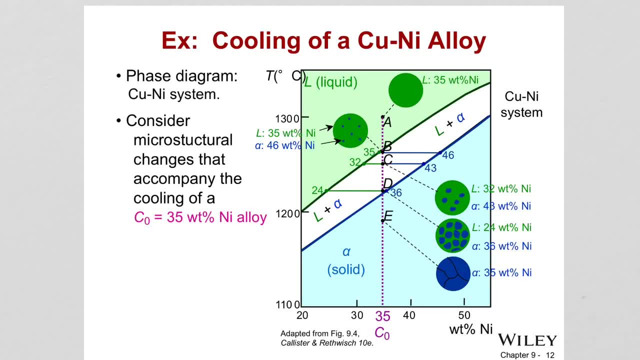 This Is S. That's Where The Differences Coming From. So We Have The S And Can We Look At How The Microstructure Changes, Like Under. 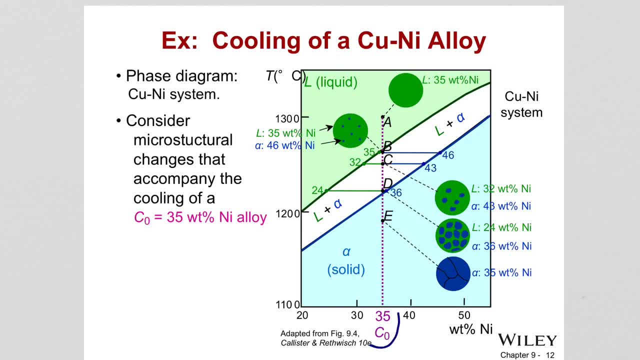 Microscope. Right, How The Microstructure Changes Is A Function Of Temperature. Let's Say, At This Composition We Have, So Let's See How The Microstructure. 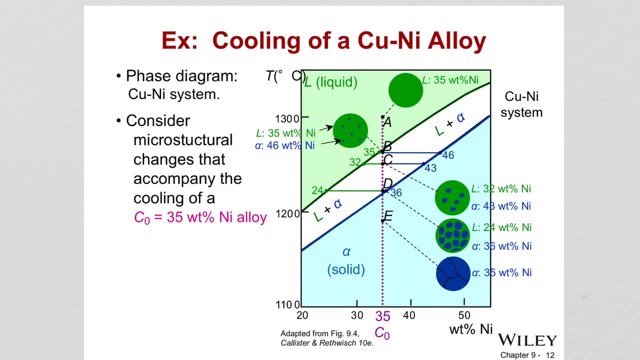 Is Changing. So At Point A, We Have A Pure Liquid And Its Composition Is 35. Weight Percent Nickel. And When We See At Point 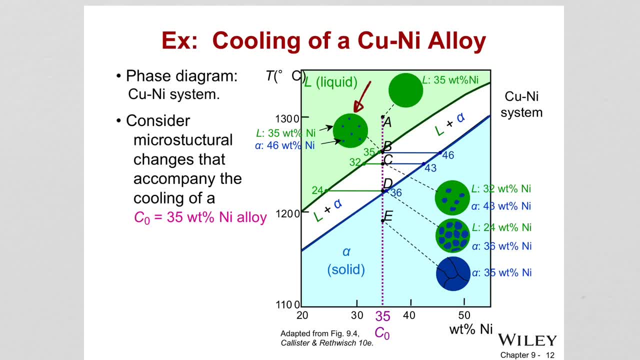 B. The Microstructure Shows That In The Background We Have Liquid Which Is Shown With Green And Solid Face, Which Is The Blue Face Is 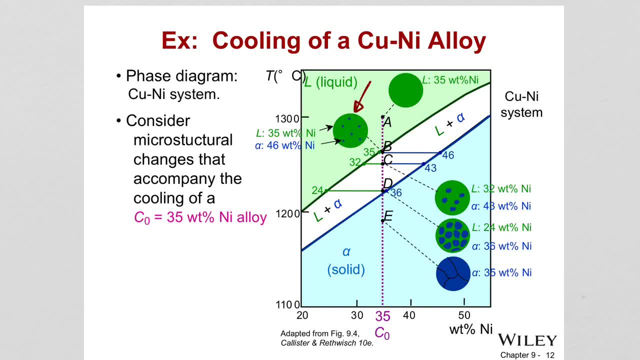 Starting To, And Its Intersection With The Liquid Is Line Show Us 35.. Its Intersection With The Solid Is Line Shows Us 46.. Percent Nickel. 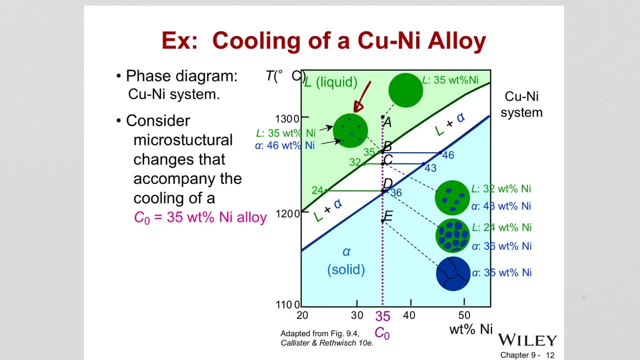 That Means That The Liquid Composition Means The Nucleated Particles Of Alpha Now Getting Bigger Right Inside The Liquid. They Are Getting Bigger. 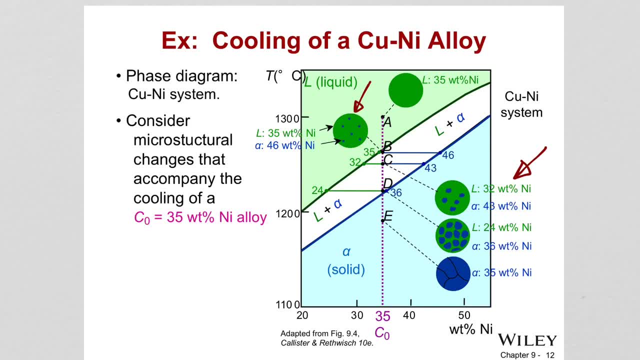 Growing Because We Are Cooling It Down. You Are Solidifying The Material- liquidus and solidus line And liquidus line intersection shows us a composition of 32.. That means we have 32 percent nickel in the liquid and again 43 percent of nickel in the 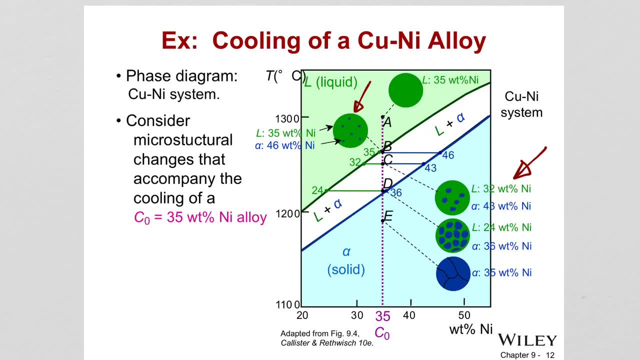 solid because it's the intersection of that tie line with the liquidus line. right here I read it And then we keep cooling it down. Now we came to point D. We still have a mixture, mixture, but the solid is getting bigger, As you see, with the blue here. And what about the? 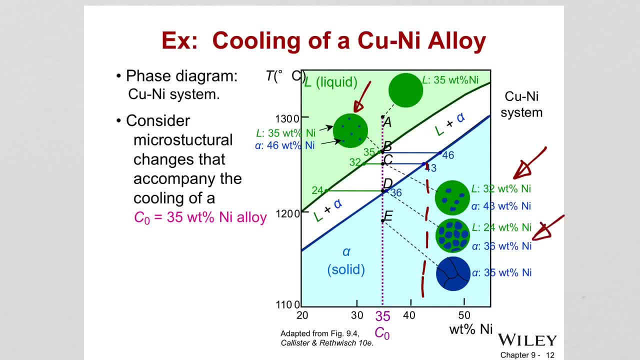 percentages of the compositions of the liquid and alpha. Again the same way. we read 24 and 36.. 24 for the liquid composition and 36 with the for the solid composition. After that, point D: we kept cooling down and we came to point E. At point E we just have: 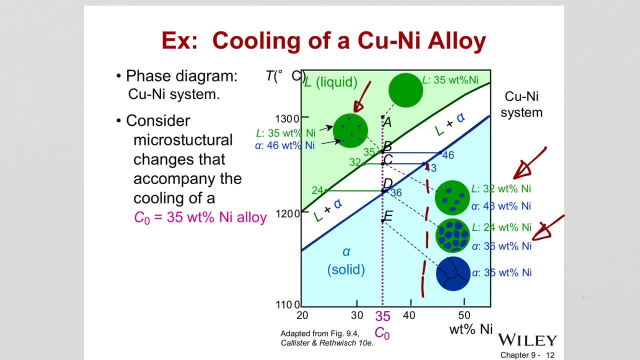 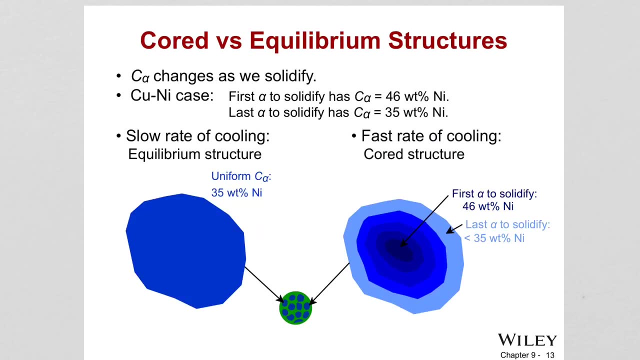 two conditions: a solid phase, and you can see how the solid form with grain boundaries and the composition is 35, 8% nickel. now there are differences between doing a slow cooling and fast cooling, and the phase diagrams are obtained for slow cooling rates when we provide enough time to atoms to diffuse into 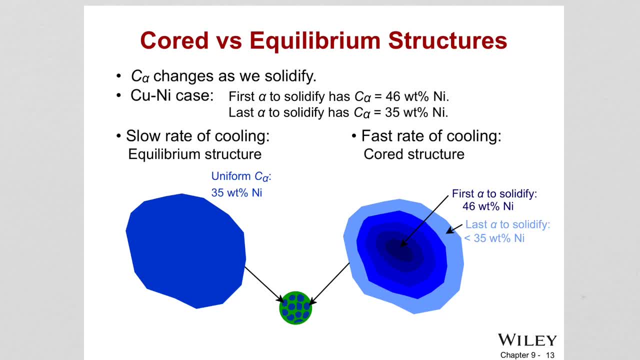 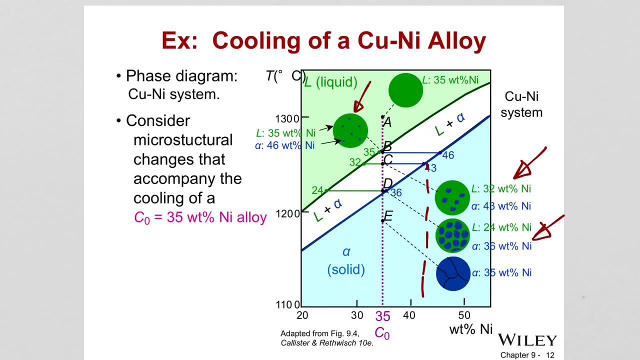 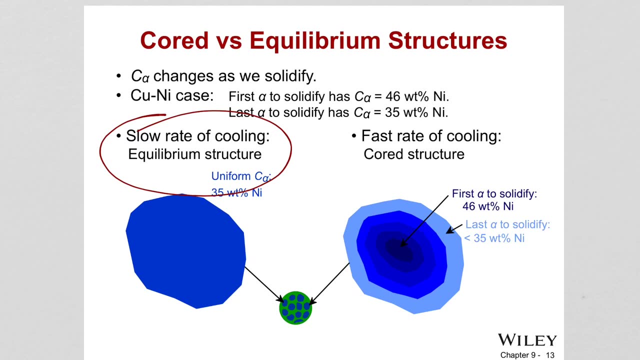 their equilibrium structure. so if you do solid so slow, cooling rate, that means at the end. at the end means if, when we reach the stage a, we have a uniform structure, means everywhere the nickel composition is 34- 35 percent. but if you don't do it so fast and don't allow the atoms to reach their equilibrium, 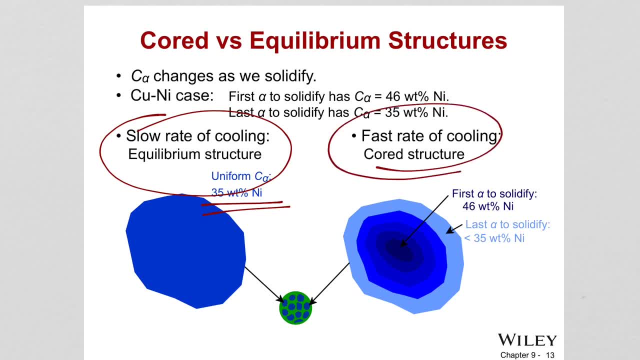 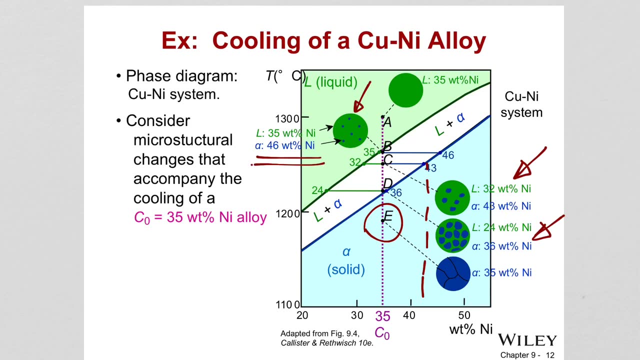 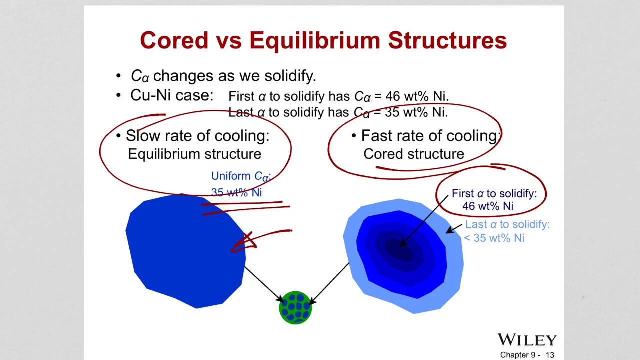 you do it fast, that means you will have a chord structure. that being said, the initially solidifying phase will have 46 percent nickel. here we see it right: initial nickel weights. they have 46 percent nickel and you need to end up with 35 percent. if you do it slowly, you end up with 35 percent, but 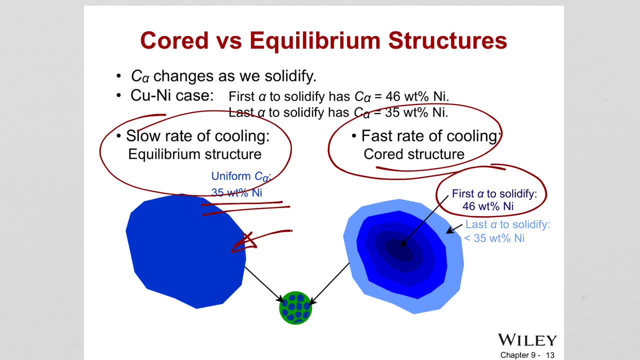 if you do it fast, what's going to happen? you will have layers of different layers of the same alloy, but the composition is different throughout the structure. so the last part that solidifies should have 35 percent, but there's going to be a range of compositions in the structure. 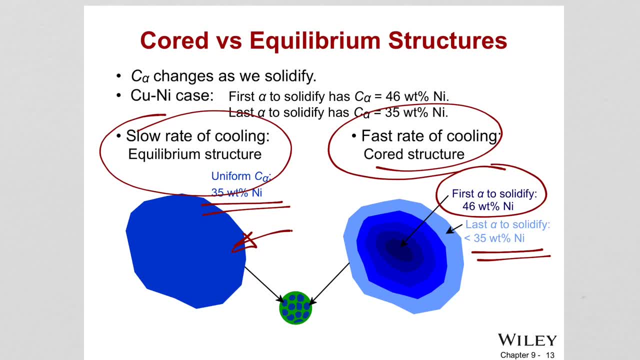 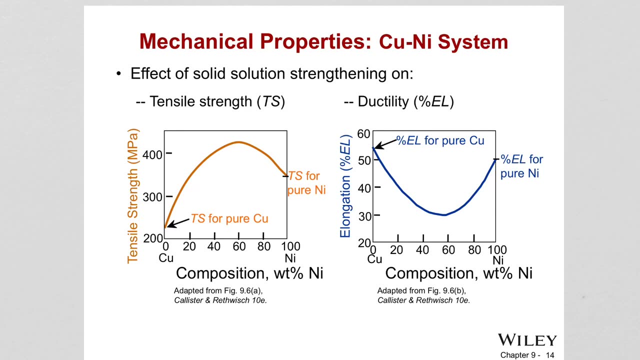 you it's not going to be a homogeneous structure because you don't let enough time for atoms to move to their equilibrium positions Here, as we have seen in the strengthening of materials. so if we look at the copper- nickel system, you can see the effect of solid solution hardening on the tensile strength and ductility. 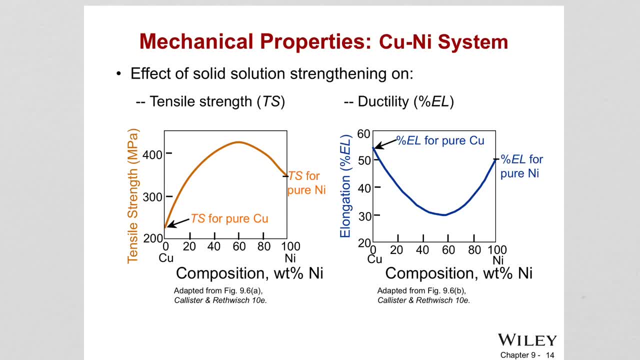 and as we increase the composition of nickel in the alloy, the strength is increasing initially and then reaches a certain point- 60 percent, let's say- reaches a maximum. As you keep increasing the nickel amount, it's actually causing a decrease in the tensile strength. So that means actually: 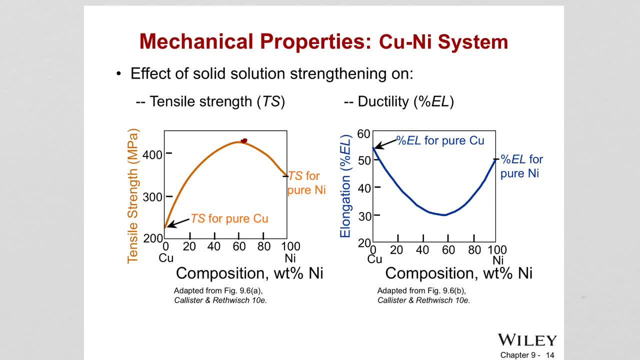 there is an optimum composition where you actually achieve the highest tensile strength. This is the same, of course, tensile strength. if you look at the ductility, similar behavior, Of course. this time the ductility is decreasing with increasing nickel concentration until a point 60%, and then again increases. 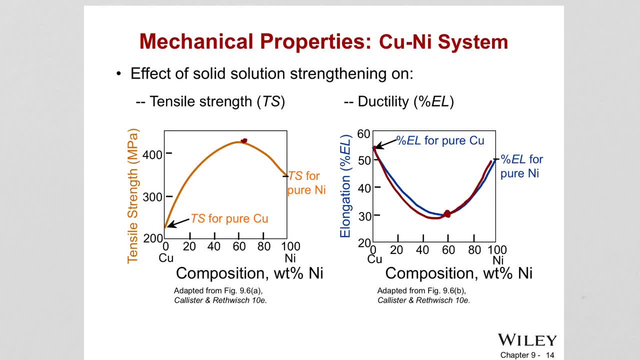 So this 60% of nickel seems like the optimum composition for the copper-nickel alloy. So these tests have to be done for different types of alloying systems to figure out what is the optimum composition at a certain temperature. So they kept the temperature constant here. 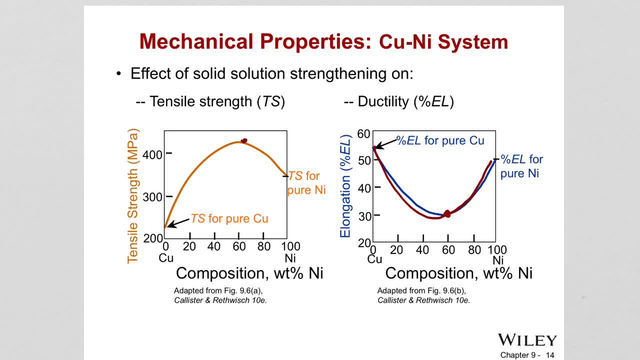 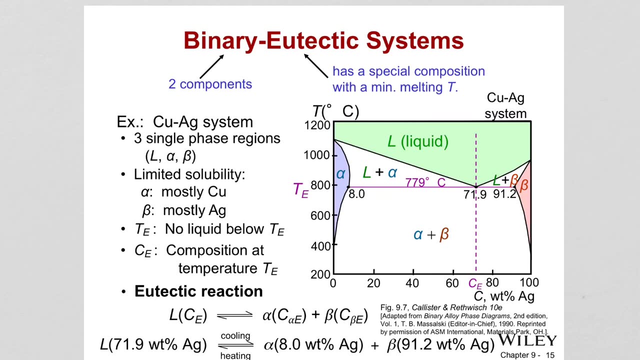 And then they are looking for how the properties are changing with the addition of nickel. Now we're going to take a look at binary eutectic systems. Binary means again two components. Eutectic means this mixture has a special composition with a minimum melting temperature. 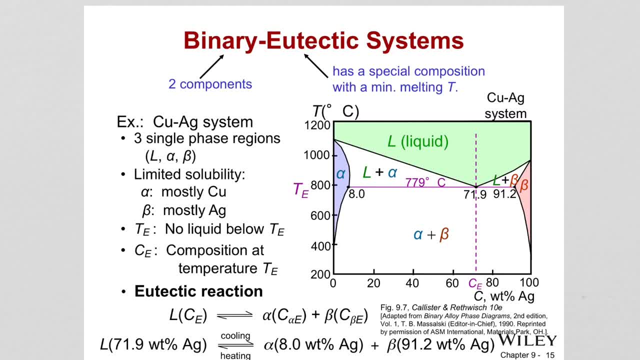 So in this case we are seeing a copper and silver And if we look at the phase diagram again, as a function of temperature and composition of silver, different types of phases are available. We see alpha, liquid, beta, And in some regions, for example here, only alpha is stable. 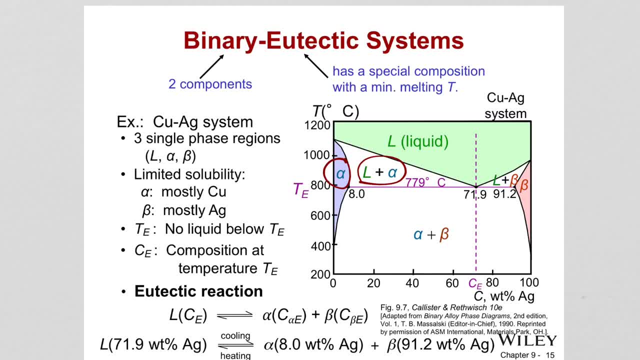 In these regions, for example, liquid and alpha together, stable In here liquid stable beta, Liquid beta And alpha and beta. So, again, depending on the temperature and composition, you can read the phase diagram and see which phase is present in that circumstances. 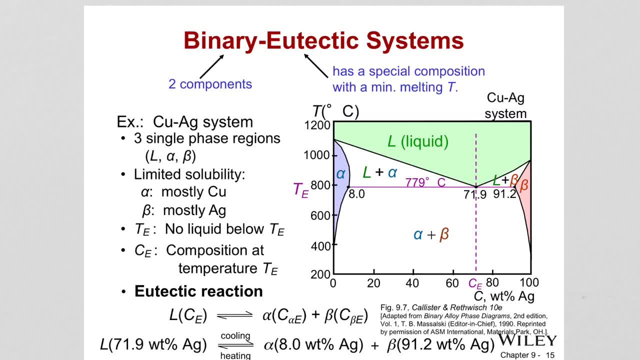 So now alpha has a limited silver solubility. We are seeing that If we look at the maximum solubility of Silver in alpha is around 8. So 8% silver maximum solubility in this structure. 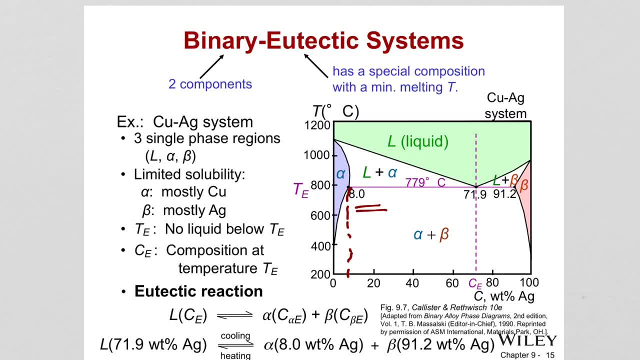 So what about beta? Beta means, if you are looking here, maximum solubility of silver is actually very high, So it can solve up to 95 or so. So that means like 5% copper is soluble inside beta. 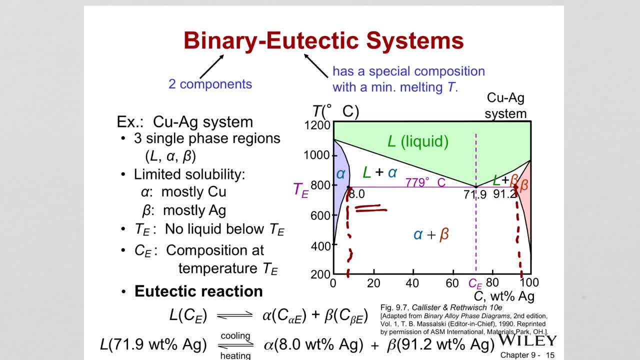 Okay, so these are the solubility limits- maximum element that we can dissolve in that system- And we are seeing something. So in 0% silver, that means we have 100% copper And its melting point is: 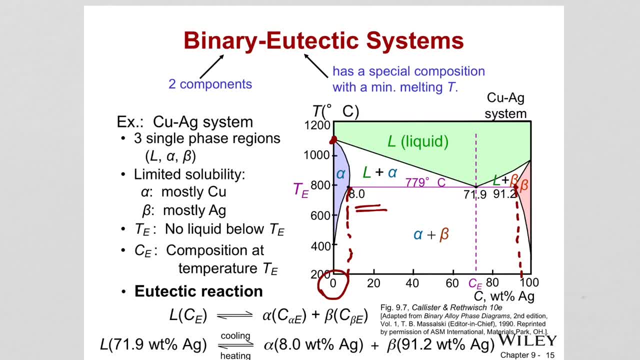 Right there, I mean for pure copper And for pure silver. the melting point is there. So when you have a eutectic system, these, When they are put together, silver and copper, they will have a low minimum melting point at a special composition. 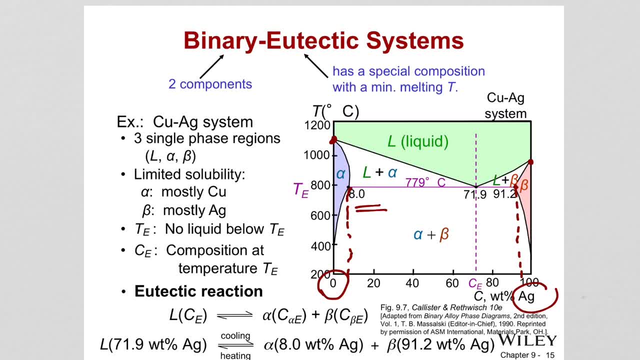 And that special composition you can see Because the melting point is when you go from liquid to solid phases. So in that position, in that composition, which is the eutectic composition, with the symbol E, it was shown subscript E. 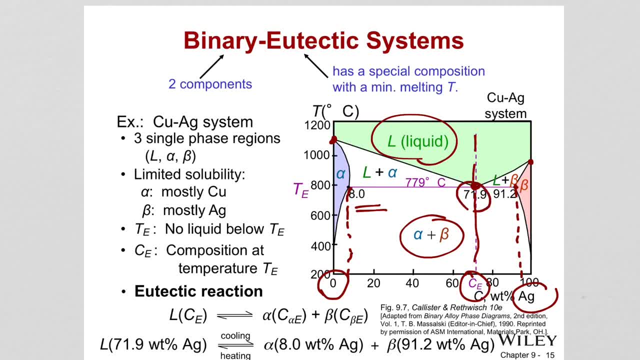 This composition- 71.9, is the eutectic composition, And it is. This material is reaching a minimum melting point, which is- you read it from here- approximately 779 degrees C, So Te is therefore the liquid. 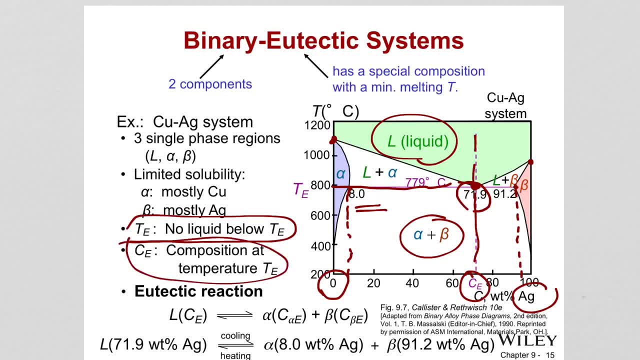 The eutectic, The eutectic temperature. CE is the eutectic composition. Okay, So eutectic reaction is done. We are going from liquid, which is at the composition of CE, And we are going to two solid phases, alpha and beta, when we cool it down. 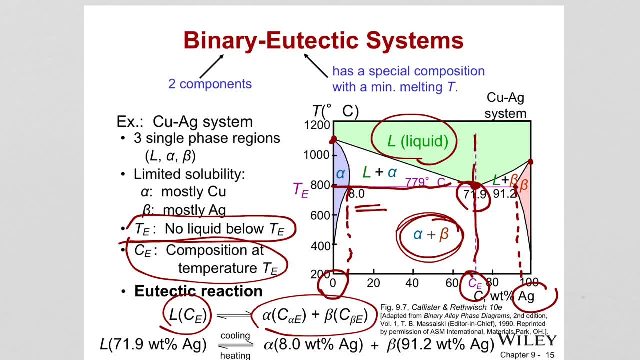 So alpha and beta compositions is Going to be red like this: Let me show you Erase And we choose some color. Okay, So in this composition you go to draw your tie line And then go here and read 8% as the alpha composition. 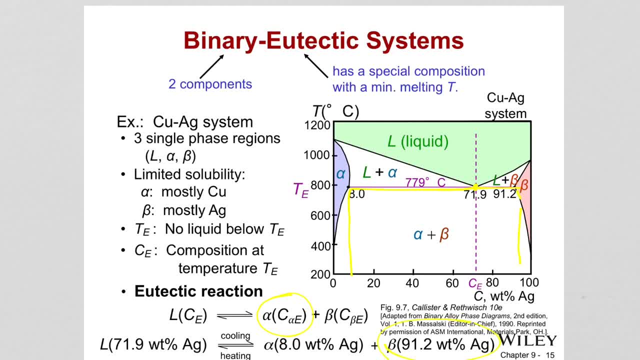 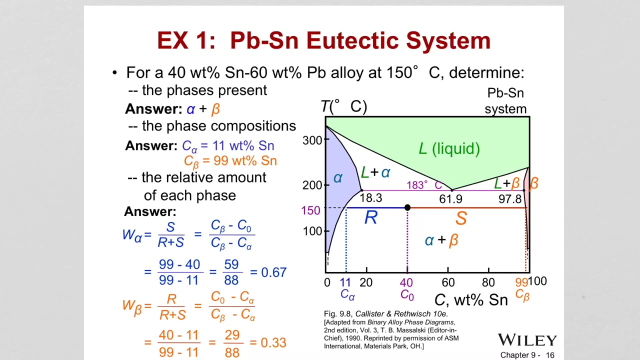 And 91.2% for the silver composition, So this intersection is 91.2.. Okay, That's it, But the The liquid composition was this one, which is 71.9.. Okay, So the question is coming. 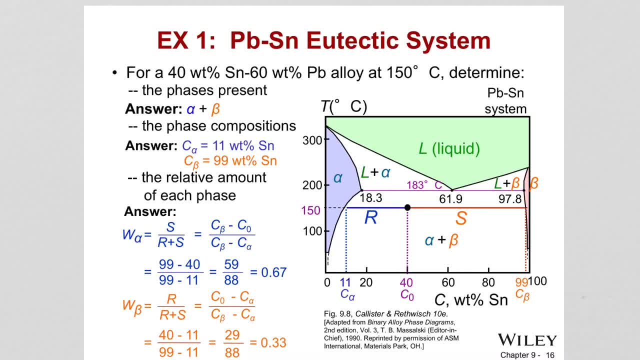 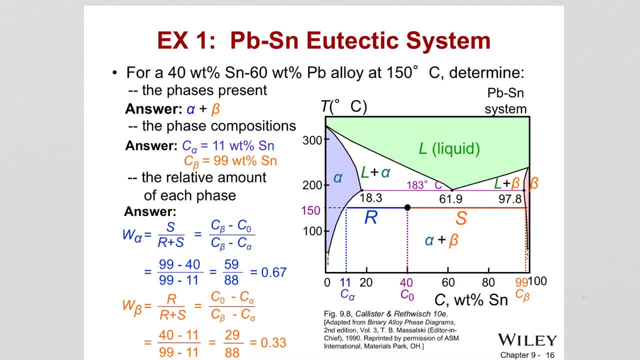 So this is the eutectic. So this is the eutectic. Of course, that means 60% lead, automatically Right, And which is at a composition of 150 degrees C. So now, if you want to determine in your phase diagram, tin and lead phase diagram, 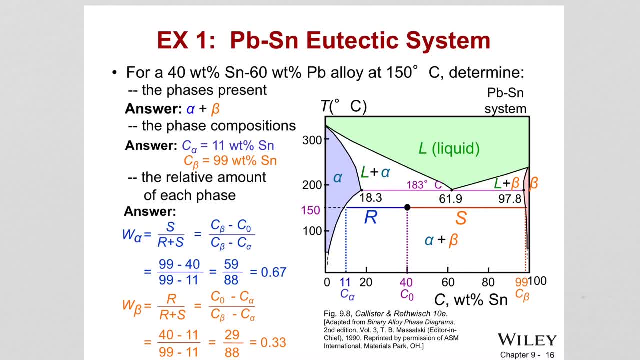 you need to be careful what is given to you on the X axis, Because in this case, X axis is showing us weight percent of tin. So therefore, Okay, Okay, Okay, Okay, so we have. so we are given: yeah, we need to look at the x-axis and then here you have tin right And 40% tin. then you need to look at the concentration of the tin to be able to read the x-axis, okay. 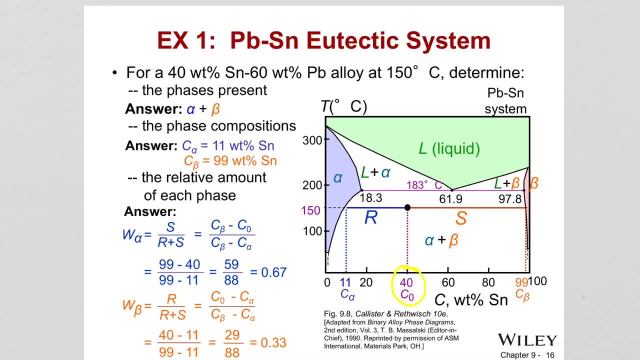 So this is your original composition and the temperature given to us is 150, so we look at the intersection and we find that we are located in a region where alpha and beta solid phases are in equilibrium. Alright, so that means I have both alpha and both beta in the system, And what are their compositions? What are their compositions? It's easy. you look at the tie line. 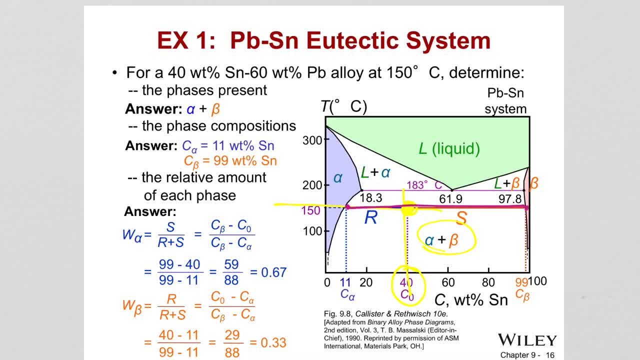 temperature line, you start from here to here and look at its interaction between the phases. so if you look at the intersection of this tie line with this line, it should give you the composition of alpha. and if you look at the intersection of this tie line with the beta phase, it should give you the beta. 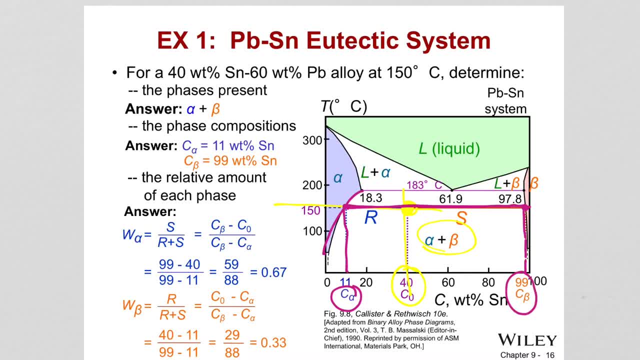 phase composition. so in alpha phase you have 11% tin in of course, the remaining is the lead. in beta you have 99% tin, which is 1% lead. so now we know that. what about how much alpha and how much beta I have in overall alloy? this is the 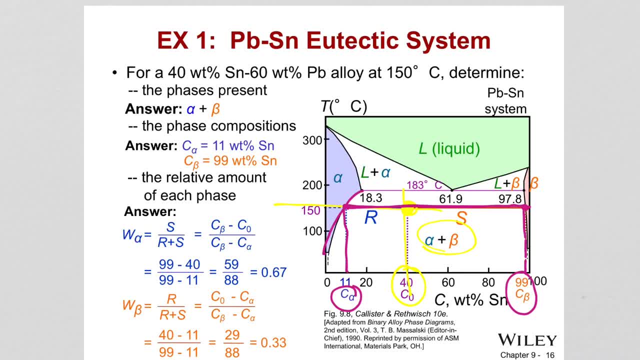 weight fractions of alpha and beta. right? so in order to do that, we're going to use our equation. so, in order to do that, we're going to use our equation. so, in order to do that, we're going to use our equation. so our equations was like that. so all we. 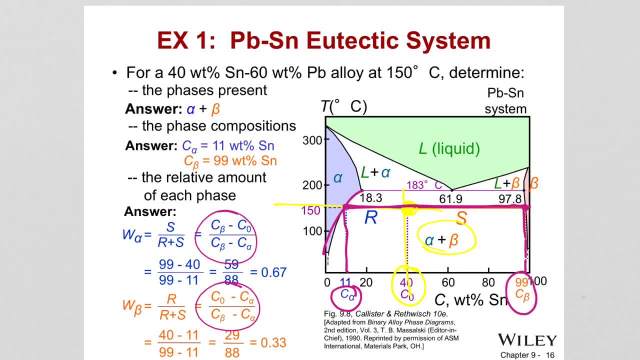 so our equations was like that, so all we so our equations was like that. so all we have to do is put plug in. the have to do is put plug in the have to do is put plug in the information right. so this is 99 minus 40. 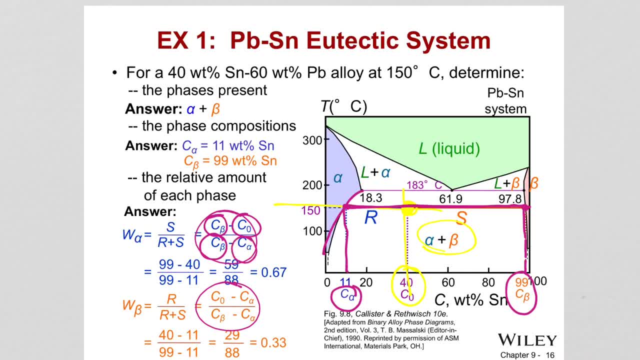 information right. so this is 99 minus 40. information right. so this is 99 minus 40. this is 99 minus 11, and you get 0.67. this is 99 minus 11 and you get 0.67. this is 99 minus 11 and you get 0.67 percent and 67 percent or 0.67 weight. 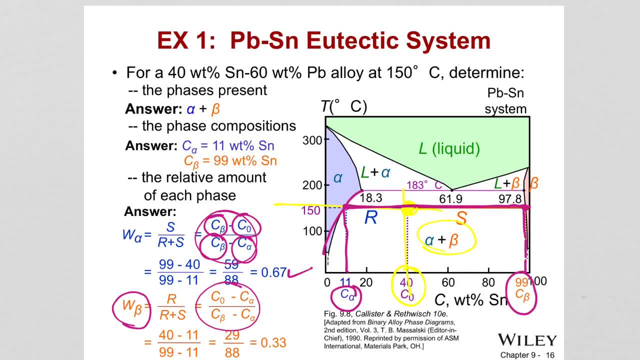 percent and 67 percent or 0.67, weight percent and 67 percent or 0.67 weight fraction. so what about the weight fraction? so what about the weight fraction? so what about the weight fraction of beta? the remaining should be. fraction of beta, the remaining should be. 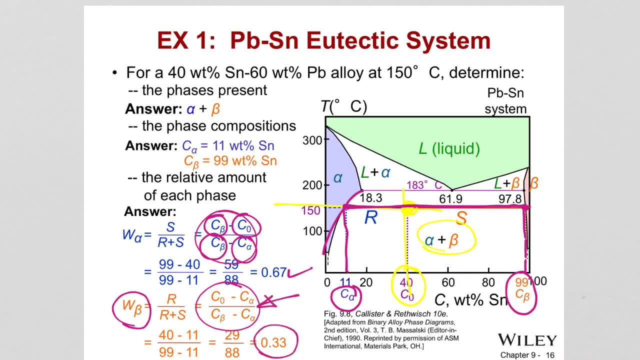 fraction of beta. the remaining should be. but you can calculate it again from this. but you can calculate it again from this. but you can calculate it again from this equation. so this is a typical phase equation. so this is a typical phase equation. so this is a typical phase diagram. question that can come in the. 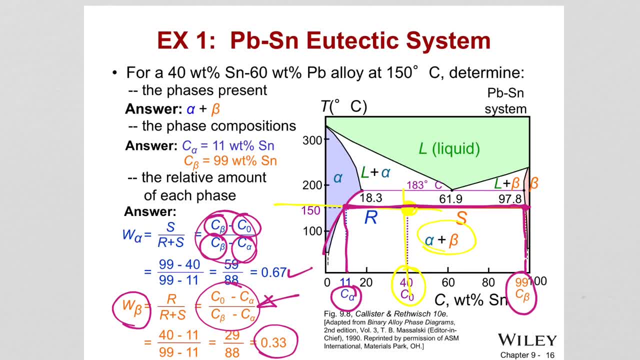 diagram: question that can come in the diagram. question that can come in the exam. a lot of questions can be asked, so exam. a lot of questions can be asked, so exam. a lot of questions can be asked, so you guys need to learn how to read the. you guys need to learn how to read the. 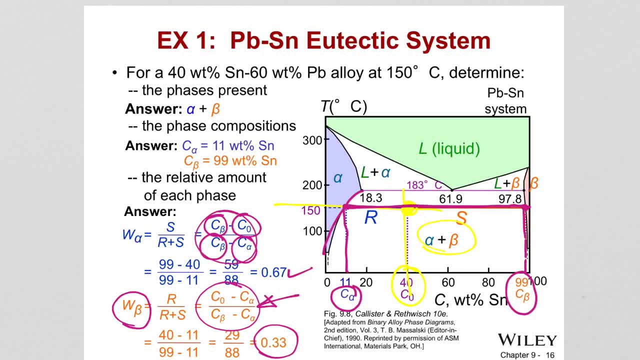 you guys need to learn how to read the phase diagram and if you're having phase diagram and if you're having phase diagram and if you're having difficulty after the lecture, please come. difficulty after the lecture. please come difficulty after the lecture. please come and ask questions to me. come means text. 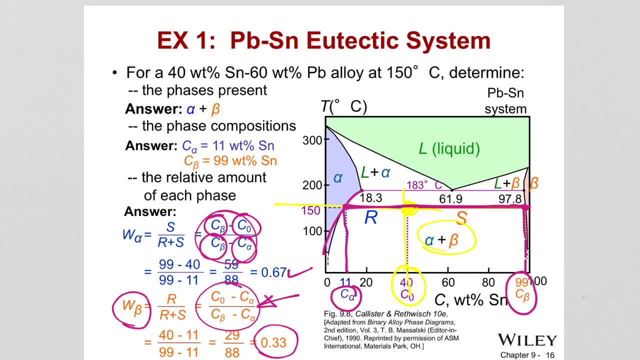 and ask questions to me. come means text and ask questions to me. come means text me. of course. unfortunately, that's the me, of course. unfortunately, that's the me, of course. unfortunately, that's the reality here. so you guys gonna text me- reality here. so you guys gonna text me. 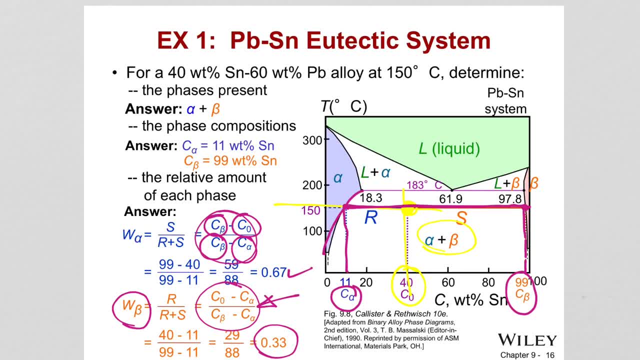 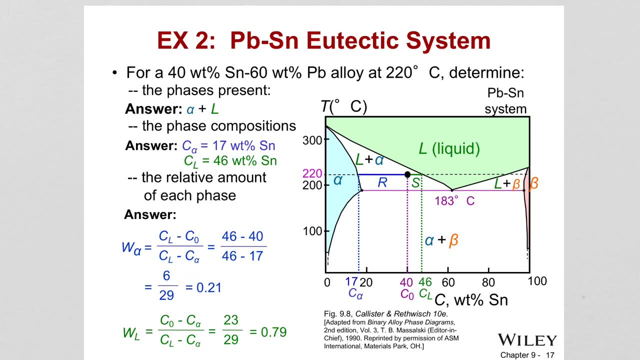 reality here. so you guys gonna text me or come to office hours and ask, or come to office hours and ask, or come to office hours and ask questions to TAS and try to learn about questions to TAS, and try to learn about questions to TAS and try to learn about it, okay, okay. so another example: here we 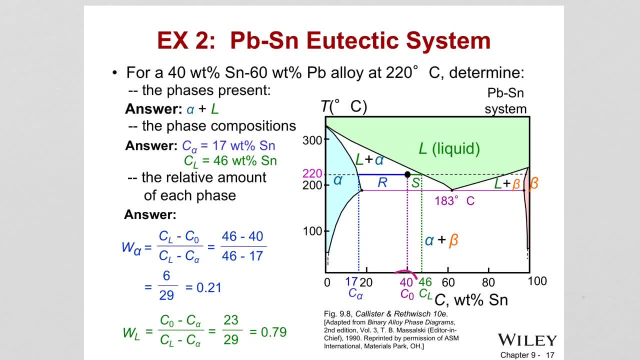 it okay, okay. so another example: here we it okay, okay. so another example here. we have still 40%- 10 alloys. so our again have still 40%- 10 alloys. so our again have still 40%- 10 alloys. so our again original composition is 40% this time. 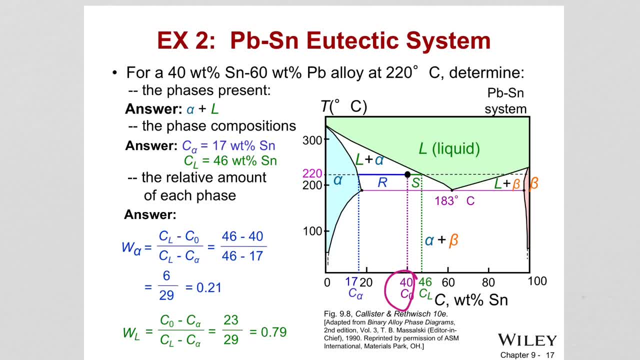 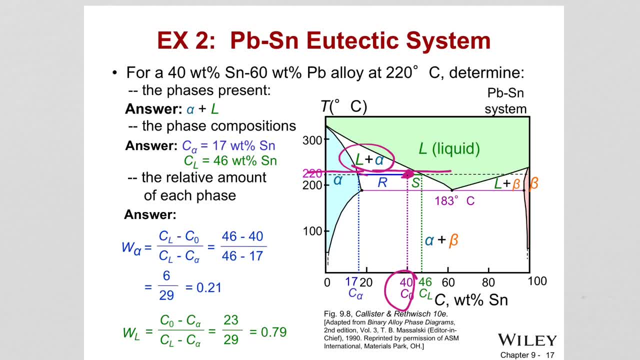 means I have liquid and alpha in, means I have liquid and alpha in equilibrium. so what is the composition of equilibrium? so what is the composition of equilibrium? so what is the composition of liquid and what is the composition of liquid? and what is the composition of liquid and what is the composition of alpha? again we look at the intersection. 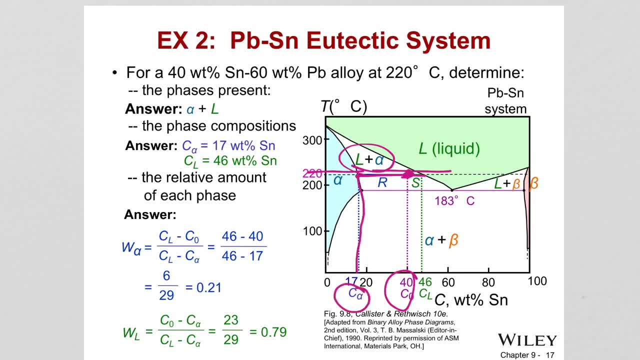 alpha again. we look at the intersection alpha again. we look at the intersection of the tie line and reads alpha of the tie line and reads alpha of the tie line and reads alpha composition here and read liquid composition here and read liquid composition here and read liquid composition here and it is 70%, 10 in. 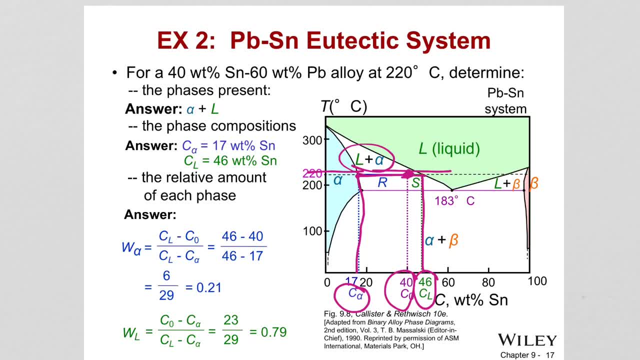 composition here, and it is 70%. 10 in composition here and it is 70%. 10 in alpha 46 percent- 10 in and liquid alpha 46 percent- 10 in and liquid alpha 46 percent- 10 in and liquid liquid. from that again you can calculate the 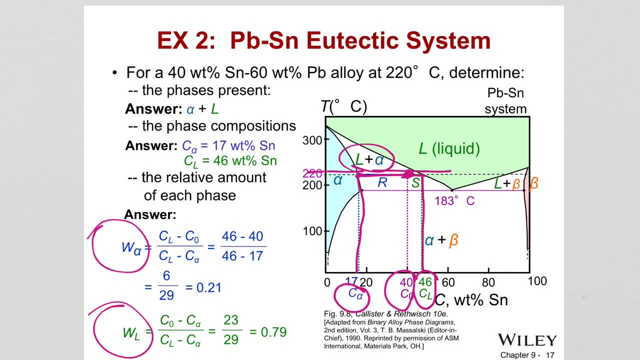 liquid. from that again you can calculate the liquid. from that again you can calculate the weight fractions of the solid and weight fractions of the solid and weight fractions of the solid and liquid phase also. so how much alpha we liquid phase also. so how much alpha we liquid phase also. so how much alpha we have 0.21. how much liquid we have 0.7, 9. 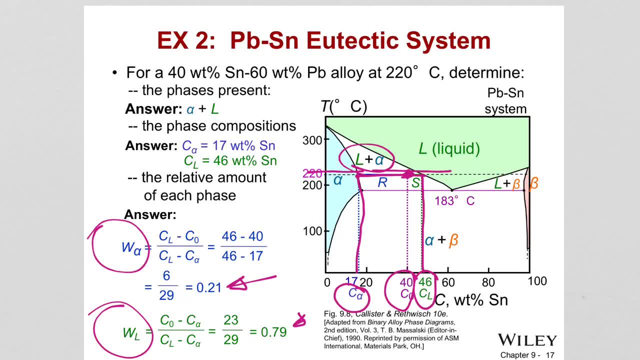 have 0.21. how much liquid we have 0.7. 9 have 0.21. how much liquid: we have: 0.7: 9. so 21% alpha, the rest is basically 79. so 21% alpha, the rest is basically 79. 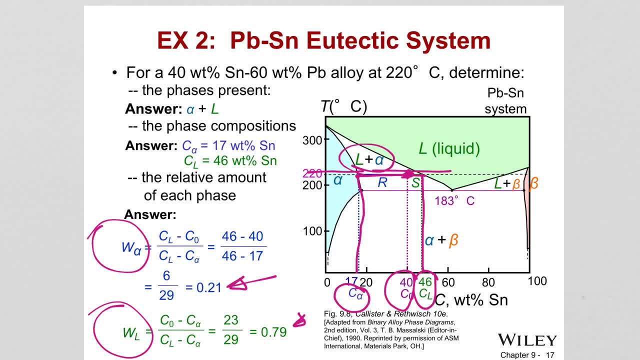 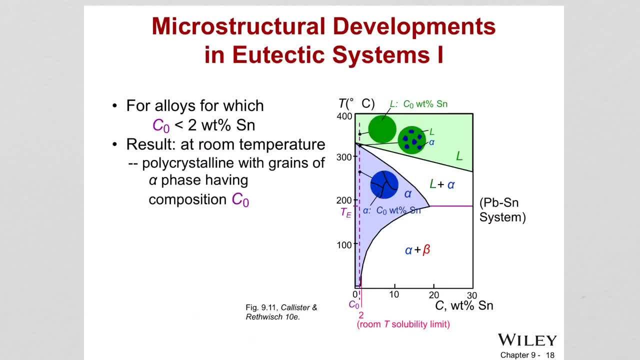 so 21% alpha. the rest is basically 79 percent beta and within this alpha the percent beta and within this alpha the percent beta and within this alpha the composition of it: 17 percent 10. composition of it: 17 percent 10. composition of it: 17 percent 10. okay, in in this system again, tin and lead. 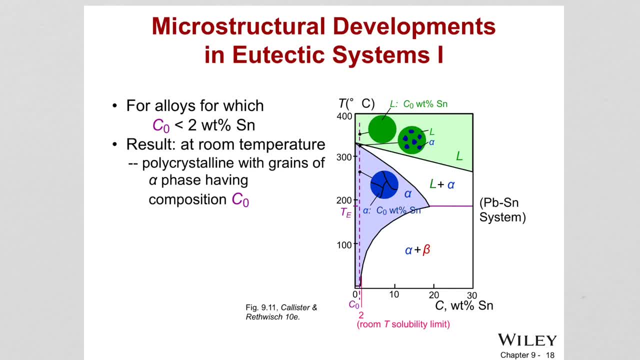 okay, in in this system- again tin and lead. okay, in in this system- again- tin and lead system. we are seeing a part of the system. we are seeing a part of the system. we are seeing a part of the phase diagram. up to 30% of tin, if let's. 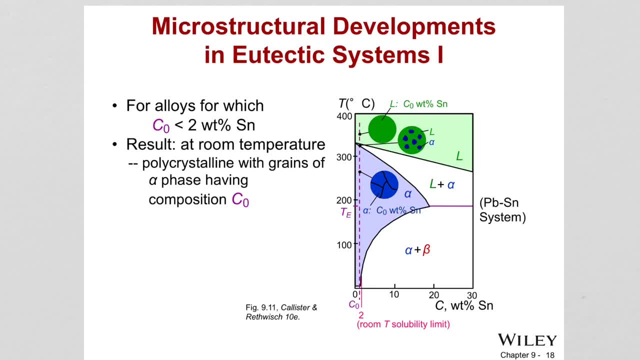 phase diagram up to 30% of tin. if let's phase diagram up to 30% of tin, if let's say you have an alloy, which is the say you have an alloy, which is the say you have an alloy which is the composition is less than 2 great percent. 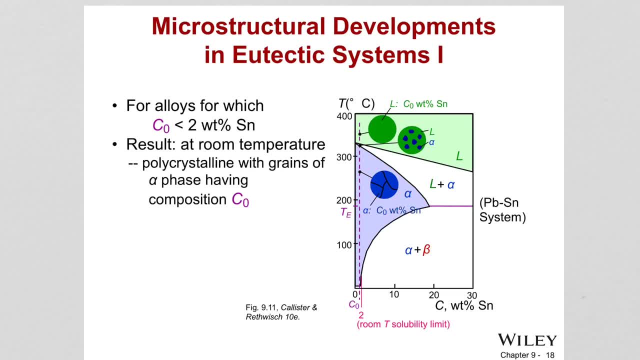 composition is less than 2 great percent. composition is less than 2 great percent tin. it is shown with the purple line C tin. it is shown with the purple line C tin. it is shown with the purple line C not. and if we want to analyze a new 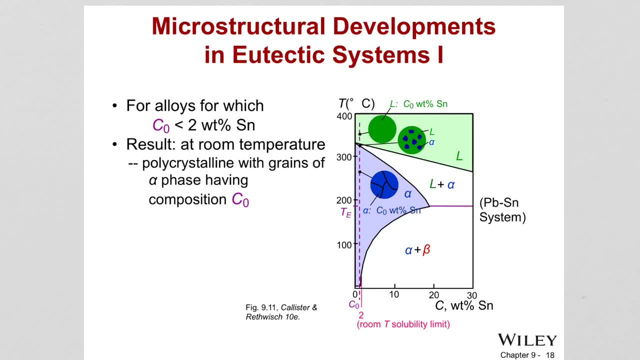 not. and if we want to analyze a new, not, and if we want to analyze a new, tactic systems, how the microstructure is tactic systems, how the microstructure is tactic systems, how the microstructure is changing at this point, right there we changing at this point, right there we. 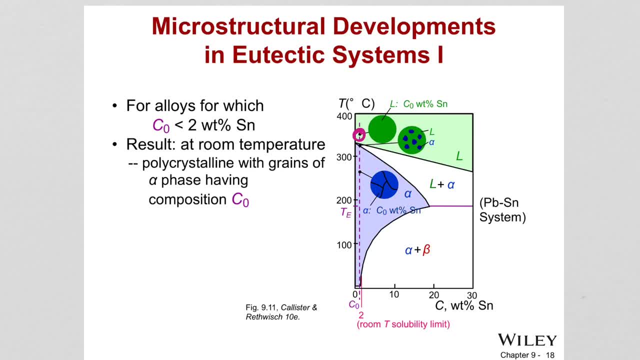 changing at this point. right there we are, only have liquid and as we cool it are, only have liquid. and as we cool it are, only have liquid. and as we cool it down, we come to liquid and solid phase down. we come to liquid and solid phase down. we come to liquid and solid phase here. so both of them are in the 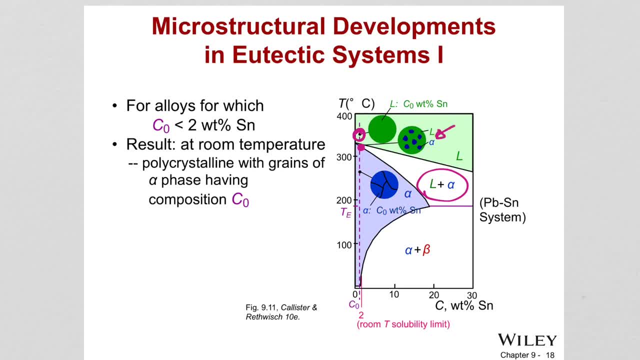 here. so both of them are in the here. so both of them are in the equilibrium. so the alpha solid is forming equilibrium. so the alpha solid is forming equilibrium. so the alpha solid is forming from the liquid green and then, as we, from the liquid green and then, as we. 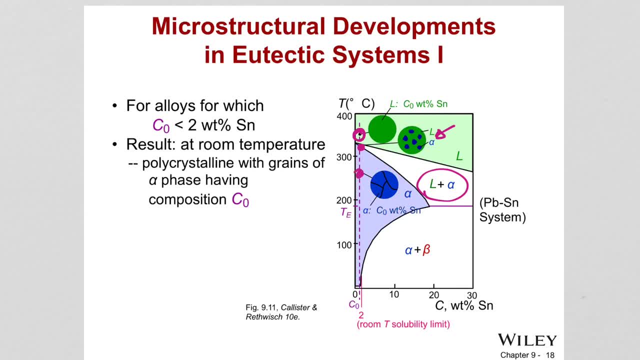 from the liquid green and then, as we keep lowering it down at this point, we keep lowering it down at this point, we keep lowering it down at this point- we can see how the green boundaries are, can see how the green boundaries are, can see how the green boundaries are forming in this pure solid phase. so we 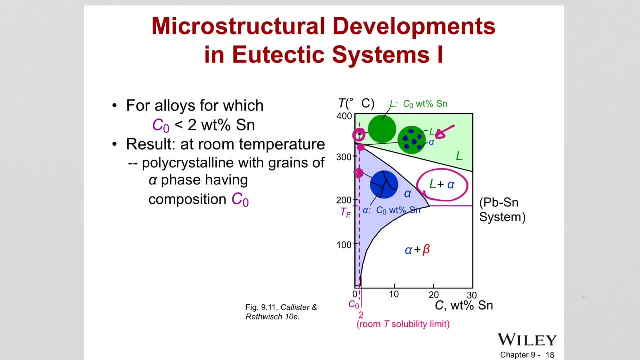 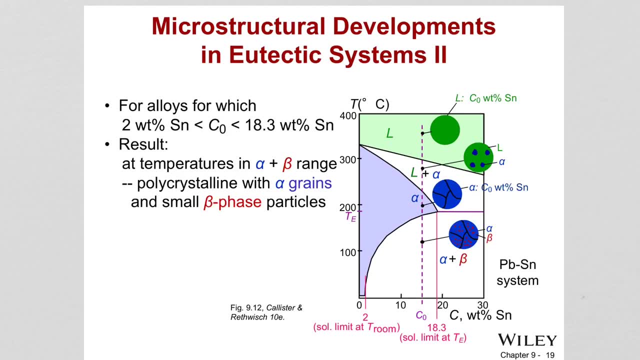 forming in this pure solid phase. so we forming in this pure solid phase, so we can see all of them have a composition, can see all of them have a composition, can see all of them have a composition of C, not of C, not of C, not, let's say, you have an alloy and the 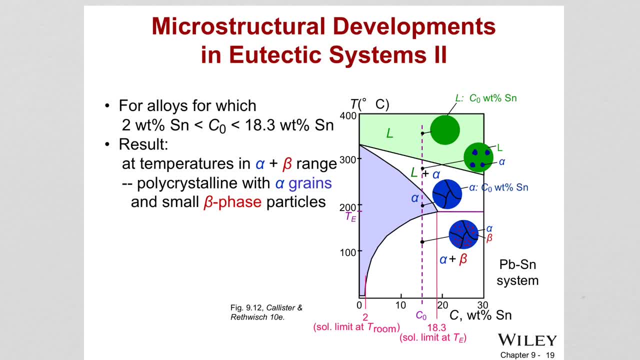 let's say you have an alloy and the. let's say you have an alloy and the concentration of the alloy, the initial concentration of the alloy, the initial concentration of the alloy, the initial composition of the alloy is in between 2. composition of the alloy is in between 2. 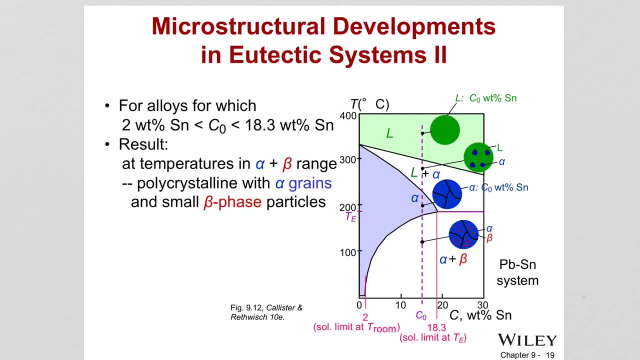 composition of the alloy is in between 2 percent and percent and percent and 18 to 18 point 3 percent, so somewhere 18 to 18 point 3 percent, so somewhere 18 to 18 point 3 percent, so somewhere here. if this is our original composition. 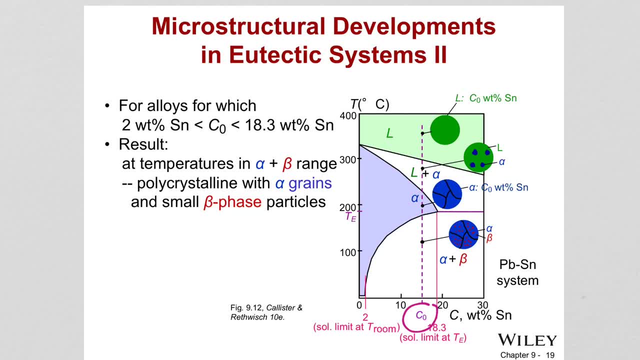 here, if this is our original composition here, if this is our original composition, so let's analyze the micro structural. so let's analyze the micro structural. so let's analyze the micro structural, micro structural developments. okay. so we micro structural developments. okay, so we micro structural developments. okay, so we start at this point and start cooling. 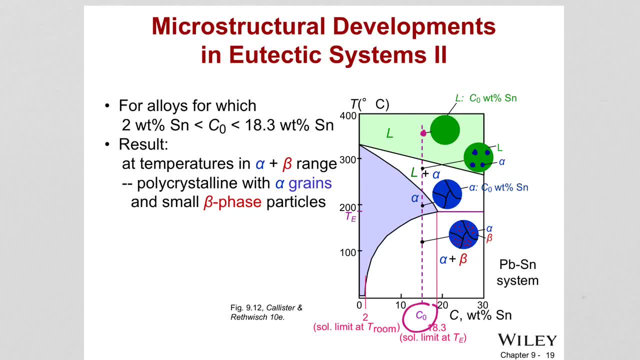 start at this point and start cooling. start at this point and start cooling down again at that point. we just have down again at that point. we just have down again at that point. we just have liquid. that's what we are seeing in the liquid, that's what we are seeing in the 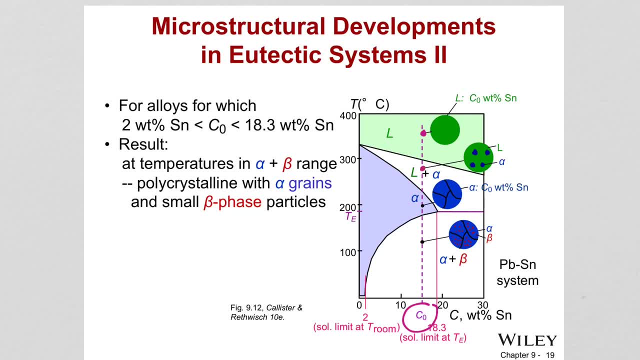 liquid- that's what we are seeing in the microscope- and then we cool it down come microscope, and then we cool it down, come microscope, and then we cool it down. come to this point now we should have liquid. to this point now we should have liquid. to this point now we should have liquid and solid liquid and alpha, and we are. 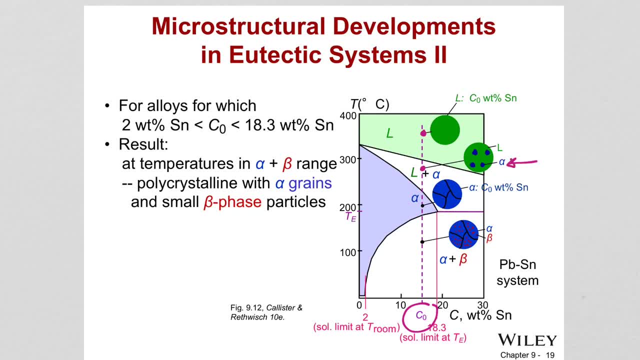 and solid liquid and alpha, and we are and solid liquid and alpha and we are seeing the alpha is starting to form, seeing the alpha is starting to form, seeing the alpha is starting to form inside the liquid, and then, as we keep inside the liquid, and then as we keep, 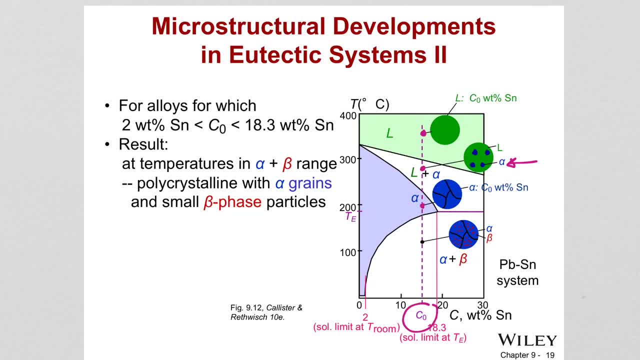 inside the liquid. and then, as we keep cooling down and down and come to this cooling down and down, and come to this cooling down and down and come to this point, we only have alpha. we can see the point: we only have alpha. we can see the point: we only have alpha. we can see the earth's only solid alpha with. 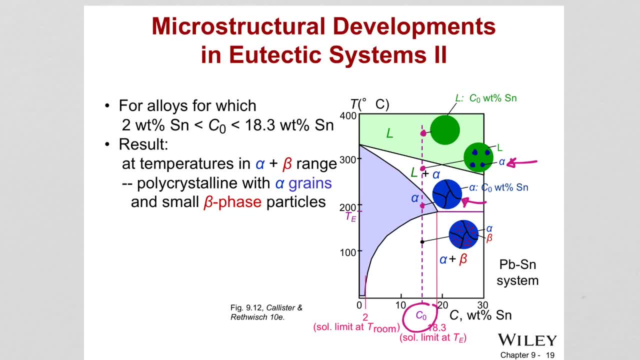 earth's only solid alpha, with earth's only solid alpha, with polycrystalline structure grain, polycrystalline structure grain. polycrystalline structure, grain, boundaries, alpha grains. now as we keep boundaries, alpha grains, now as we keep boundaries, alpha grains, now as we keep lowering, we come to this point, which is: 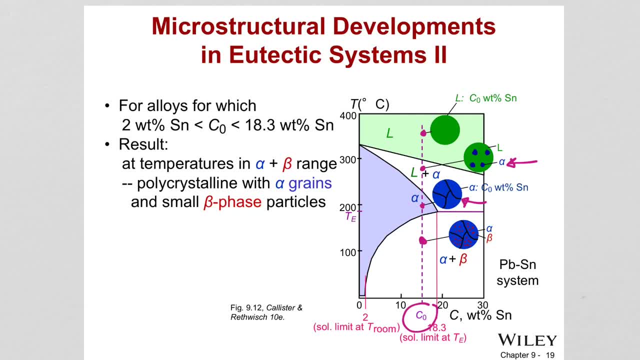 lowering. we come to this point which is lowering. we come to this point which is: from alpha, now beta starts to form. so we, from alpha, now beta starts to form. so we, from alpha, now beta starts to form. so we have both alpha and beta. so, because we 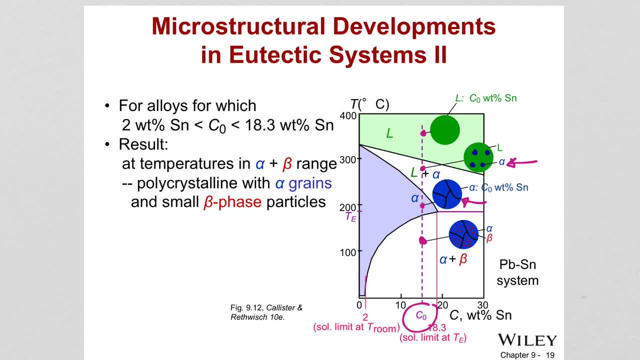 have both alpha and beta. so because we have both alpha and beta, so because we are cooling down, we started with the are cooling down. we started with the are cooling down. we started with the alpha grain structure and from the alpha alpha grain structure and from the alpha. 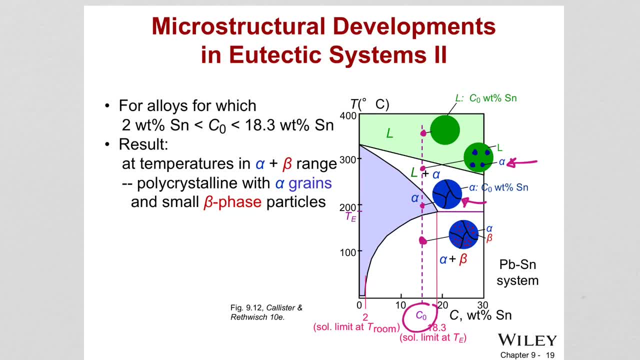 alpha grain structure and from the alpha grain structure, beta grains are forming grain structure. beta grains are forming grain structure. beta grains are forming- which are shown with the red right now, which are shown with the red right now, which are shown with the red right now, to solid phase is in equilibrium. so we 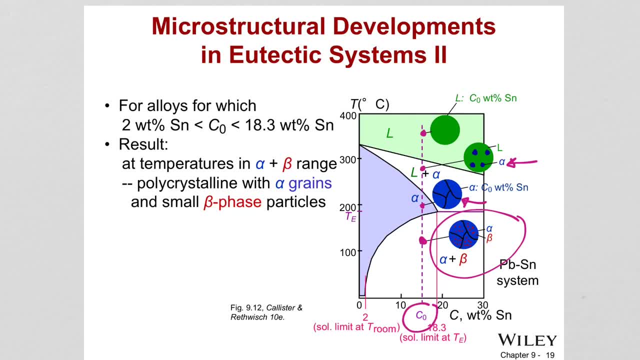 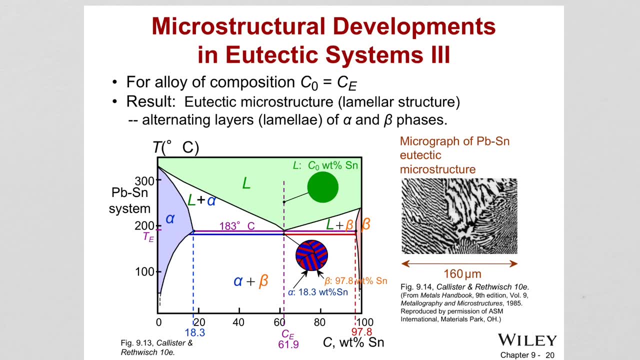 to solid phase is in equilibrium, so we to solid phase is in equilibrium. so we have alpha grains and small beta, have alpha grains and small beta, have alpha grains and small beta. particles in the mic in the structure. particles in the mic in the structure, particles in the mic in the structure. now let's look at if we are at a 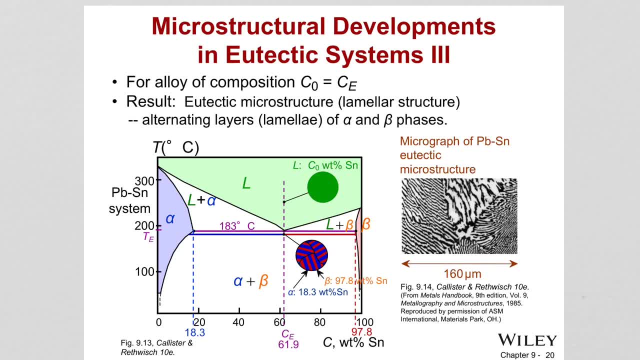 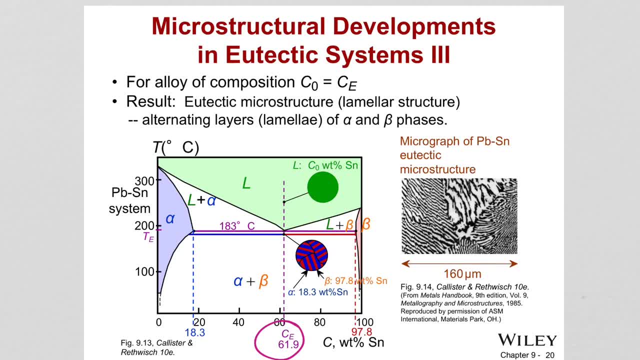 eutectic composition. that means our eutectic composition. that means our original composition is equal to eutectic original composition, is equal to eutectic original composition, is equal to eutectic temperature composition. and we do the same: cooling and analyzing the microstructure. how does it look like? 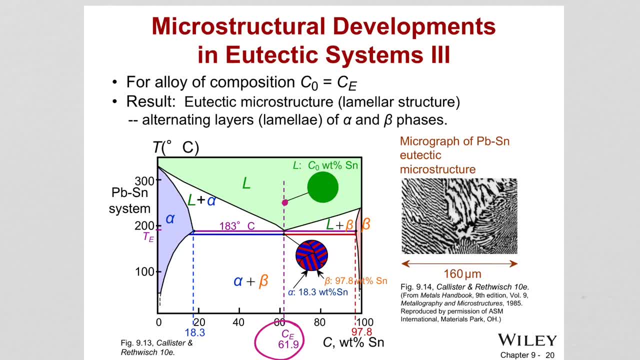 again. we start with the liquid now and from liquid as we cool it down without any other phases. as we pass the eclipsed, it will pass them. you take the temperature and then we go down. what happens from liquid to solid phases are from forming right. so that means you have the mixture of alpha and mixture of. 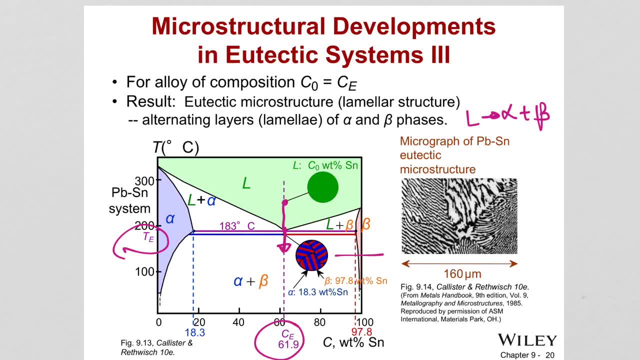 beta and eutectic structure looks like this: a lamellar structure. it is alternating layers of alpha and beta. that is how they are characterized. so in the microscope, when they see, when you see such a structure under microscope, layers of alpha and beta. so whites can be alpha but blacks can be beta. so 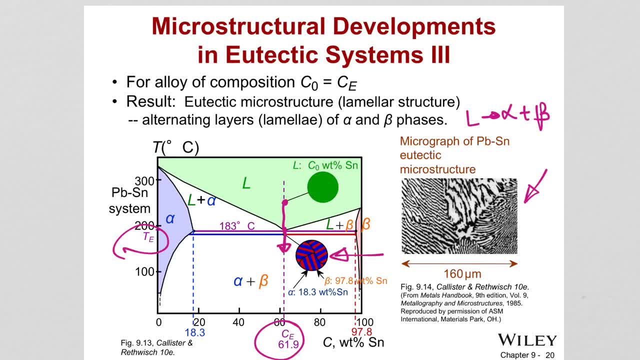 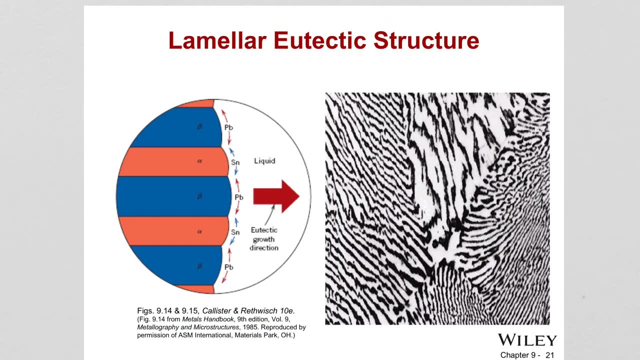 if you see that alternating layers of alpha and beta, that is a characteristics, characteristic property of a eutectic microstructure. so this is just an illustration that how, from the liquid, the solid eutectic structure is forming. okay, so of course the solid particles will start to form within the liquid. and remember, 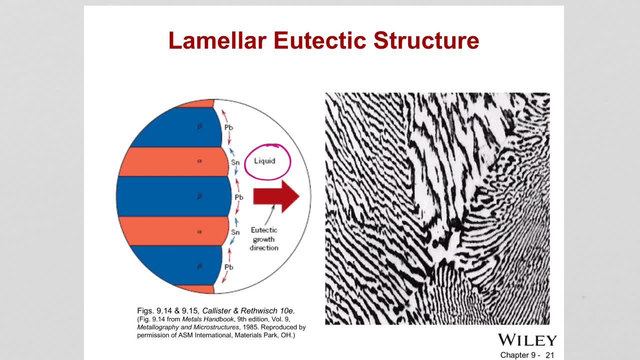 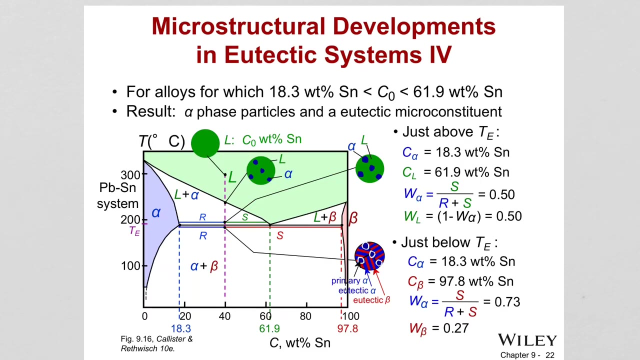 the beta phase is rich in tin, whereas the alpha phase is rich in lead. so what happens? as it grows, tin is flowing to the beta phase and lead is flowing to the alpha phase, and it keeps growing. okay, so let's study this phase diagram eutectic system and let's look at how we 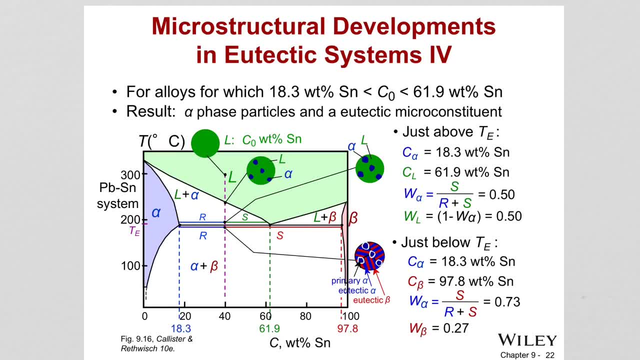 can apply the tie line principle and how we can calculate the weight fraction of each phase. so suppose now you will have an alloy and the composition of alloy is in between 80, 18.3 and 61.9. so our composition is somewhere here. okay, and 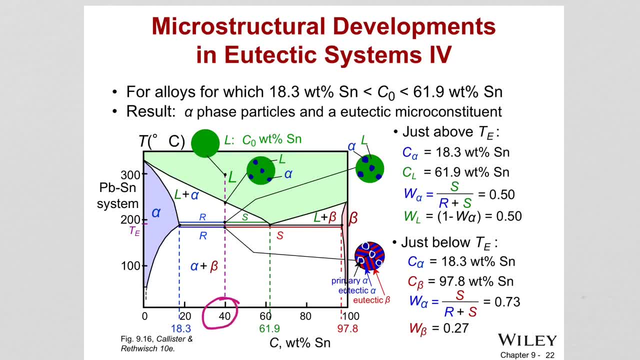 let's look at the liquid phase as we cool it down. let's say we come to this point, just above the eutectic temperature, and we we can see that liquid and alpha is in equilibrium. okay, from liquid alpha, solid is forming. and how you gonna now calculate the composition of alpha and composition of. 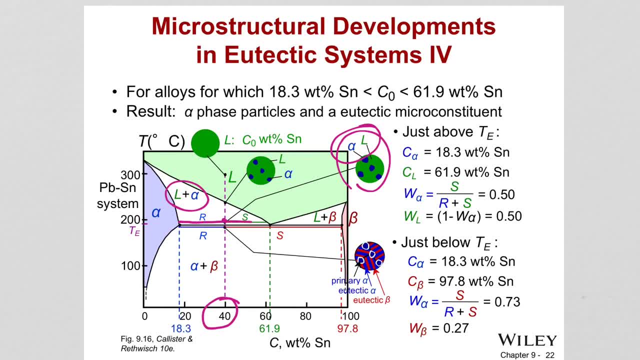 liquid. again the tie line. you go to the intersections and you read that 18.3 percent tin is in the alpha and you read this: 61.9 percent is in the liquid. because you are looking at the interaction of with the liquid line. right, so we figure that out. it's given here. so what you can do, take the 40 as the. 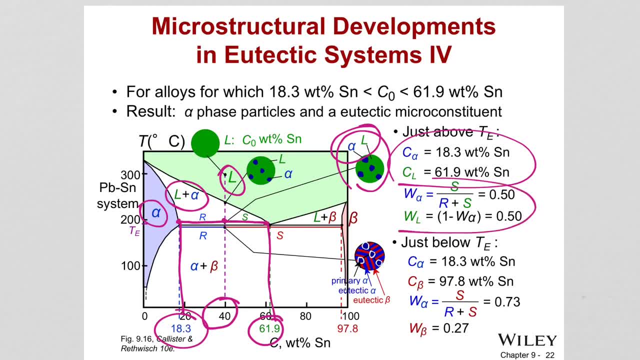 composition: original composition. plug into your equations that we have learned to calculate the weight fractions. it is 50: 50, so that means 50 percent liquid, 50 percent solid and their compositions are given here. so if you go below the eutectic temperature you should have alpha and beta. but 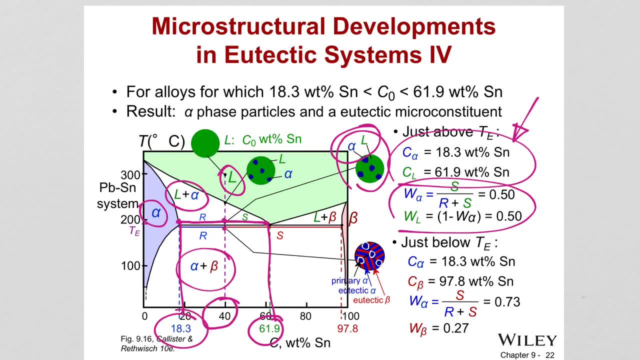 know, remember how the microstructure is gonna look like. so we had this microstructure, right, liquid and Alpha. now, when you go from here to here, basically from the liquid, you need to form alpha and beta because that is the eutectic reaction, right? so you all only already have the alpha particles here. 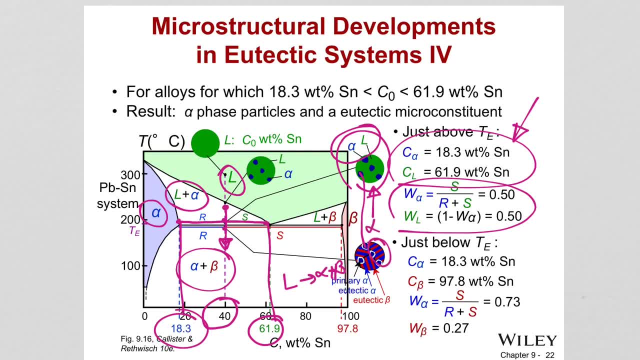 and the remaining liquid will turn to lamellar structure- alpha, Что criminal structure of eutectic stucture- alpha- and layers, alternating layers on the background. okay, so in this case you do the same, you do the same calculation and it's very close. the numbers are very. 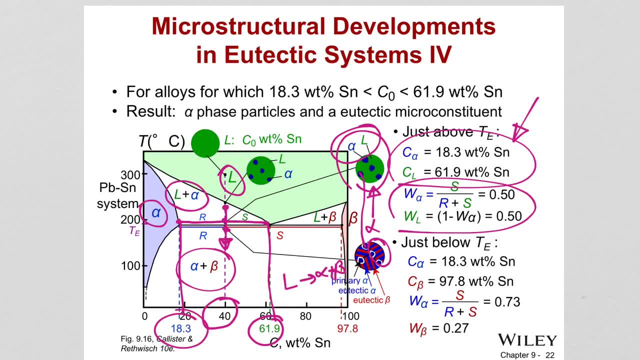 close here. so we have this. we have this point. we read this intersection again: nearly 18.3. and let me get an another pencil here. you read the: go to the beta intersection and read the beta composition and plug those in. you find the weight percentages of alpha and beta. 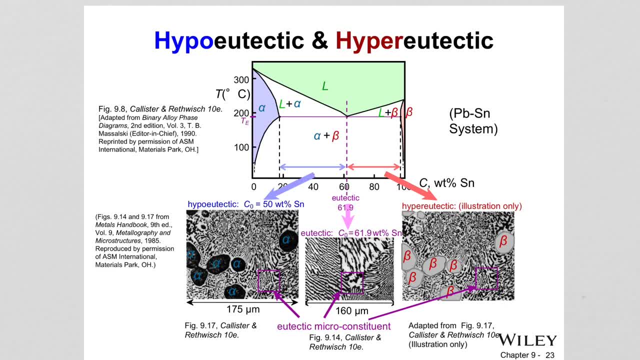 so hypo-eutectic and hyper-eutectic means before the eutectic and after the eutectic composition. so we have seen how it looks like in each of the data, all of these compositions like before eutectic, how it was right if we have a. 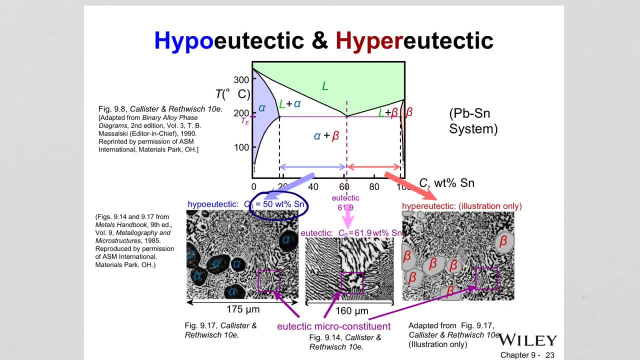 15%, 50% in. then it's gonna look like because we are coming from liquid to alpha, to alpha and beta phase, so the alpha will stay in the structure and liquid will turn into alpha and beta, like we are seeing in the microscopic image. and this is how it look in eutectic. 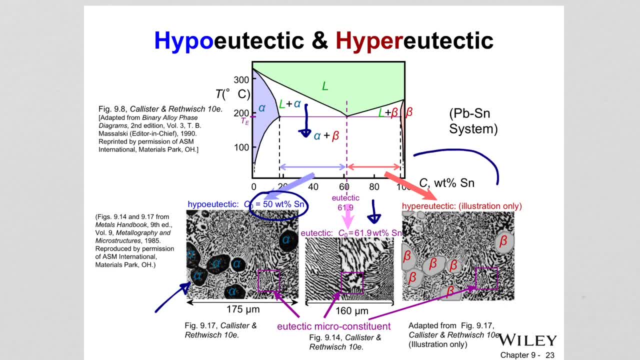 composition and after the eutectoid composition it's called hyper-eutectic. and in this case we start from right. we have beta and liquid and then, when we cool down, liquid turns into alpha and beta. this time beta particles stay and the liquid converted into the eutectic structure. alpha and beta composition. 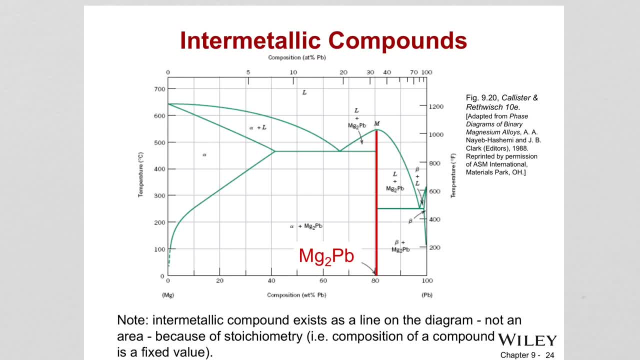 so for some systems there can be compounds forming rather than solid solutions, and these compounds, of course the name compounds mean they have distinct chemical formulas, so certain number of elements will react with certain number of other elements. so these are called intermetallic compounds, as you can. 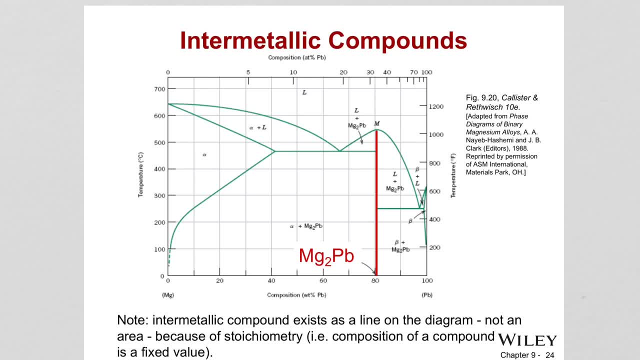 see here lead and magnesium phase diagram. we are seeing a compound which is two magnesium comes together with one lead element, so it is magnesium, two lead. so this is the name of the intermetallic compound. so this is represented in a phase diagram as a vertical line, as you can see. 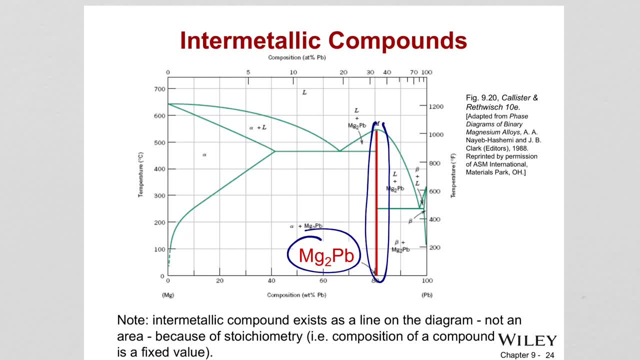 the reason for that, as written here, because of the stoichiometric stoichiometry, because the composition of a compound is a fixed volume. what you can read about this intermetallic compound is its melting temperature, because here we are on this line right and the melting temperature is right there. so 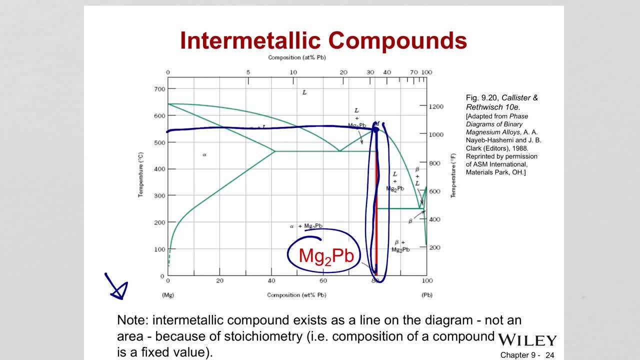 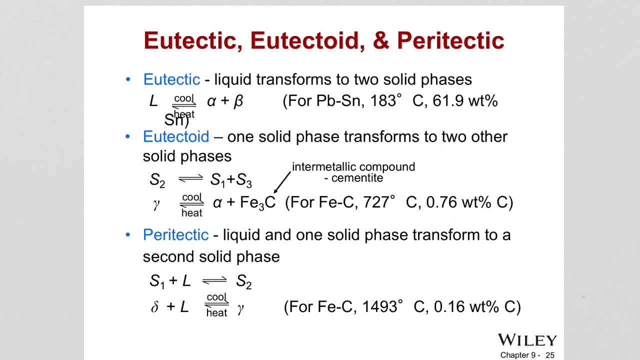 it's approximately 550, as indicated with point M here. other things you might notice: the solubility of lead in magnesium is extensive. this is relatively indicated by the large span of the alpha phase. however, the solubility of magnesium in lead which is shown with the beta is very uh. 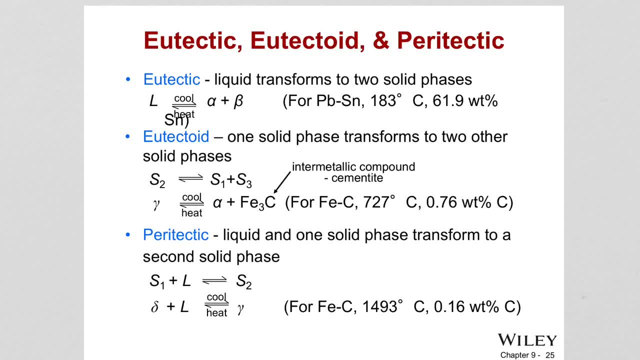 narrow, so it's very limited liquid goes into when it's cooled down, alpha and beta phase. there are also other types of reactions, like eutectoid, peritectic. so when we are talking about eutectoid, one solid phase will go to two solid phase. okay, so here in the eutectic from liquid we go to two solid, in eutectoid from one. 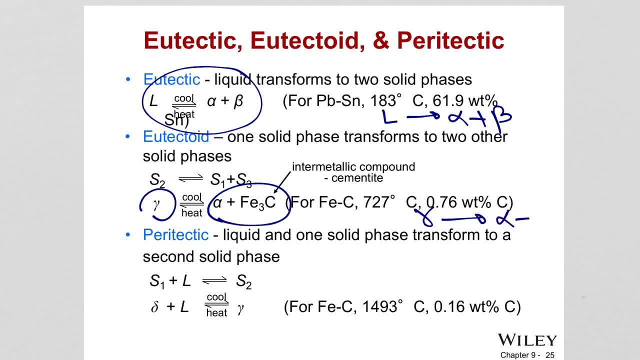 solid gamma, you go down to two solids. the difference is you start with a solid phase here, you start with a liquid phase. okay so, and peritectic is when you have solid phase and liquid phase, for will come together to form a second solid phase. so Delta solid form comes together with liquid and when it's cooled down, forms. 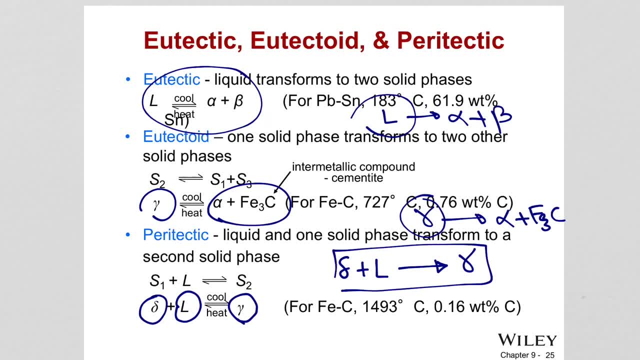 gamma solid phase. that is the peritectic. so here it's also giving you. so S means from solid to solid, from solid liquid combination to one solid. so these are the characteristics of all these reactions and they are giving exact characteristics of all these reactions and they are giving exact. 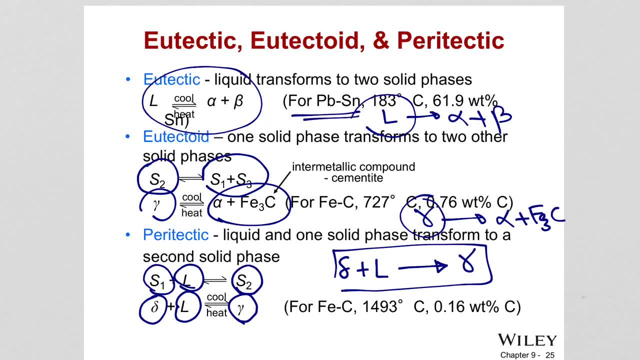 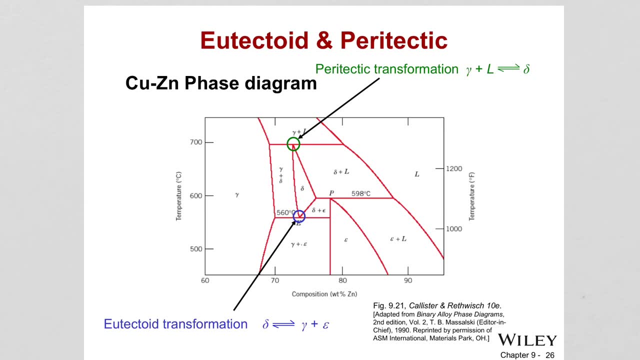 examples from different phase diagrams. we have seen this in thin lead phase diagram. these eutectoid and peritectic reactions exist in iron carbon phase diagram. here we are seeing an example of eutectoid and peritectic reactions. here we have the copper and zinc phase diagram. so it 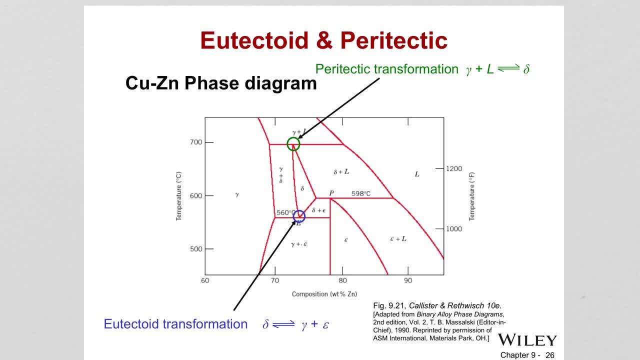 point A we are given it is a eutectoid transformation. upon cooling down from delta, we are going into gamma and epsilon, Meaning from one solid two other solids are formed. What about the peritectic? When we start from this point and cool it down, it goes from gamma plus liquid to delta, So from liquid and 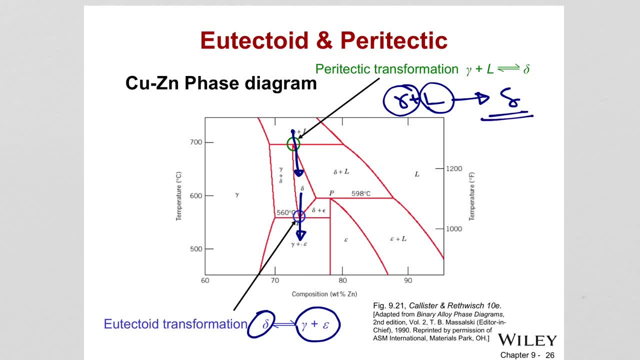 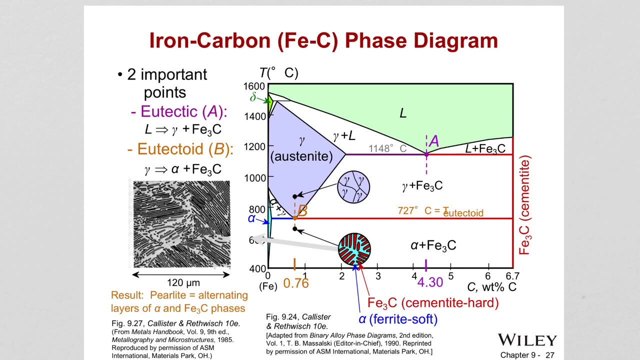 solid combination, you go to form one solid. So you, as you can see, very complex phase diagrams also exists, like in this case we are seeing copper and zinc. So iron carbon phase diagram is the most important phase diagram you ever gonna see, because this phase diagram is used in the production of steel, cast iron and 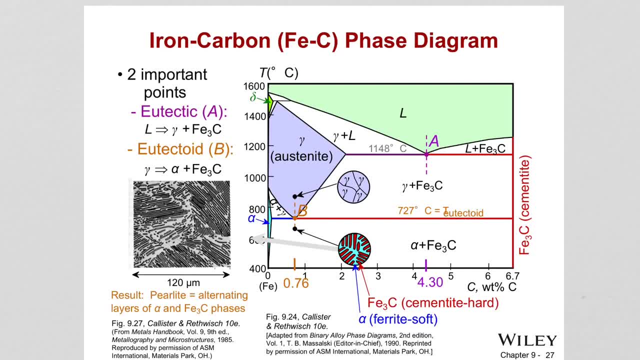 that's why those are the most commonly used materials. therefore, this phase diagram is very important. So it is. as you can see, in the x-axis the carbon range is given, but you see, it's given up to a six point seven percent, Because at six point seven percent what we have is an. 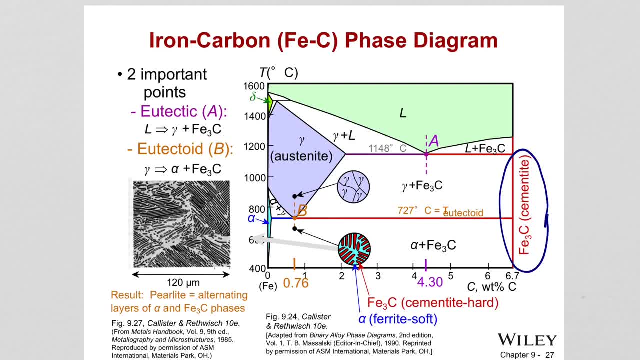 inter-metallic compound called cementite iron three carbon. And this is the only important part of the phase diagram because it gives information about steel manufacturing, steel production, Because the steel, remember, is a combination of an alloy of iron with carbon. So that's why only this region of that phase diagram is actually very important. 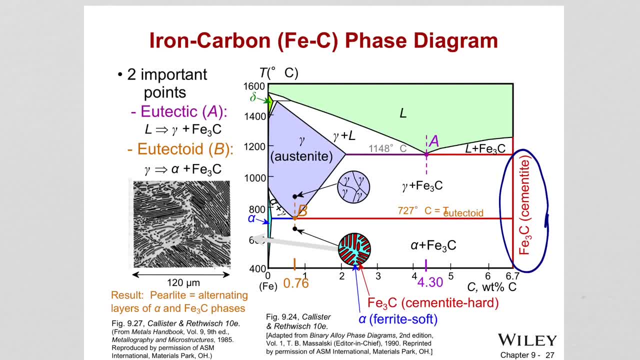 So in the iron carbon phase diagram we are seeing two important points. You see, at point A there is a eutectic reaction because when we cool down from liquid we are going into two solid phase, which is gamma and cementide. So the gamma is called ostonite, as you can see. 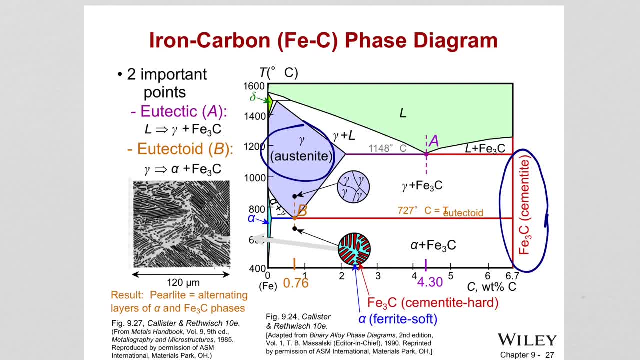 here. So these names are important. Gamma is the ostonite and there is also one eutectoid reaction at point B where we go from ostonite solid to upon cooling, we form alpha solid plus s before the cooling. So it is dangerous for ours, the eutectoid reaction that we see, which also 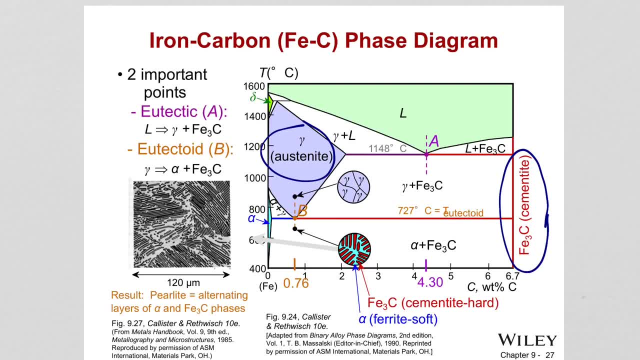 happens. So it is dangerous for ours When we say that the arty working with cuma, that's what we again cementite. so from one solid we form two solid, so it's called eutectoid. so this structure of iron, the structure of alpha plus cementite, is called pearlite. 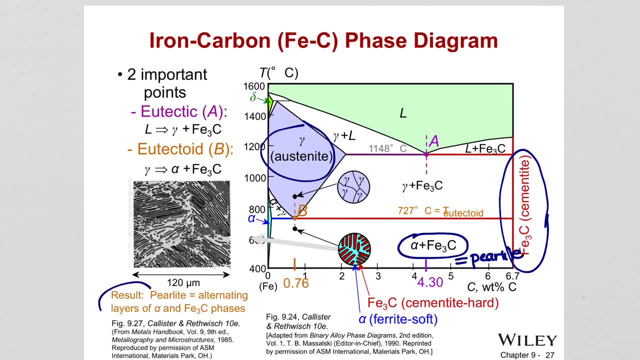 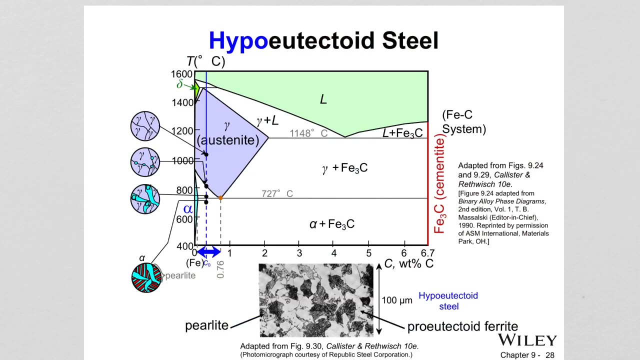 so together they have a name. here you can see pearlite looks like this because we know this is a similar to eutectic structure, right alternating layers of alpha and cementite. this is hypereutectic steel. so before the eutectoid composition. 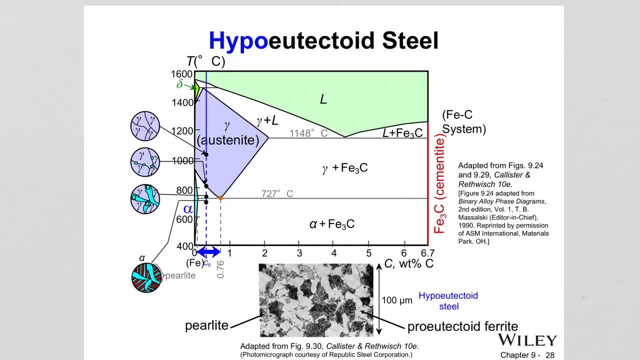 so, as you can see in the iron carbon phase diagram, the eutectoid temperature is 0.76 percent carbon here. this is where the reaction happens, right. we go from gamma to pearlite, which is the combination of alpha iron to cementite, so at this point and below that. so this is where we have the eutectoid still, but now we are. 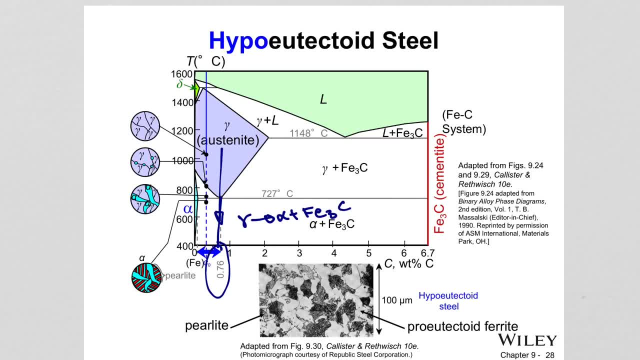 talking about hypereutectate, meaning before the eutectoid composition. that means in between 0 to 0.76, so somewhere in between eutectoid and cementite can choose the composition, which is CNOT. as you can see, let me delete that. 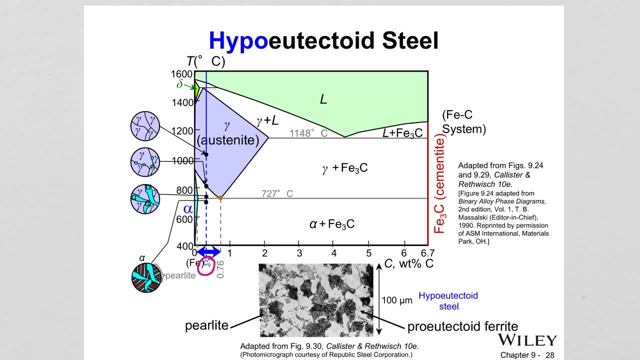 okay, so you can see CNOT at that composition. let's start with an alloy. at this temperature, at this temperature, we have only a gamma, austenite. okay. so it's a alloy of iron and carbon and we are seeing a solid solution of iron and carbon, which is the gamma and called austenite upon cooling down what we are. 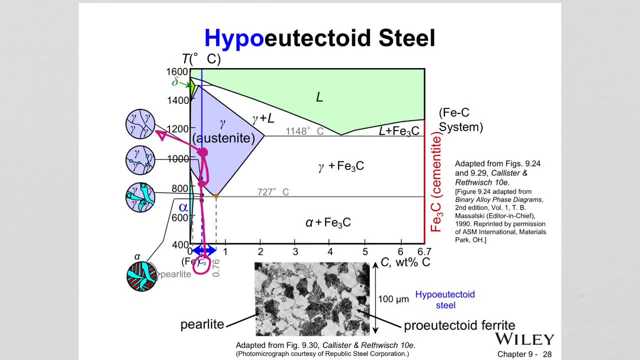 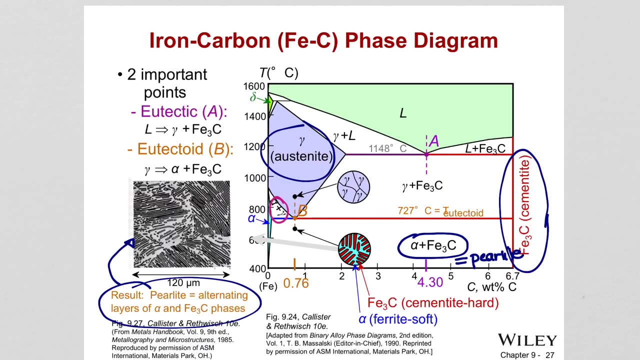 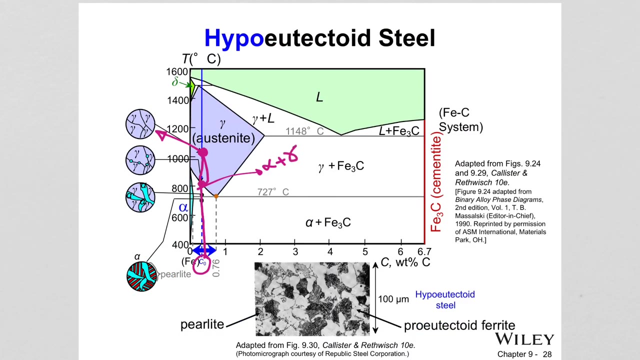 coming here is right there. okay, right there. what do we have here? we have alpha plus. let me see here, here, here, gamma. so from austenite, upon cooling, you need to have the formations of alpha, and i think the alpha is shown here. yes, with the blue. 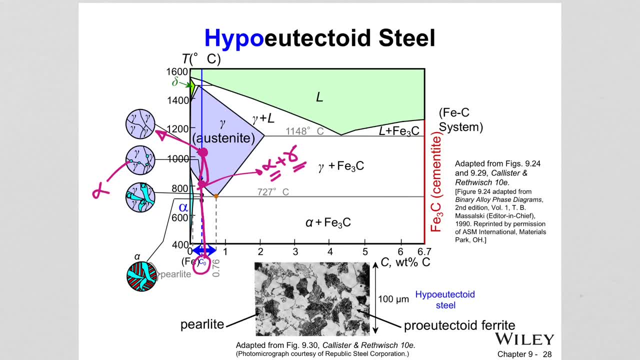 dots. so alpha is starting to form. as you can see, they are forming at the grain boundaries. where are the energetic regions? remember, atoms are more disordered in the grain boundaries. so nucleation of alpha from austenite starts at the green grain boundaries and we continue to cool down. right, we came here. 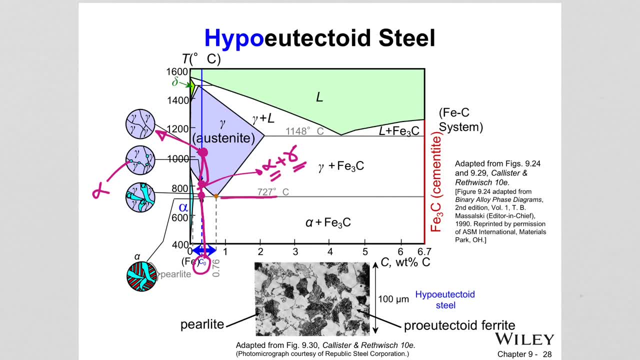 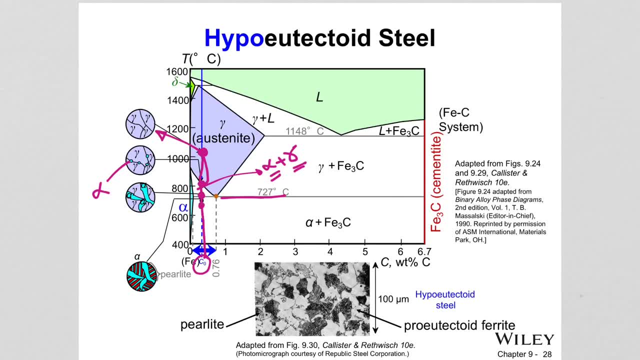 alpha phase. alpha phase grown a little bit. so if we go below the eutectoid temperature right now, from that alpha, from that gamma, so the alpha will stay. okay, as you can see, it stays. but from that gamma you need to form perlite, which is uh, which is the mixture of 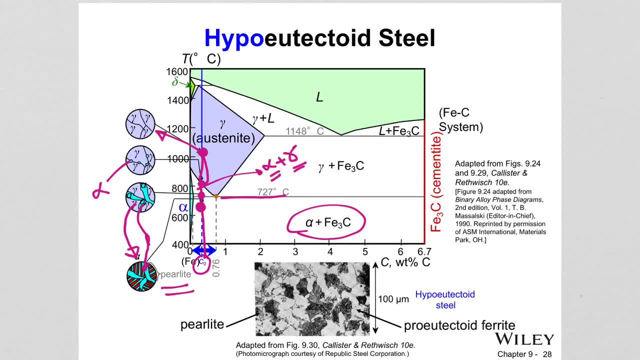 layers of alpha and cementite. this is how it actually looks like, if you can see a hypo eutectoid. still, as you can see, we have pro eutectoid ferrite. ferrite is the name of alpha alpha ferrite, so here the alpha structure is shown with the 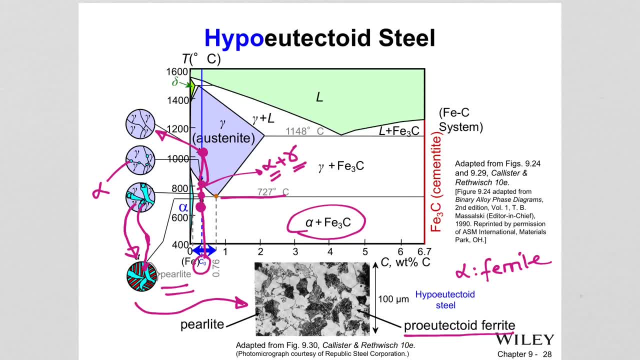 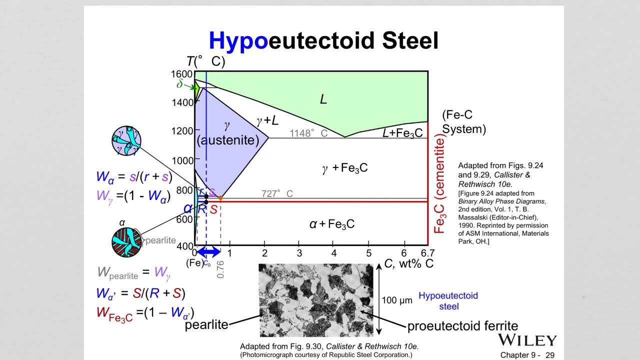 white in under microscope and we are seeing the lamellar structure of perlite right these regions. okay, so in this figure we are given. how do we calculate the weight fractions if we have a hypo eutectoid still, and then if we are above the eutectic you take to take away temperature, if we 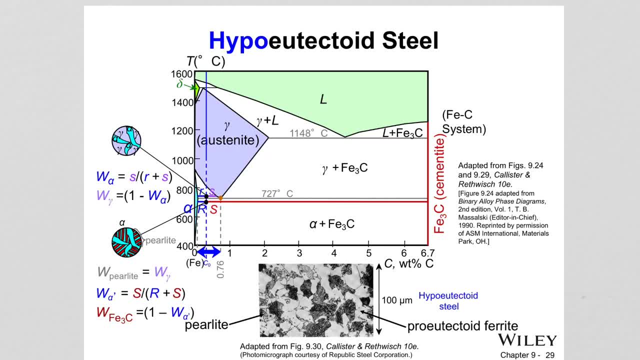 are above, as you can see in this point, right there, right, this is our stabilizer structure and this is the eutectoid temperature. if we are above that, and what is in equilibrium is right, there is alpha plus gamma. so what are the weight fractions of alpha and gamma? 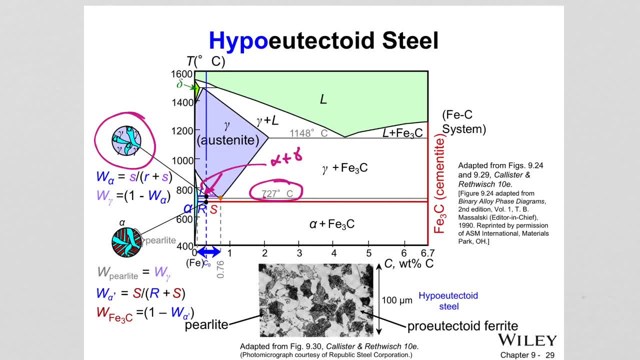 of course you're going to read it the same way. right, there is the tie line here, and then you're going to read the numbers here. okay, and from the equations we have learned, you can calculate it easily. what about if there is the weight fraction below? so we are talking about 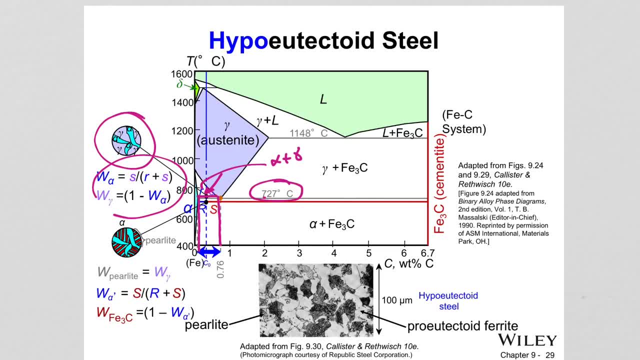 below. let me see: choose a color here so it's visible. let's choose this, okay. no, not this. this, okay. so so let's say you are at this point. that means you have alpha and then pearlite structure. so how do you read the composition? this, what this time? because you 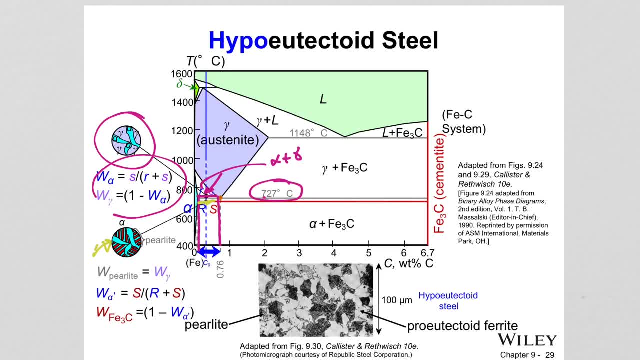 are below the eutectoid temperature. your tie line is going to be this big because there is cementite right. so from here you read alpha composition and from there you read cementite composition. of course, this will give you only the per. the weight fraction of pearlite is actually equal to the weight fraction of 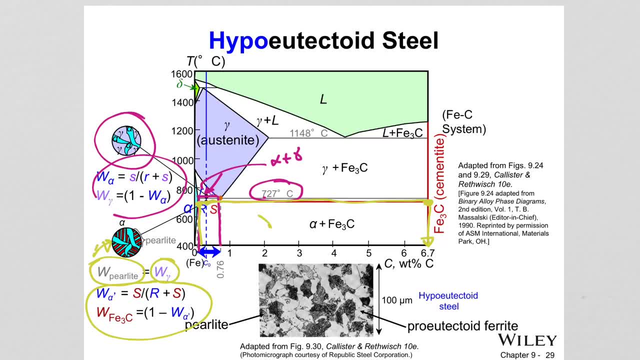 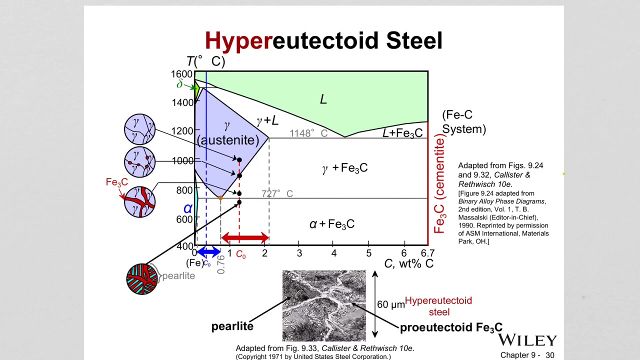 gamma, because from gamma you form the pearlite, right. so, but if you want to find the weight fractions of gamma, you have to find the weight fractions of gamma and you have to find the weight fractions of gamma. so it's one of these. you have to find the weight fraction of gamma, and it's general. 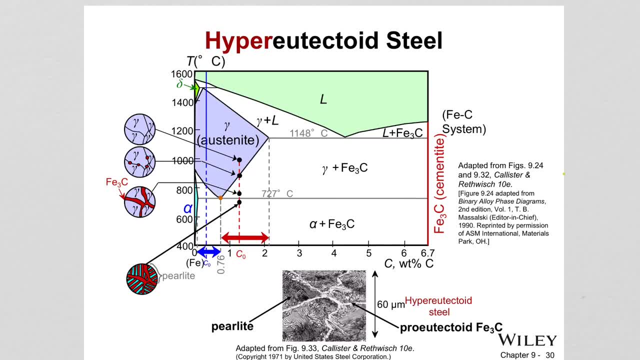 saving all this stuff and you so, if we want to use two temperature code numbers rests on our perspective of alpha之前, about up until uh. this range right. so within this range means above. above. we take to it composition. you can choose a composition and analyze the microstructure. so we start with. 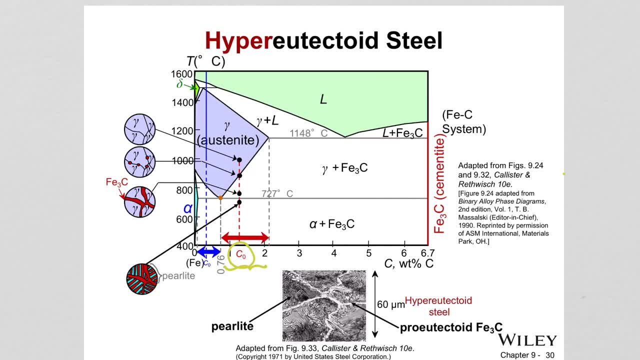 gamma, austenite, and from that um, a cementite is forming. as you can see, as you go down, uh, cementite is forming. now i have alpha and cementite in equilibrium. then if you go below, if you are just above the you take, you take to it. then you have again our gamma and cementite. 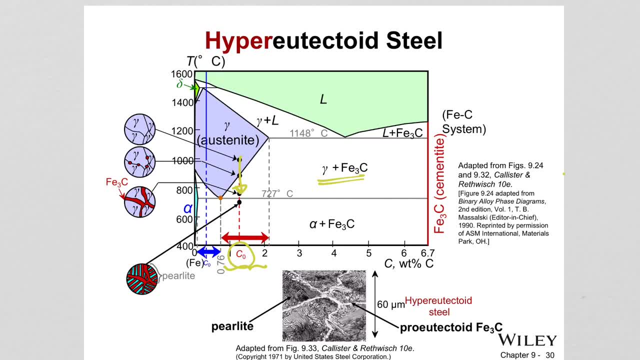 as you can see in the structure, and if you go below the you take to it temperature. now, from that gamma austenite it forms alpha and cementite structure. as you can see here, this cementite stays, this gamma forming the pearlite structure which has alpha plus cementite. 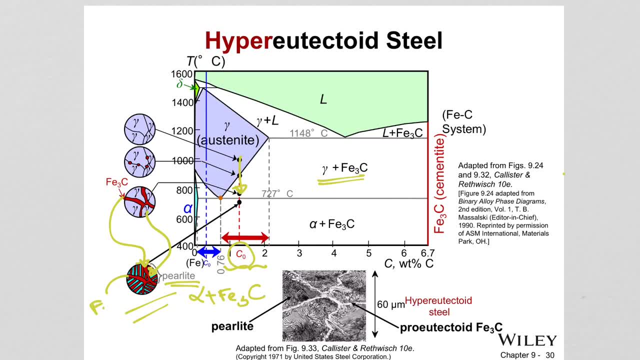 and it's how it is look like. see, these are cementites under microscope. and then you see the lamellar layer by layer structure. we call pearlite. okay, so again, the weight fractions are the same way. if we are above the, you take to it temperature right there. then you can read the. 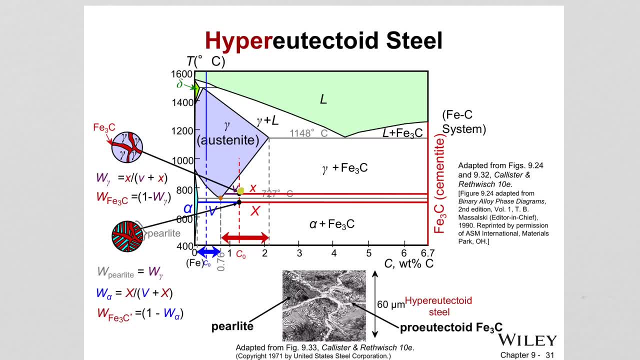 uh uh, amount of cementite and then the composition of the cementite from this intersection and composition of the gamma from this intersection. so by using the same level rule you can calculate the weight fractions of the gamma and the cementite at that point. and remember, from cementite, cementite stays the same from gamma. 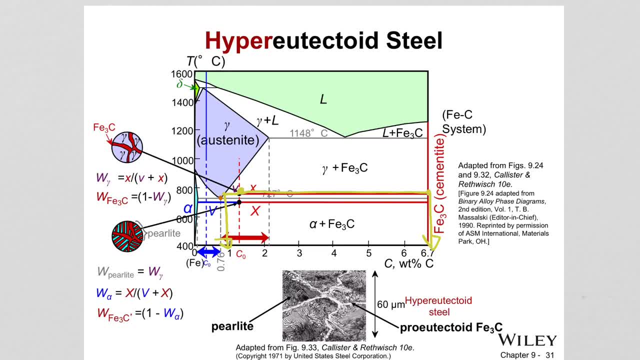 uh, pearlite forms. so the weight fraction of the pearlite is therefore equal to weight fraction of gamma, because, uh, the same right from gamma, the pearlite is forming. and uh, if you want to know the composition of alpha and cementite inside the pearlite, uh, inside the pearlite, and then you can. 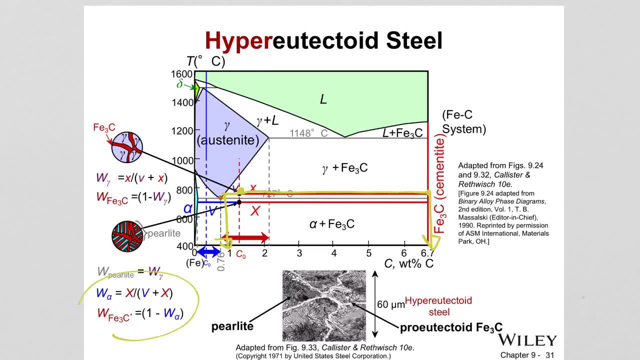 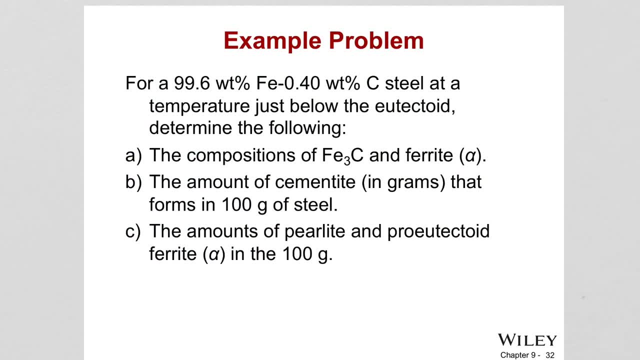 useそうですね, but we only~~~~~~~~~. ok, very Caustic, ok, but when you just say platinum without the so and uh nitric acid, again. let's look at an example. if the Uttek to it tmp temperature 0.4% carbon steel, carbon steel, 태 big as much as a temperature just below the utனk lt temperature low than 0.8% to it, Yeah, and begin to tap dil servants. again, we need to use the lever rule again. okay, let's look at an example. for a 99.6%32 iron mass rubdown, stamina, iron and point four, % carbon steel, carbon steel, carbon steel at temperature just below the. you take two it m Demperature. again, we need to use the in addition to pskFFTiez millions. I'm going to give you a little gothyJand if you want to read the sample. if not, take any ayuda if you want to read them, all these diagrams. 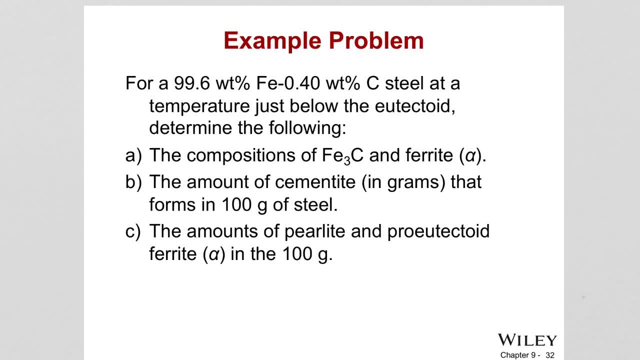 determine the following. So we are looking at the carbon-iron-carbon phase diagram and looking at the carbon composition of 0.4 weight percent. So a the compositions of cementite and ferrite be the amount of cementite that forms in a hundred grams of steel and amounts of 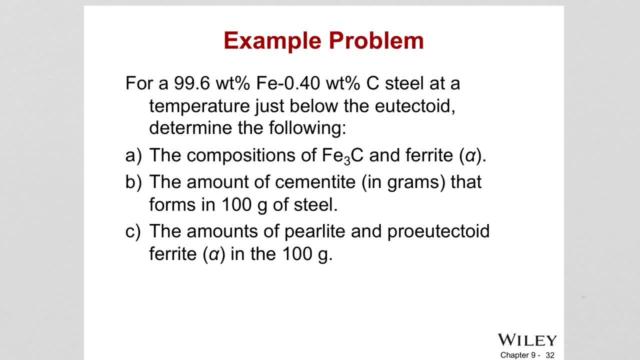 pearlite and JK2 ferrite in a hundred grams. Okay, so you need to understand that we have. we have a steel and which is alloy of iron and carbon. Cr поставure on ironform is 100 grammes. feature of down-to-earth. 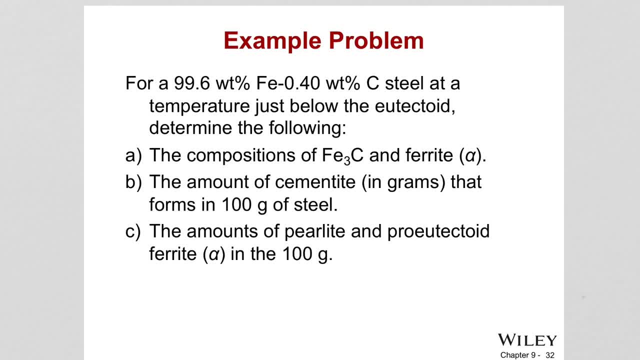 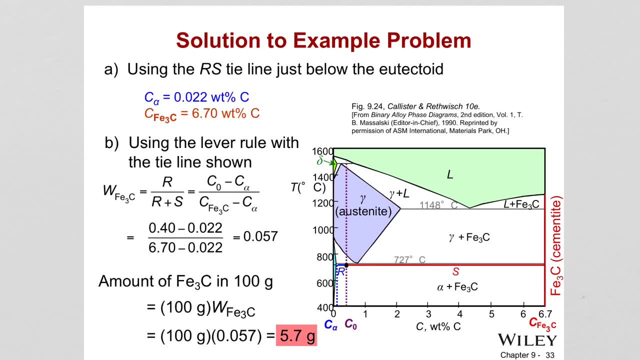 performance of iron is mountainous. so the weight fraction, l'echo force, a recipes ignorante of this hour. macroniner gas concentration to the number oflilà Ladurée Jı lolä. composition of this steel is 0.4 percent. So if we look at the iron carbon phase diagram, 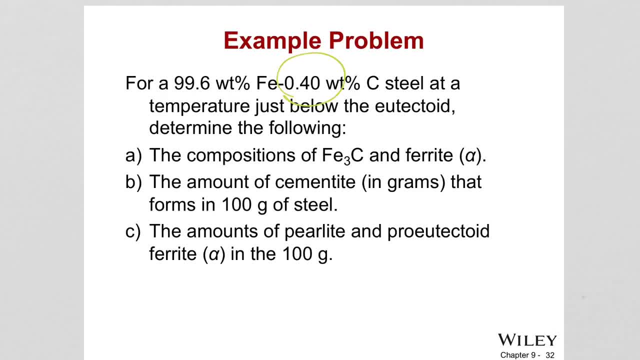 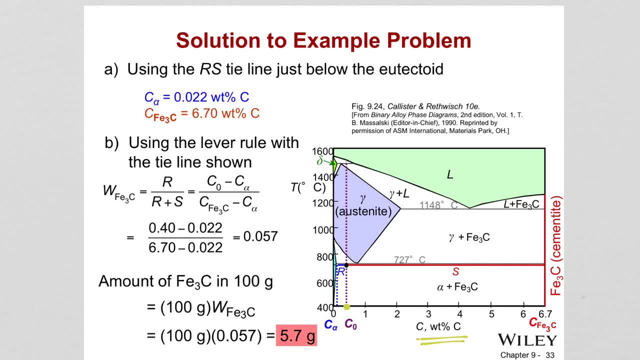 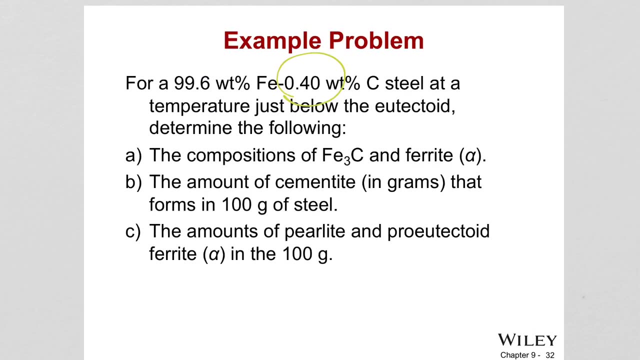 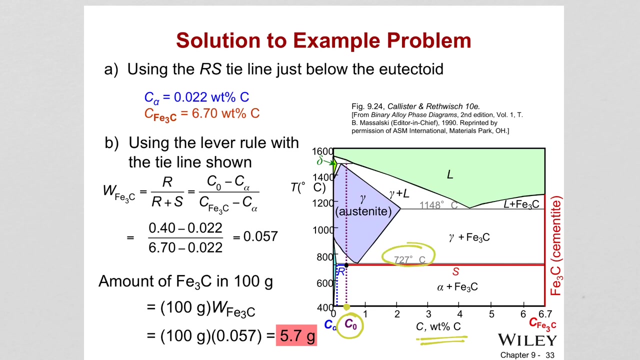 first locate your composition right. this is the composition in the x-axis we are given carbon. locate 0.4. okay, it's somewhere here and this is our original composition and we are told that at a temperature just below the eutectoid temperature. So just below this is the eutectoid temperature, right? 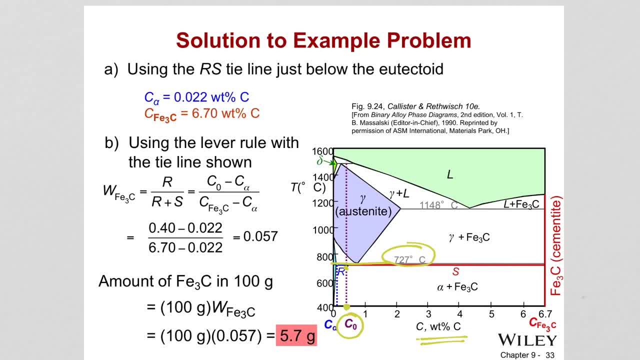 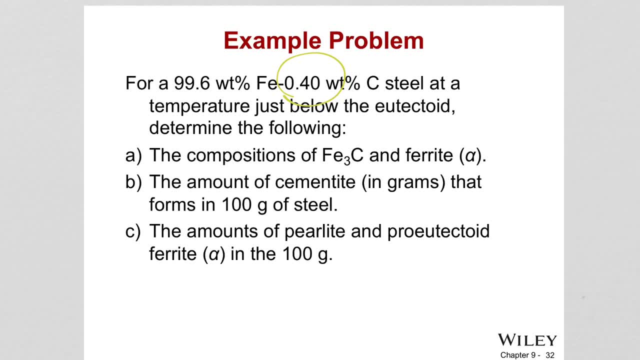 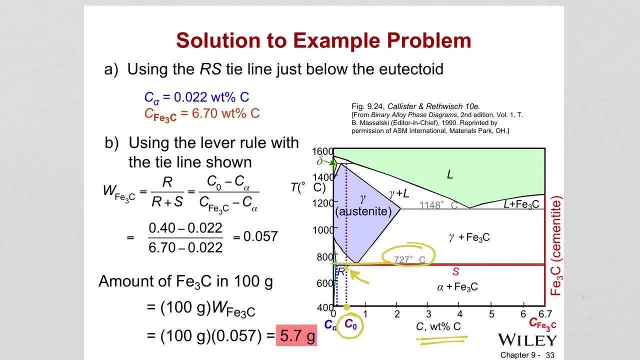 somewhere below that eutectoid temperature. we have to read the composition of what does it ask? let me see the composition of cementite and ferrite. Okay, it's easy because at this just below the eutectoid temperature, sorry, it's very late. 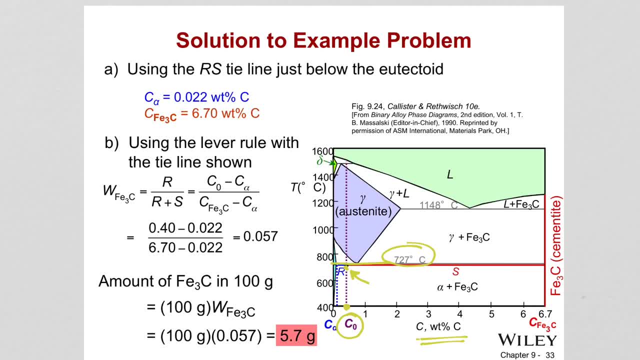 my mind is not able to concentrate. Okay, so we are talking about just below the eutectoid temperature and we are seeing, we want to find the composition of alpha and cementite right. So, like the tie line, we draw the tie line like this and go to the intersections like this and read the 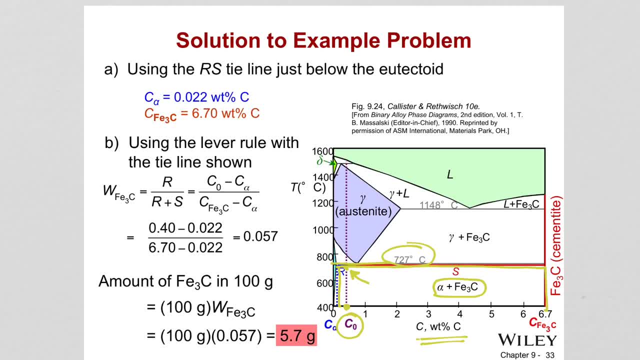 compositions there. Of course, if it's not very clear from the diagram, reading some approximate value is okay, but we read 6.7 percent for the cementite and we read approximately 0.0228 percent of carbon for the alpha. Okay, So these are the ones that are inside the pearlite. 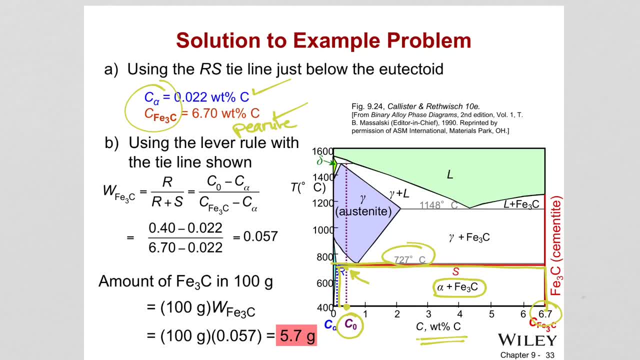 Okay, Now, using the lever rule with the tie line shown, calculate the weight fractions. Okay, this is easy because we know from the equation the weight fraction of cementite and weight fraction of- oh it's, let me see what's asked- the amount of cementite that forms. okay, 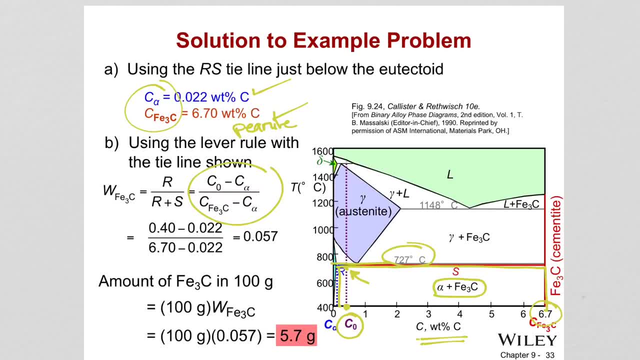 So see, you have 100 gram of that material. how much of it is cementite? now we are talking about the weight fraction. so if you find the weight fraction of the cementite using this phase diagram, as we have learned, which is 0.057.. 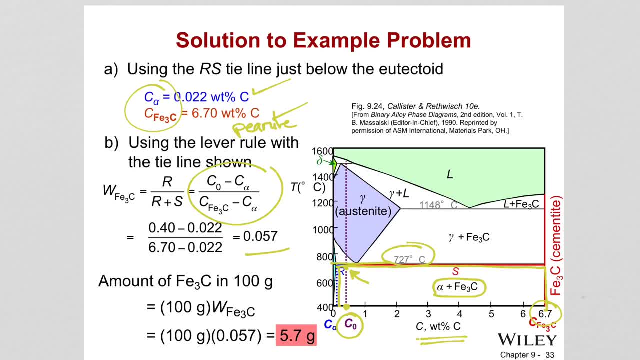 that means 5.7 percent. okay, what is the 5.7 percent of 100 gram? and that should be 5.7 gram. so 5.7 gram of the 100 gram is actually cementite. so next, let's see what does it ask. we figured this out, this out. 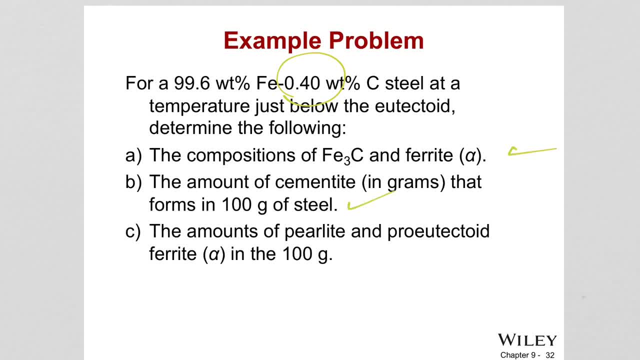 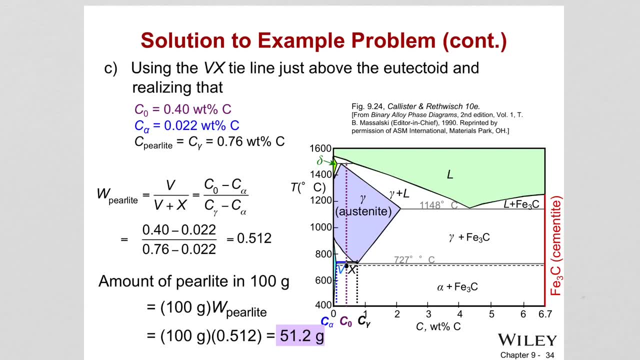 the amounts of perlite and protectoid ferrite in 100 gram. okay, so now you gotta remember, here we had gamma and alpha and from that, when we cool it down below, take to it this gamma went formed cementite and alpha ferrite. but also alpha remain in the structure. if you remember, we have alpha here, here like. 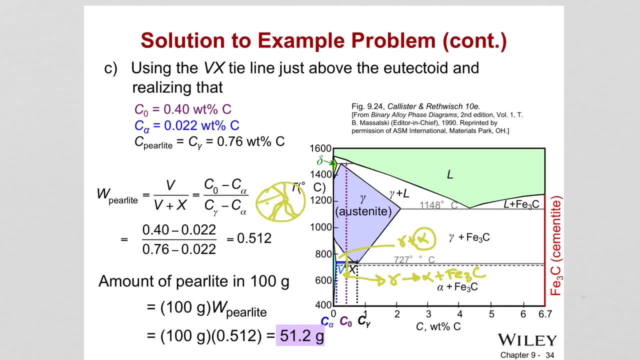 this and then and lamellar structure which is formed from gamma. so this formed from gamma to ferrite structure and cement, cementite and ferrite, and this was the alpha. okay, so we know what C naught is, which was 0.4, and we know C. 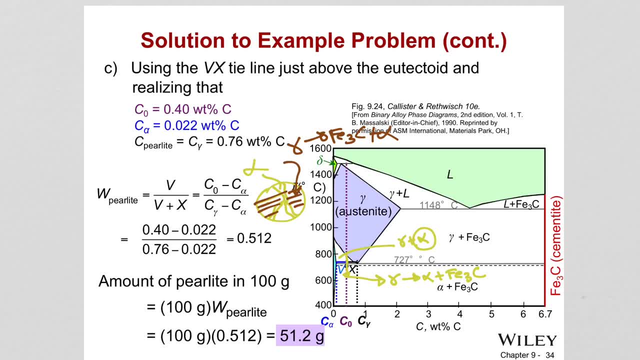 alpha, the composition of the alpha, remember this is just above the eutectoid temperature. so we are talking about this as a tie line here. so I read the compositions from there. I know C, that I read C, alpha and C, gamma is read from there, because there you have only alpha and gamma. and remember the pearl. 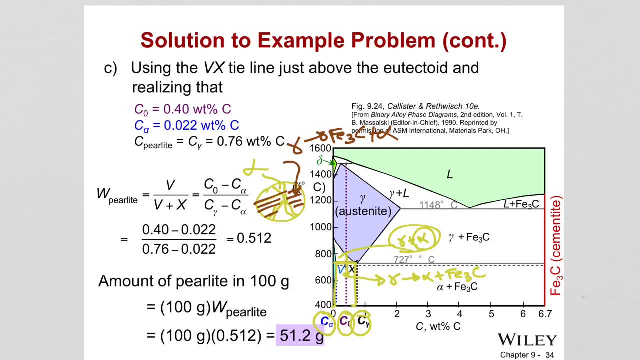 light composition was equal to the composition of the gamma, which is- which is your read from here, right this one- 0.76.. So we got to find the weight fraction of perlite just above the eutectoid. and again the same way we calculated from: 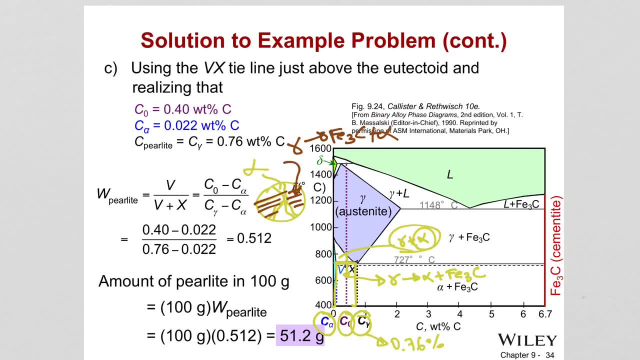 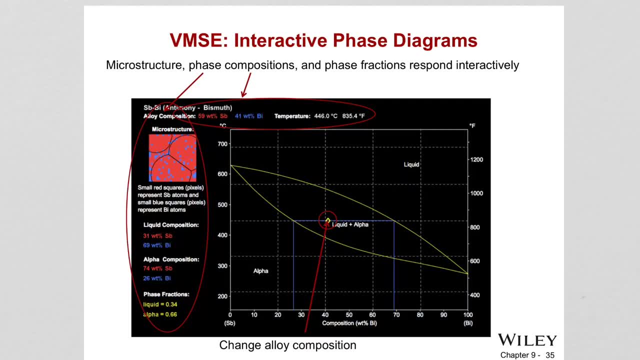 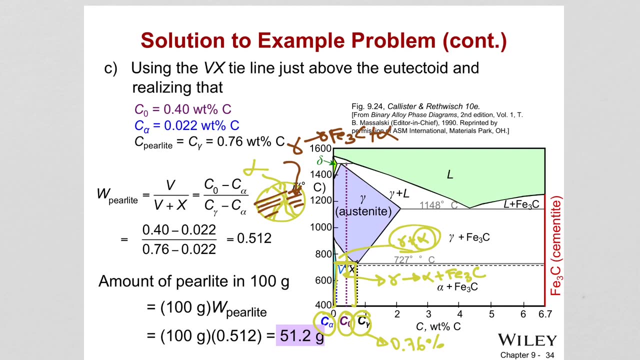 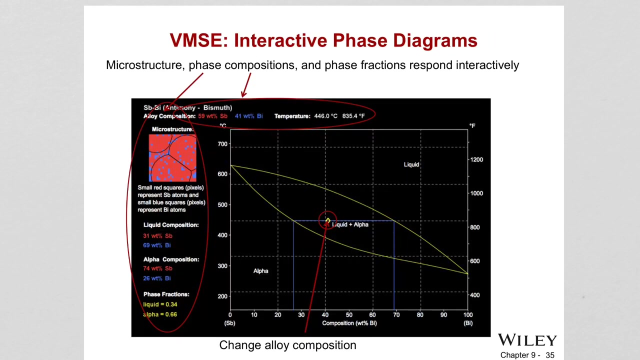 the level rule that means we have 51.2 gram. of that, 100 gram is perlite, Of course. the remaining should be the alpha, right? So hundred minus 51.2 should be giving you the weight fraction of the alpha. So again you can look at the virtual material science in engineering and 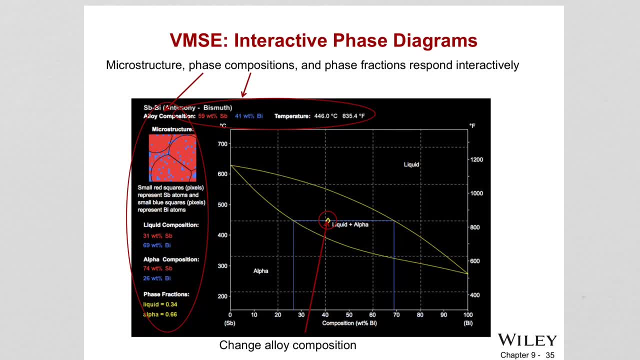 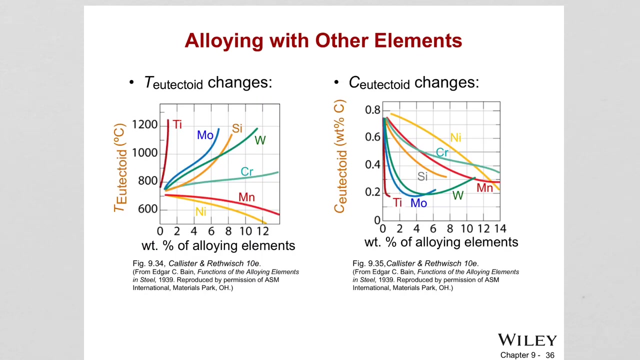 there are interactive phase diagrams. you can check the microstructure how it looks like. for different kind of phase diagrams you can just google VMSE or I already sent you guys several links to that website. so sometimes this iron carbon system steel is added. other alloying elements are added to the 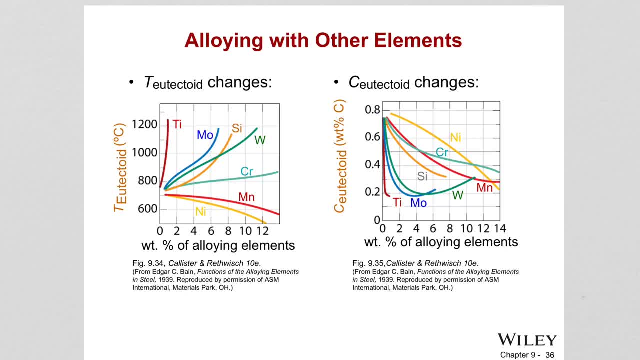 structure and there are reasons for that. if you want to control, do you take to a temperature? we take to its composition and induce some changes to that phase diagram and And people may want that because controlling the working temperatures are important, So they add actually other alloying elements. 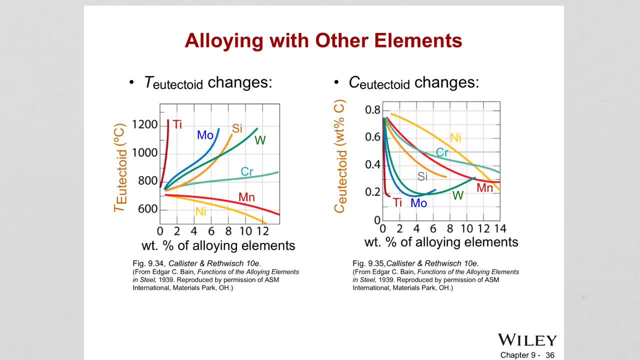 So that is one of the reasons why people add alloying elements to the iron-carbon alloying system And you can see how eutectoid temperature changes with addition of alloying elements and how different alloying elements changes the eutectoid temperature differently. 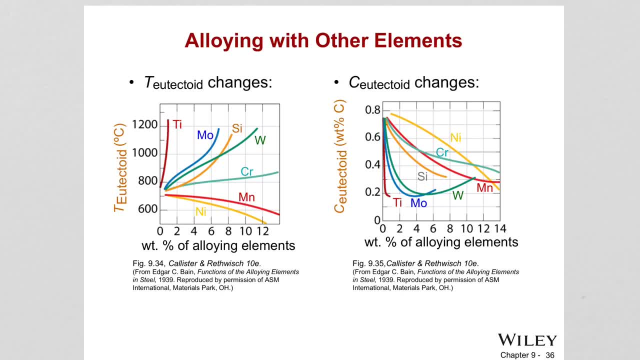 As you can see, adding nickel, as a function of nickel element, the eutectoid temperature is decreasing. Manganese is the same, But some elements like titanium, molybdenum, silicon- they are increasing the eutectoid temperature. 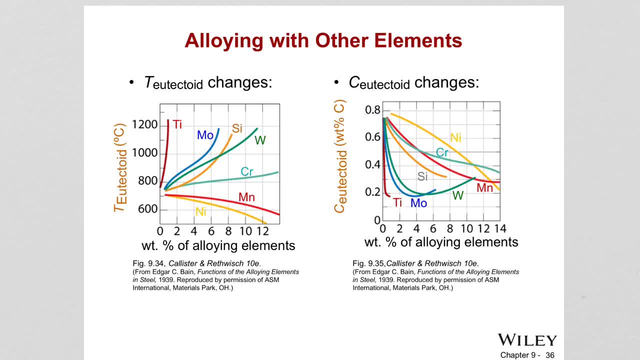 And we see the how elements addition of other alloying elements also affects the eutectoid composition. They are also changing the eutectoid composition on the carbon-iron phase diagram, So their effect can be seen in here right. 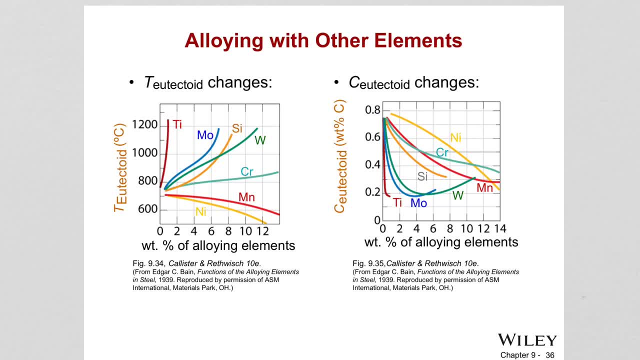 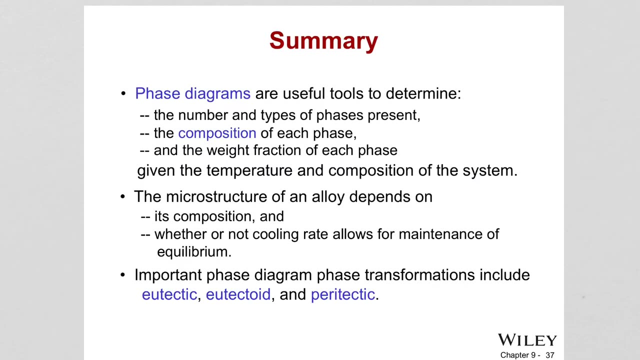 So with titanium, all elements seems like they are decreasing the eutectoid composition, But with titanium they are increasing the eutectoid composition on the carbon-iron phase diagram. So, in summary, we learned about phase diagrams. These are important tools because we might want to know what phases present in the structure. 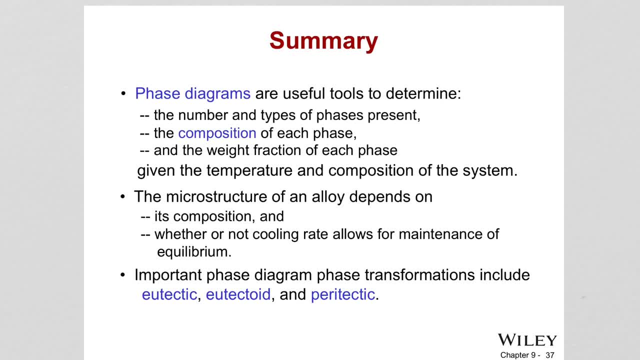 depending on what is the composition, temperature. And we learned that we can actually get information like what is the weight fraction of each phase or what is the composition of each phase, depending on the temperature and composition. And we have learned that microstructure of an alloy depends on its composition.